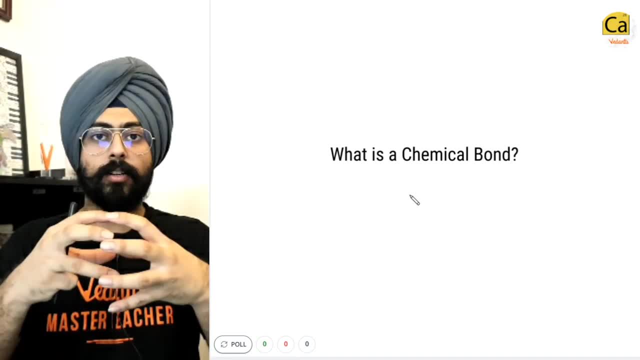 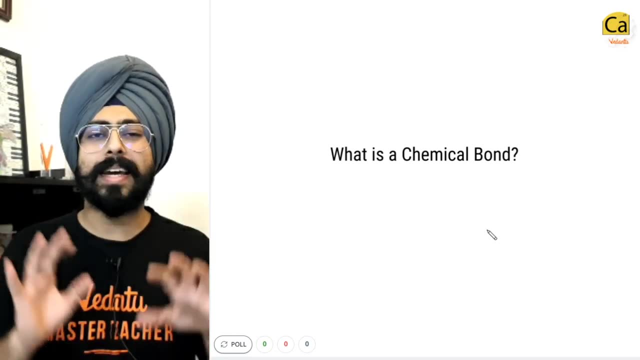 is just the forces of attraction that keep atoms together so that they are stable as an entity, as a molecule. yes, So there are multiple theories on why these forces exist, but basically these are electrostatic forces. Now, how they achieve stability? There are different, different. 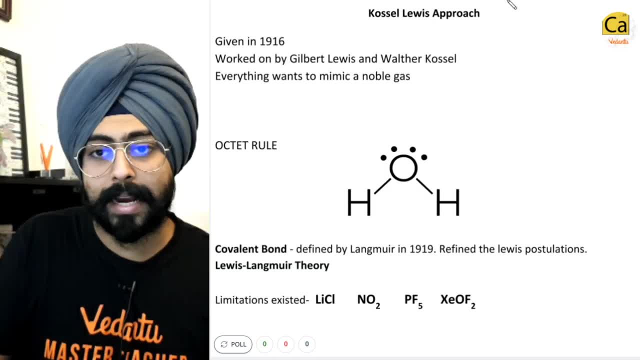 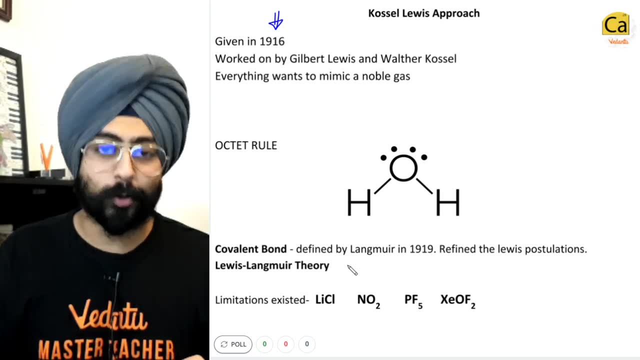 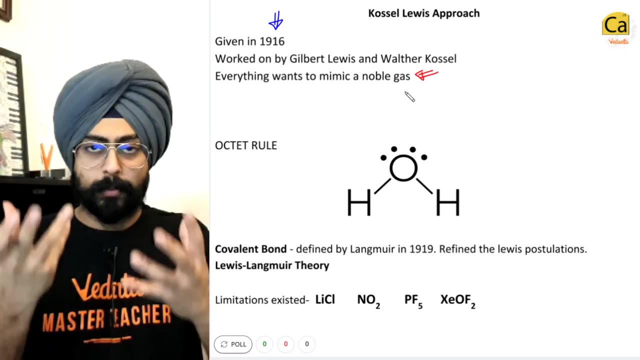 different theories to that. So the very first theory was given back in 1916, alright, and it was worked on by these two people, Gilbert Lewis and Walter Kossel. Everything wants to mimic a noble gas. This was the idea. Why? so, Because these people realized that noble gases like helium, neon, 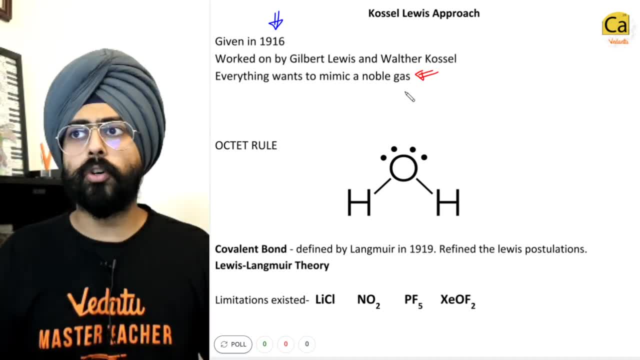 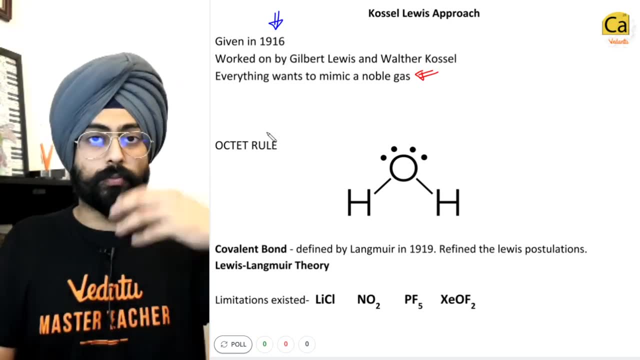 argon, they don't really want to react with anything else. So since they are already stable, everything else wants to become stable like a noble gas. Hence came their idea of the octet, and the theory was revised and, you know, made better, better by this guy called. 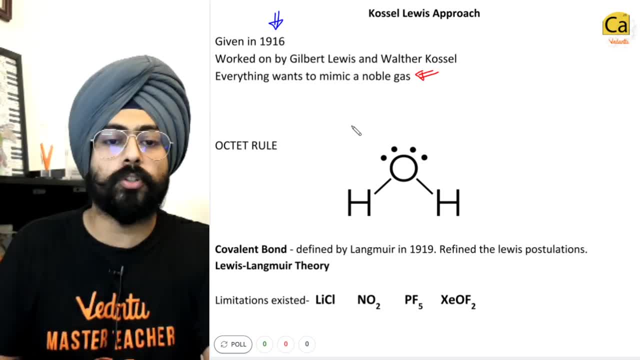 Langmar in 1919, and he just redefined the Lewis postulations, and hence came the octet rule, that you need to have eight electrons in the outermost shell of an atom for it to be stable. So what we have over here is a Lewis dot structure of water. yes, So over. 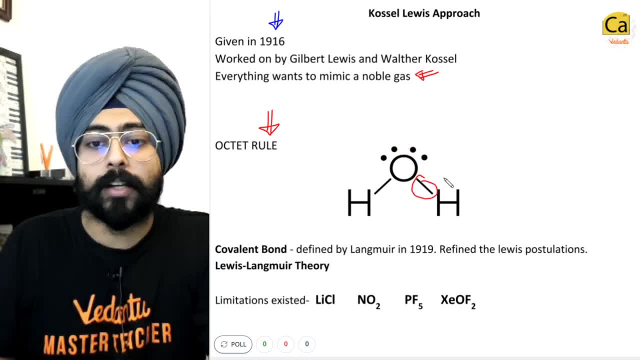 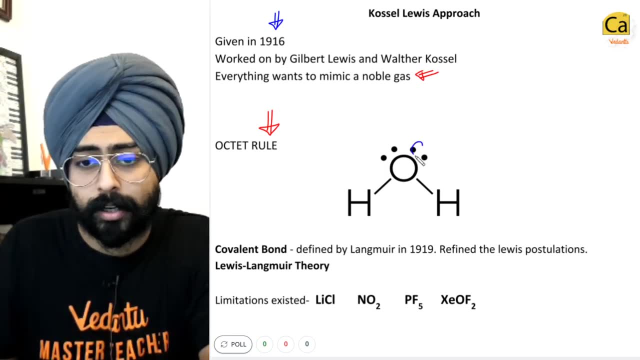 here you have two lone pairs and you have two bond pairs. Always remember that a bond pair has two electrons. Yes, if you notice carefully, oxygen's octet is complete: 1, 2,, 3,, 4,, 5,, 6,, 7, 8 electrons. 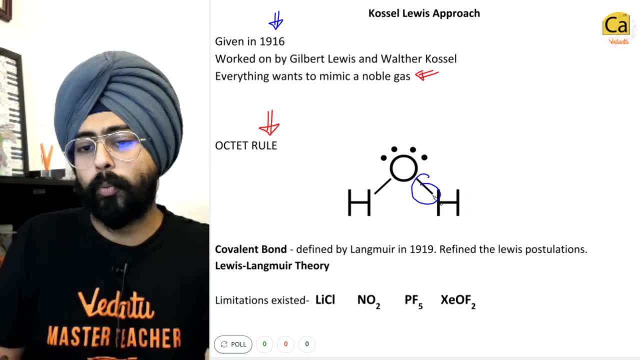 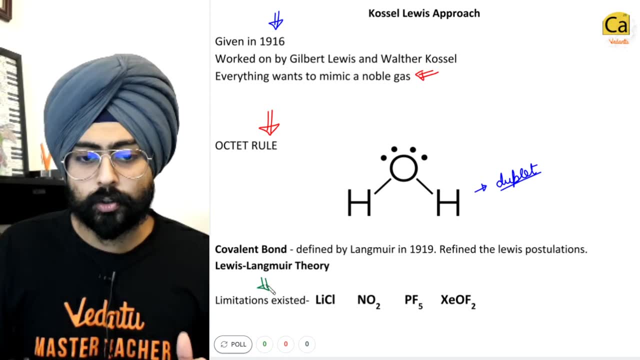 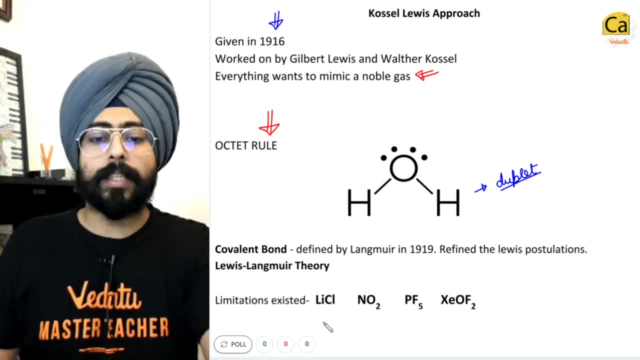 But if we look at hydrogen, hydrogen me only the duplet is complete. yes, In hydrogen only a duplet is complete. So let's quickly come to the limitations of this octet theory: LICL, even in LICL, lithium has a duplet, not an octet. So there were compounds in nature which 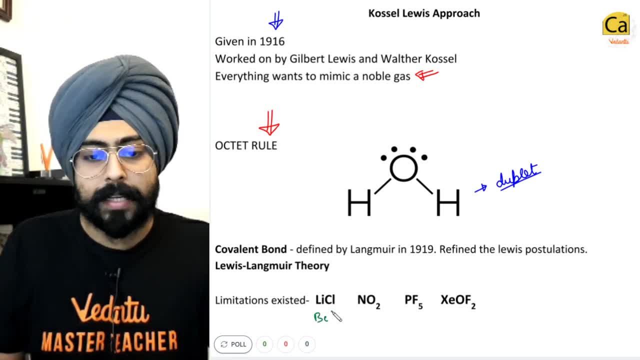 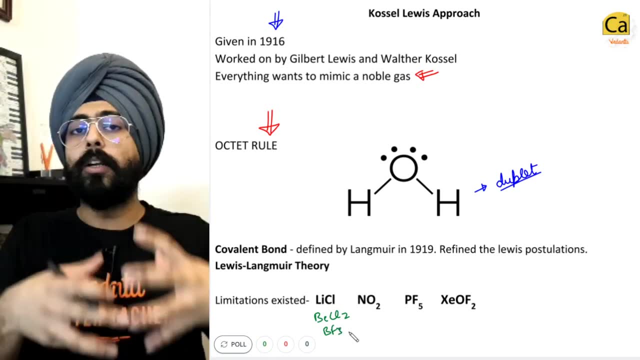 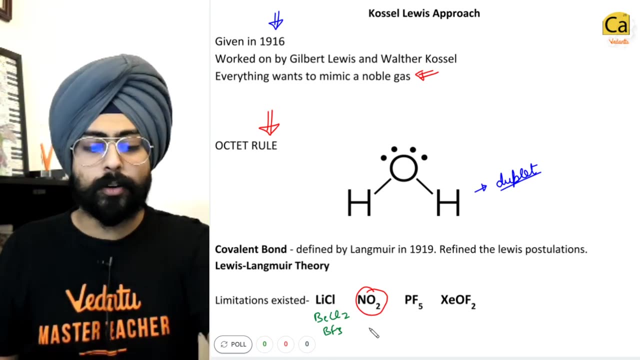 had incomplete octets. For example could be BECL2, BF3, so on and so forth. So there are lots of compounds in this nature which have an incomplete octet. That was one limitation. Then comes compounds like NO2.. What about NO2?? NO2 is an odd electron species. Do you realize This is an odd electron. 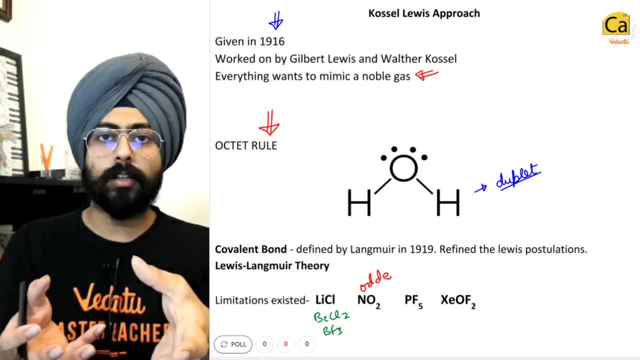 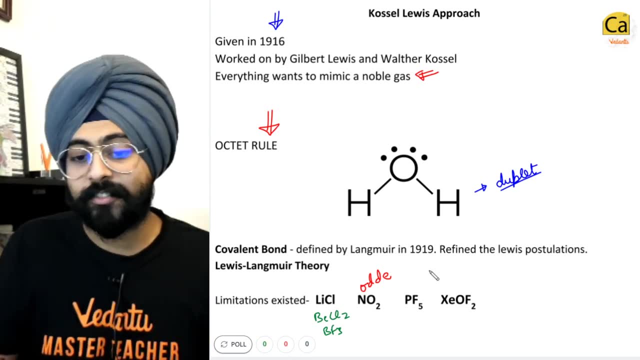 species. So if you have odd electrons, obviously you cannot focus on making the octet, isn't it? Odd electrons, how can you make an octet? Then you have PF5.. In PF5, for phosphorous, what's going on over here? This is the expanded octet. Yes, this is the expanded octet. You. 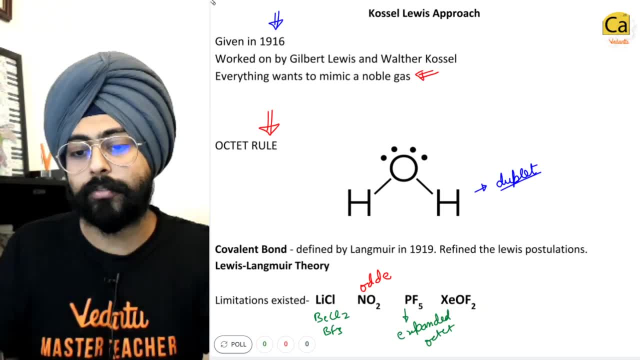 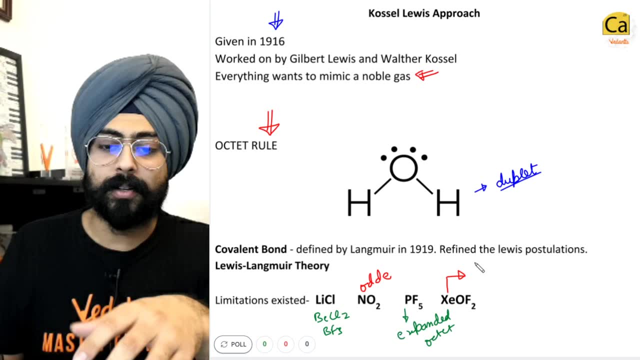 have 10 electrons in its valence shell and finally you have XCOOF2.. This theory was based on the idea that the noble gas is stable, But Xenon being a noble gas- even Krypton- these guys react with a lot of Halogens and 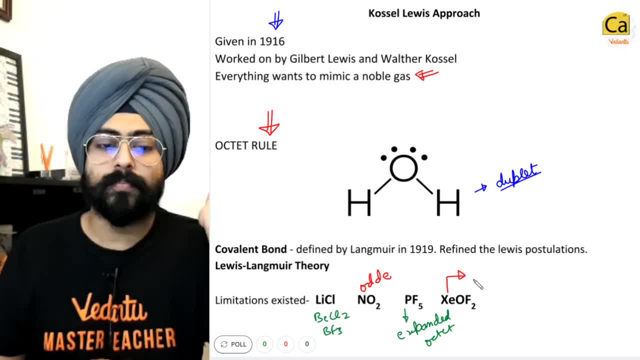 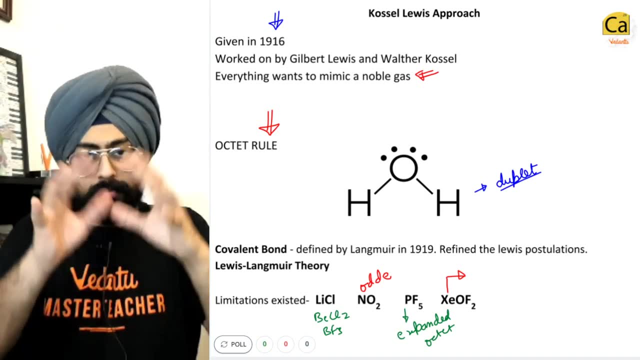 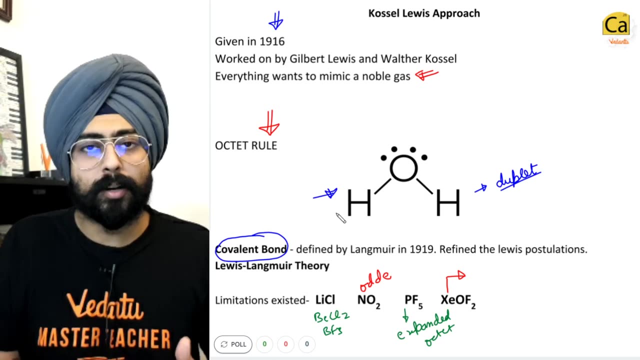 Chalcogens. the basis of this theory was not very good, fine, So this was the coastal Lewis approach. then, now that we have understood the basic octet rule and the limitations of it, we also know that water has two covalent bonds, and covalent bond essentially means sharing of. 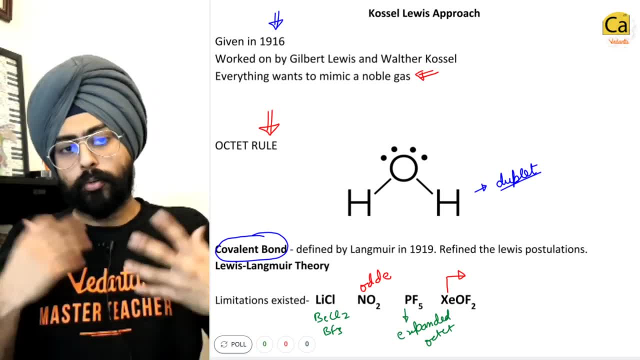 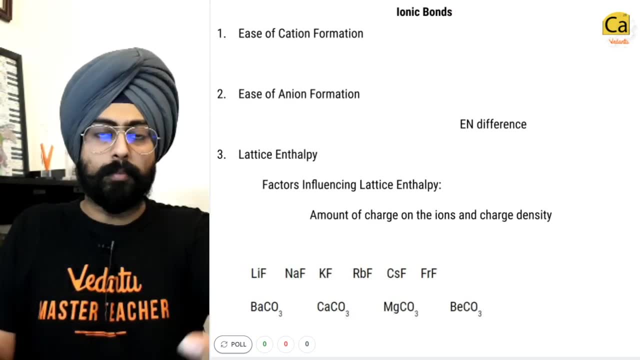 electrons defined by Langmar in 1919.. So now we should move on and talk a little bit about the other type of bonds that we have, and those are ionic bonds. Now, in order to form an ionic bond, in order to form an ionic solid, there are a few things that you 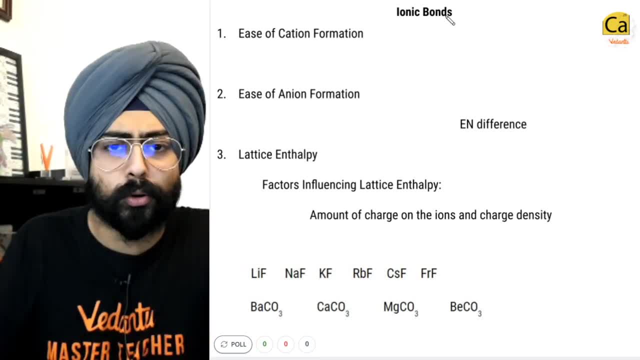 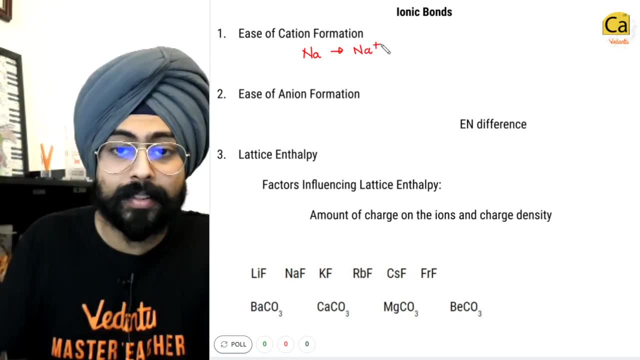 should keep in mind, and this is known as the Born-Habers process. I am sure you all remember that first ease of cation formation. So if you are forming a cation, for example this, then the process should be very easy. So, for example, the ionization energy of this. 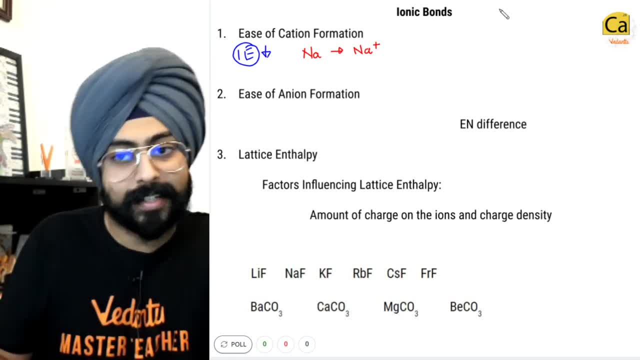 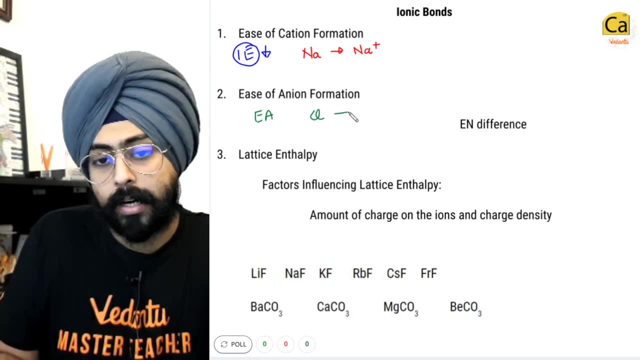 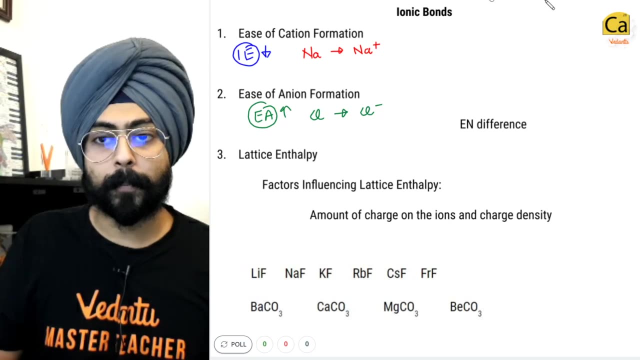 particular process should be low in magnitude. yes, then similarly, ease of anion formation, electron affinity or electron gain, enthalpy: Let's say we are turning chlorine into chlorine negative. this value, this magnitude, should be high. the anion should want to form. Then, talking about the electro negativity, 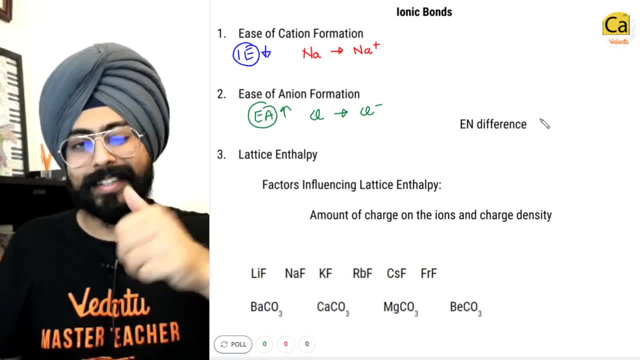 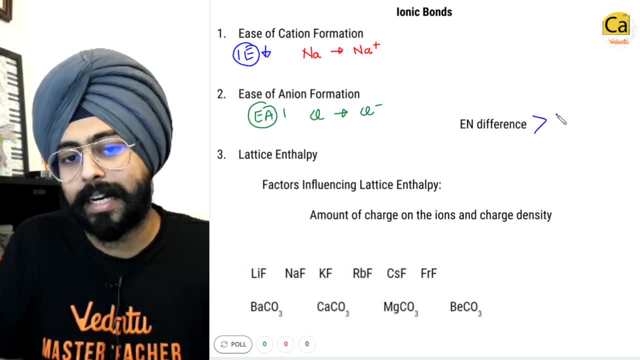 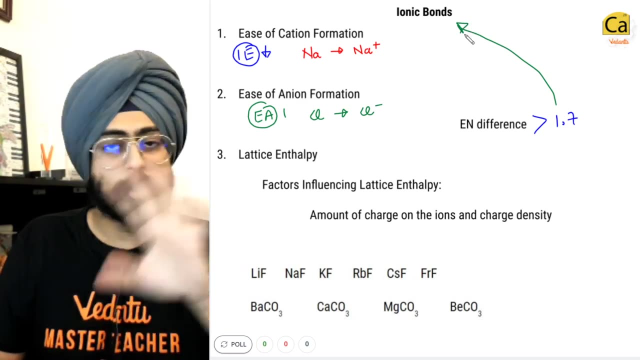 difference- something that we told in periodic properties chapter as well- that as a general thumb rule overall, if electro negativity difference, if electro negativity difference is greater than 1.7, then most likely the bond is going to be ionic. It's not a union. 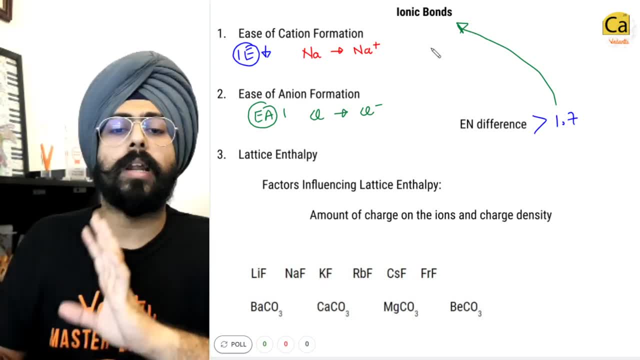 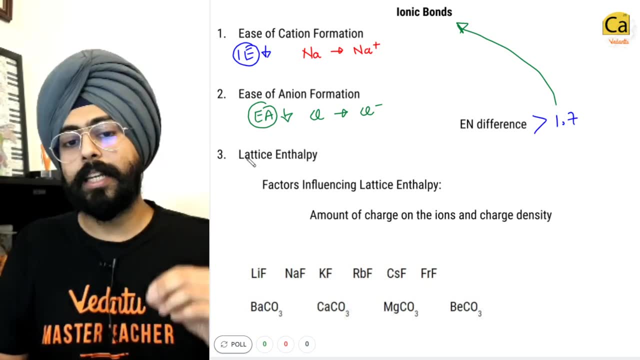 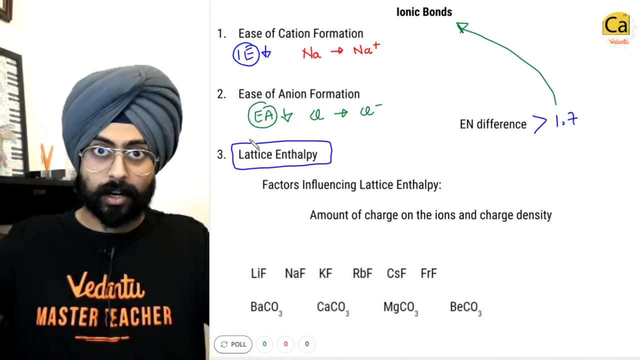 a universal rule. it is a general thumb rule that is applied to 90% of the cases. Fine, so less electron affinity, more ionization energy and then, finally, you should have lots of lattice enthalpy. What is lattice enthalpy? The energy released when one mole of ions come together and form one mole. 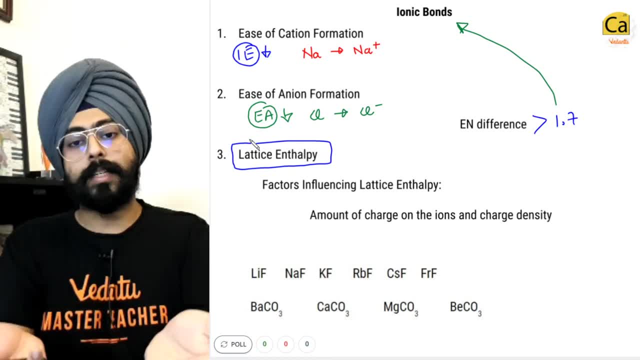 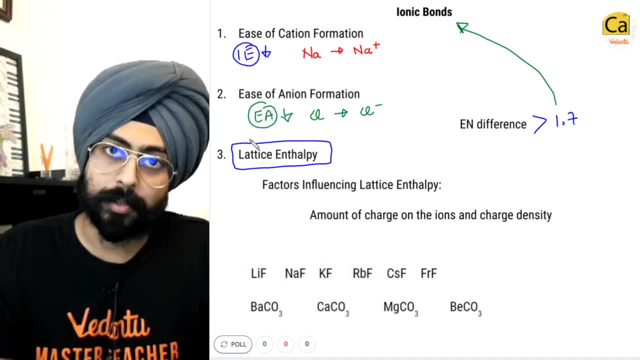 of a lattice. Yes, so one mole Na positive, one mole Cl negative, you form one mole of the lattice and the energy released during that process is known as the lattice enthalpy. Yes, so what are the factors that influence lattice enthalpy? Essentially, the amount of charge on the ions. 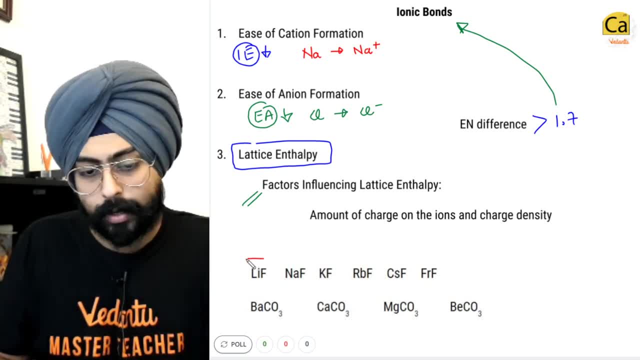 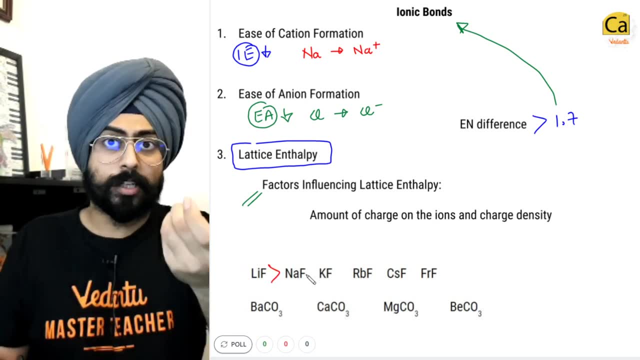 and the charge density on the ions. So, my dear friends, let's look at the first example. If I talk about the order of lattice enthalpy over here, lithium fluoride will have the highest lattice enthalpy because lithium has the most amount of charge density over here in all of. the cations and ions are the same all over here. Yes, so in this example, lithium fluoride will have the highest charge density, hence highest lattice enthalpy. Similarly, in the example that I've given on the bottom, you know what Beryllium? beryllium is the smallest, so that's. 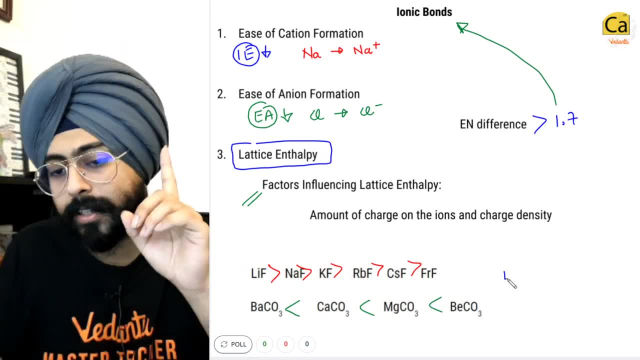 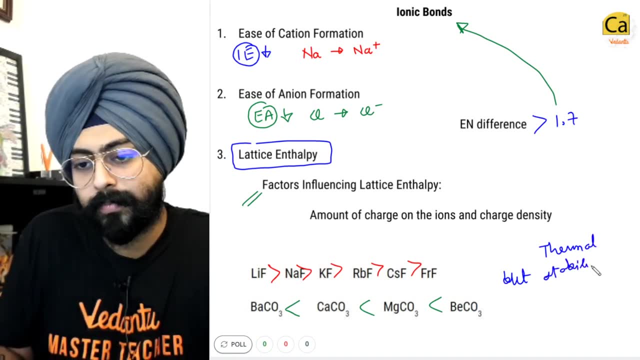 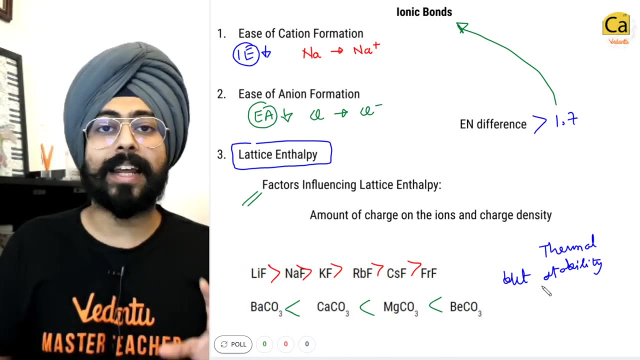 going to have the highest lattice enthalpy, but there is a catch over here. Have you heard about thermal stability? I'm sure you have. Yeah, now, when we talk about thermal stability, the order of thermal stability does not need to be the same as that of lattice enthalpy In thermal 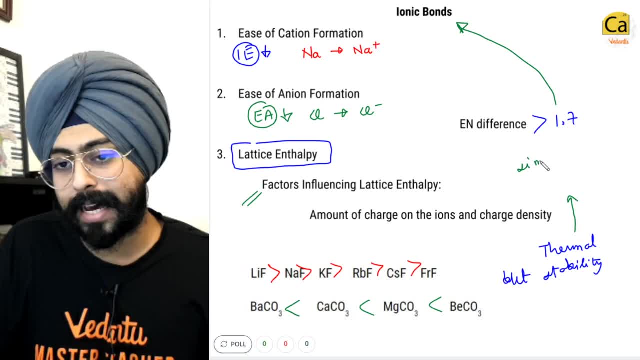 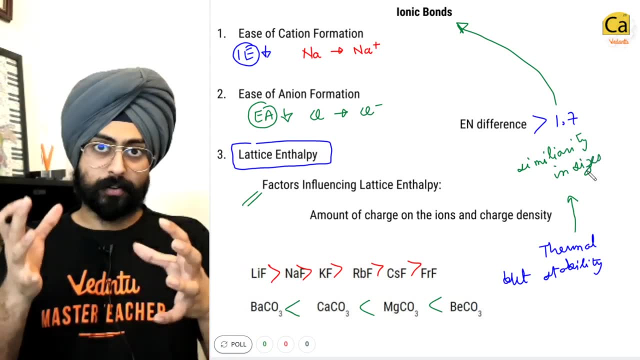 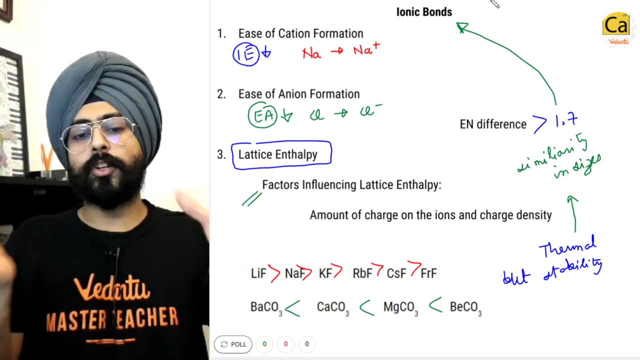 stability. we also need to talk about the similarity in sizes of ions. Okay, similarity in sizes. What this means is that, for thermal stability, small bonds better with small, large bonds better with large. Do you realize the difference between breaking a lattice? 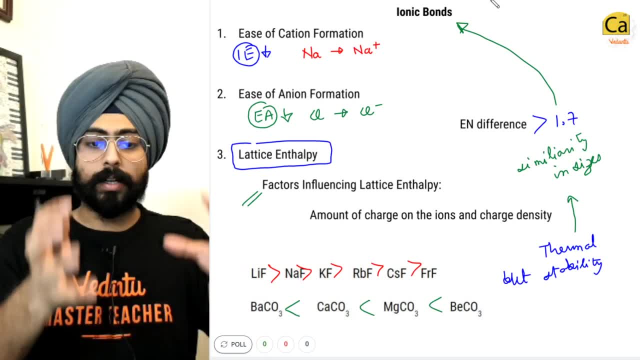 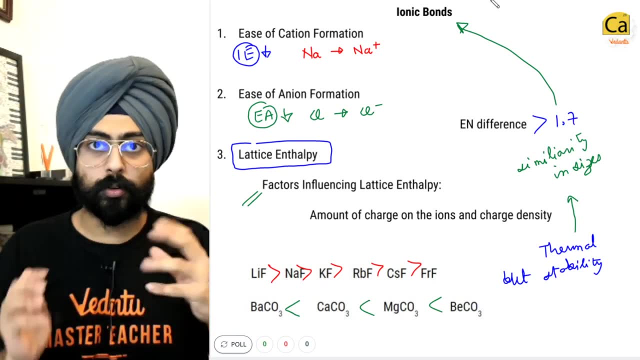 and thermal stability. When you are breaking a lattice, you are turning BaCO3 or LiF into Li positive, F negative, Ba positive, CO3 2, CO32 negative, Ba2 positive, CO32 negative. yeah, 3, 2 negative. but when we are talking about thermal stability, thermal decomposition could be any. 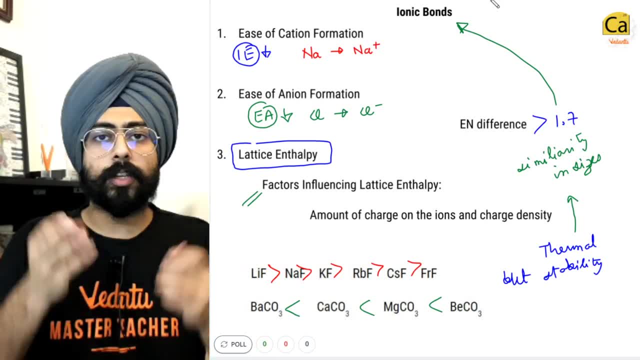 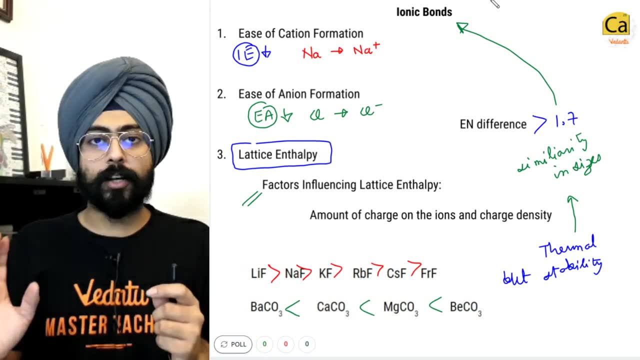 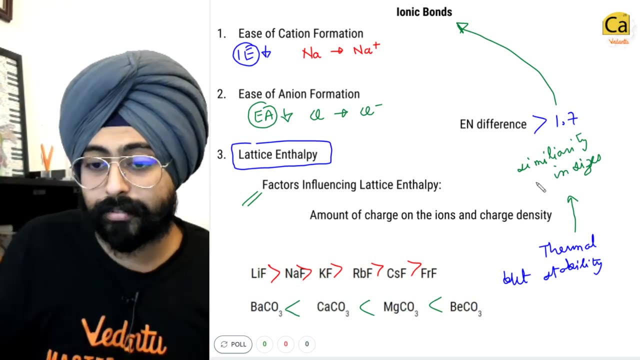 reaction. yes, thermal decomposition could be mg co3 plus heat gives you mgo plus co2. so essentially, thermal stability talks about the amount of heat you need to provide so that the compound just breaks apart into something else. hence thermal stability is different compared to lattice enthalpy. and if i talk about the order of thermal stability over here, it's going to be absolutely 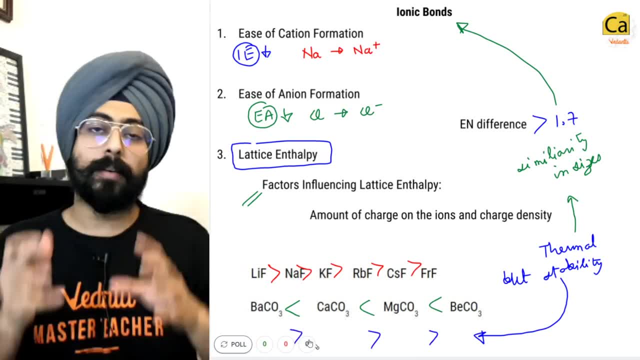 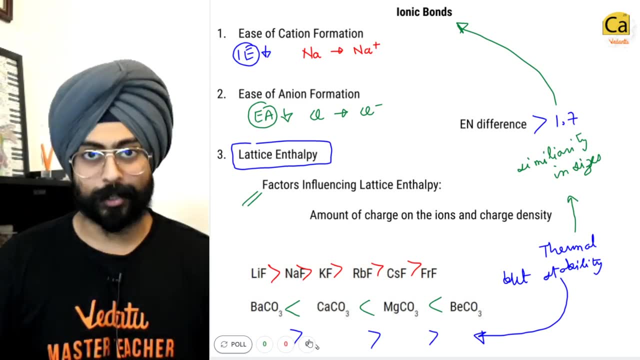 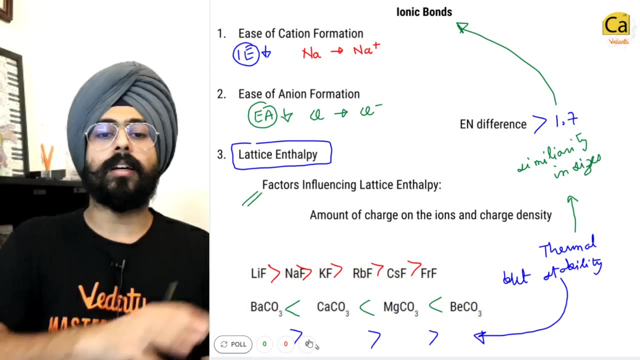 the opposite. okay, thermal stability may experimentally determined that the opposite order is to be a co3 is more stable to heat compared to be co3. all right, so whenever you are, whenever you are talking about thermal stability, think about similarity in sizes. otherwise, think about amount and density of charge. fine, very cool. now let's move on ionic. 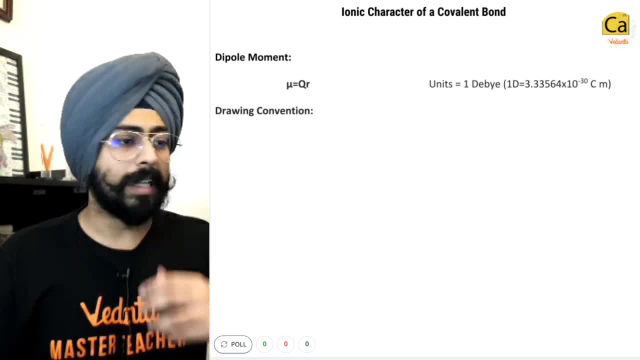 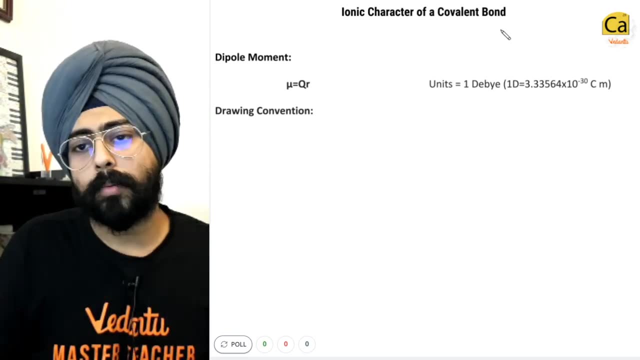 bond and covalent bond. these are our man-made assumptions, right in reality? okay, in reality, what exists is something in the middle, isn't it Fine? So let's talk about the ionic character of a covalent bond coming more towards reality, Instead of sticking to the ends of the spectrum. 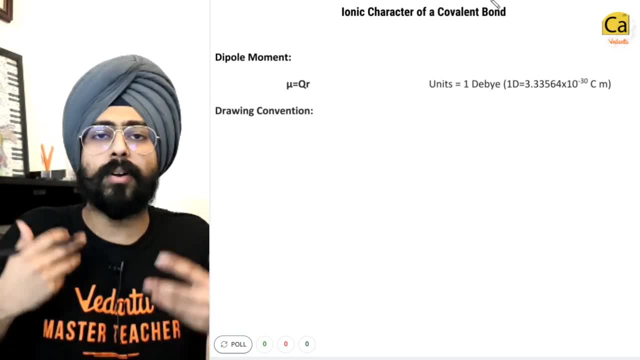 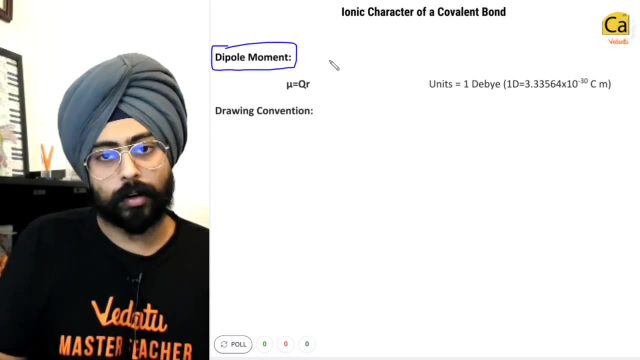 ionic and covalent bonds are just bonds. It's just our interpretation that they are ionic or covalent. Fine, So ionic character of a covalent bond is defined by dipole. moment, Alright. What is a dipole? Dipole is essentially a collection of two opposite charges. So let's say there is a 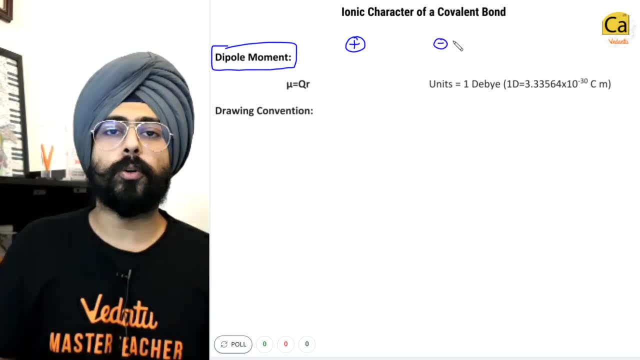 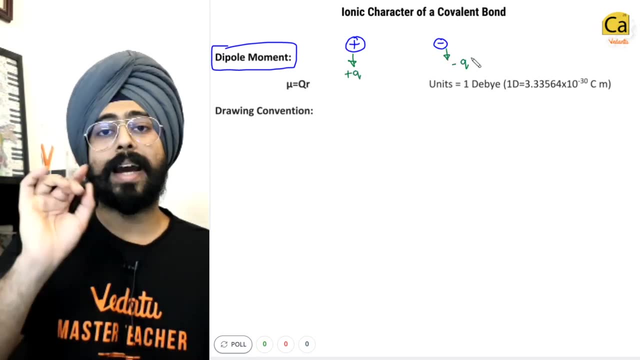 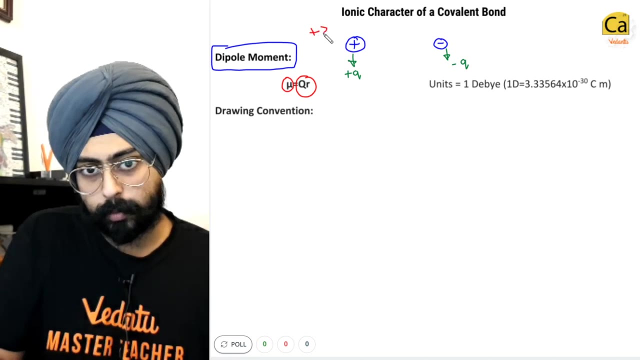 positive charge at some distance from a negative charge. This constitutes a dipole. If the charge on the positive side is plus Q and the charge on the minus side is minus Q, I can write the dipole moment, as mu is equals to Q times R. Okay, So if this charge was plus 2,, this charge was minus 2,. 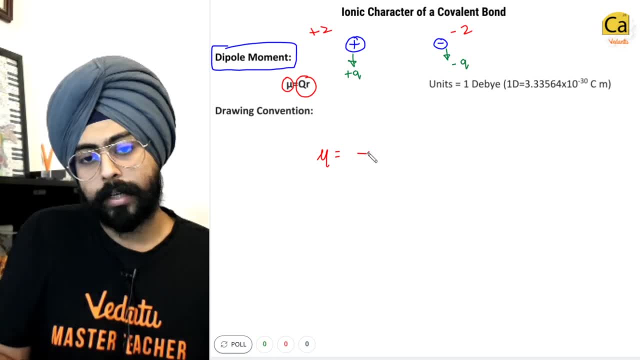 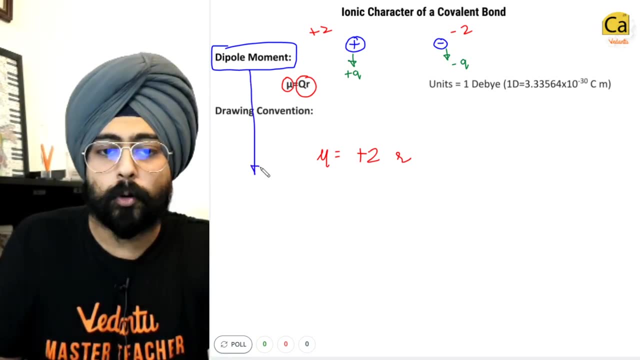 I could have simply written: mu is equal to 2 times R. Alright, And now dipole moment. as you all must remember, dipole moment is a vector quantity. Yes, dipole moment is a vector quantity In physics. the convention is: 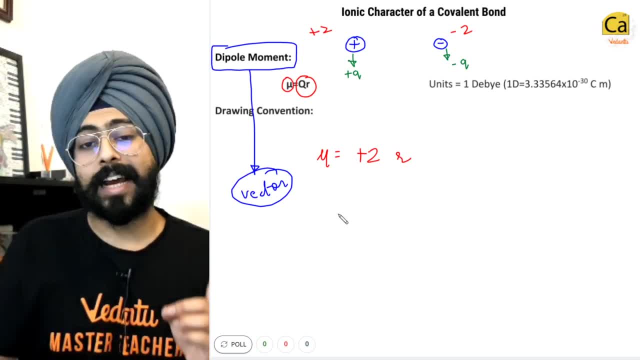 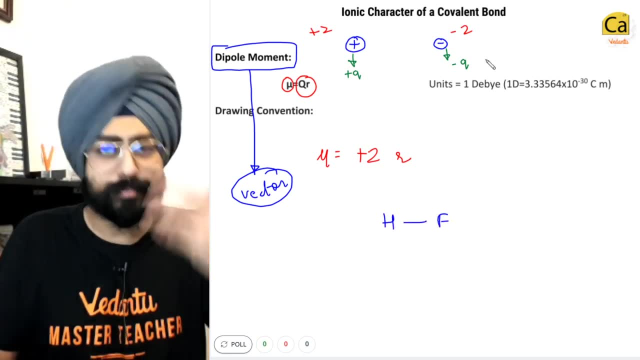 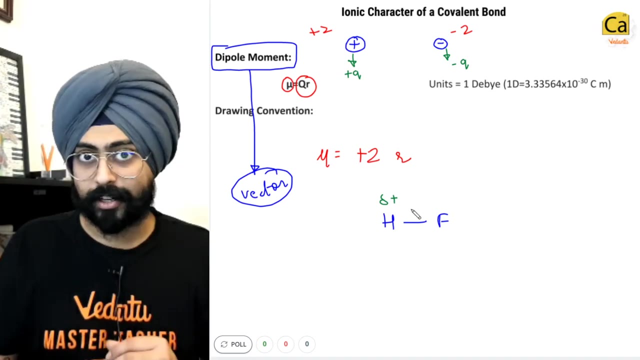 different In chemistry. alright, in chemistry the dipole always points from the positive side to the negative side. So once again, let's take the example of HF. You can also take the example of H2O. In HF, hydrogen will be partially positive in nature because of less electronegativity. 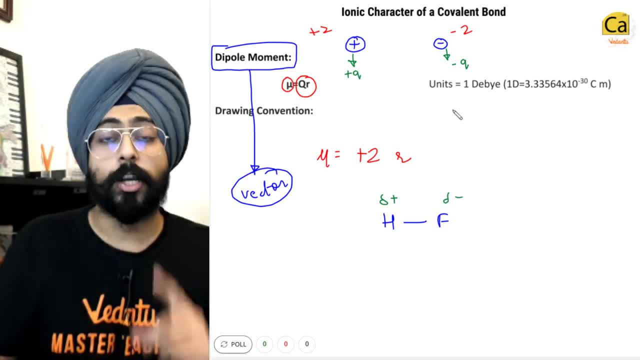 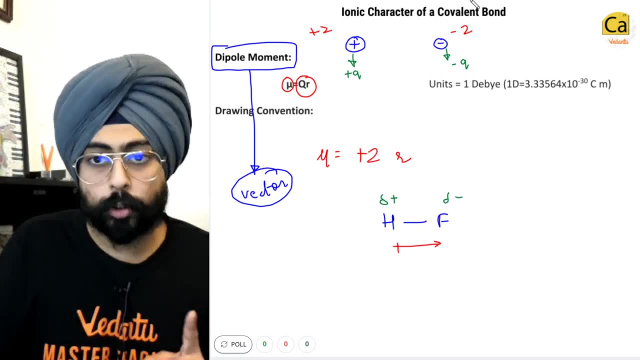 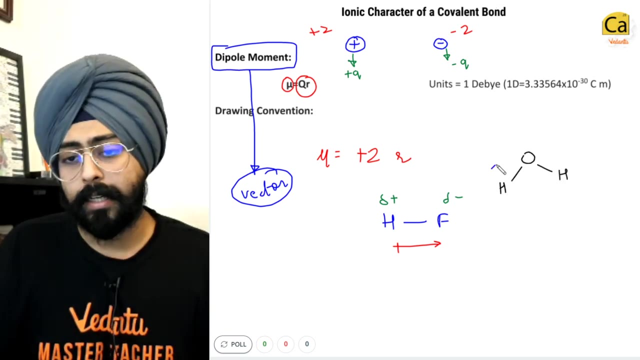 Fluorine will be partially negative because of more electronegativity. So for chemistry, the direction of the dipole direction of the dipole will be towards fluorine. It's entirely conventional. Also, since dipole is a vector quantity. if I talk about water molecules, you know that the individual dipoles 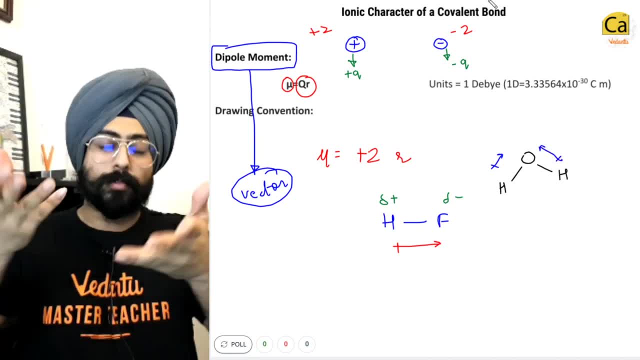 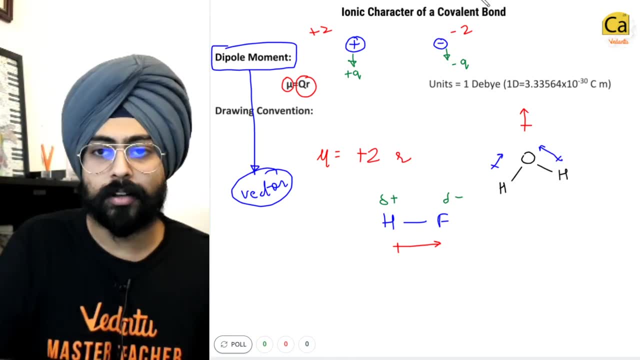 will point towards the oxygen molecule, So the oxygen atom. so overall dipole will be in the upwards direction. When you add these two up, that will be the direction of the overall dipole. Fine, So this is the drawing convention in chemistry. Also, if you want, to look at the SI units of dipole, the range is the darwin- Esteban baseline, for instance, the range of dipole pathway. So, � is the range of dipole in chemistry. So, if you want to look at the SI units of dipole, and then you will also T become the Não dipole. So this 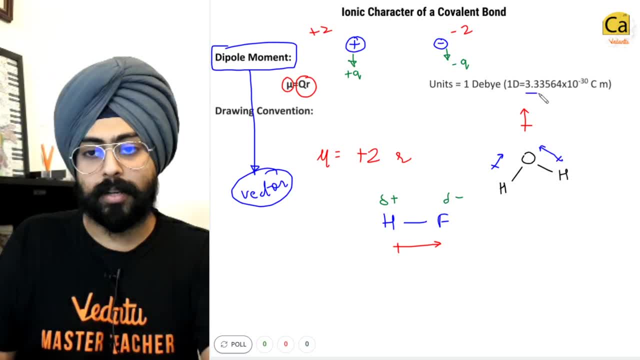 is a large increase in the size. size And, yeah, Пом is something different here, But actually, dipole moment they are one Debye, which is 3.33 x 10 to the power minus 30 coulomb meters. 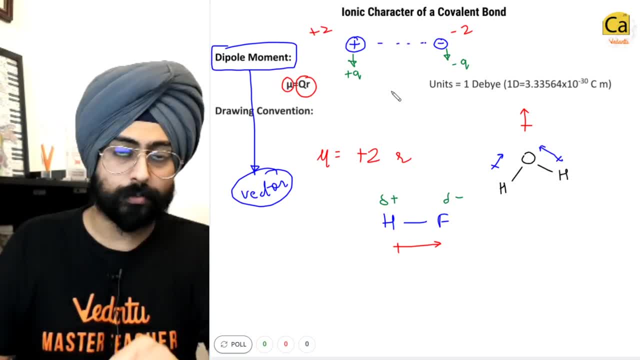 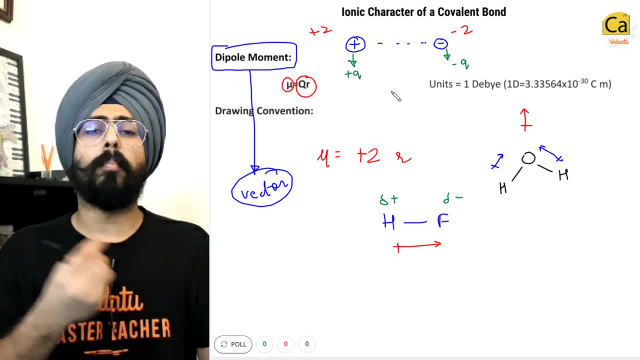 okay, so charge as well as distance is taken care of in chemistry. we talk about dipole moment mostly in qualitative terms, not in quantitative terms. we use it just to compare one thing with the other. fine, so this defines the ionic character of a covalent bond. now 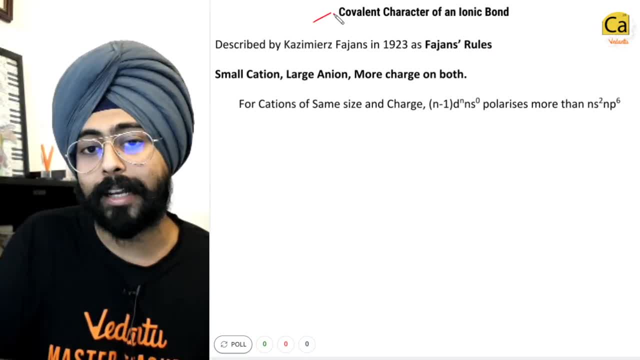 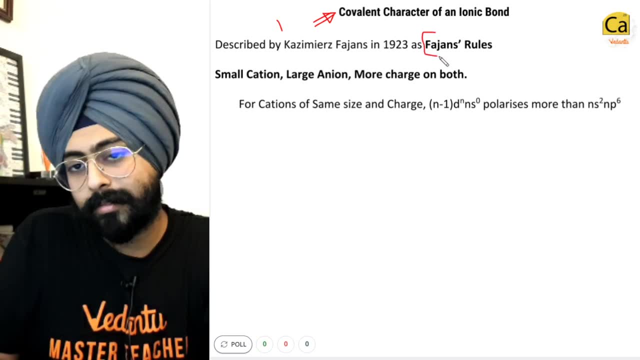 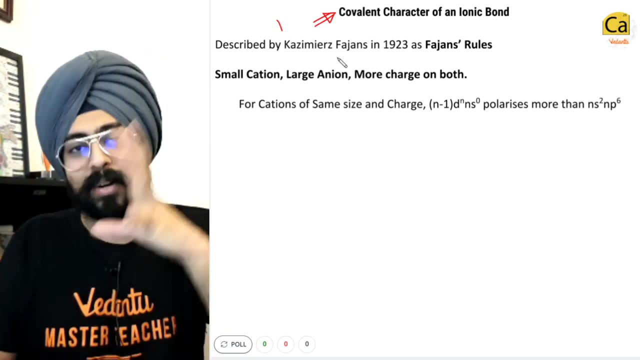 moving forward. let's think about the covalent character of an ionic bond. yes, this was described in 1923 by Kazimir's Fayans, and obviously Fayans rules. in India it's popularly known as Phajan- yeah, Phajan's rules. so what he said was that, in case you have a small cation, 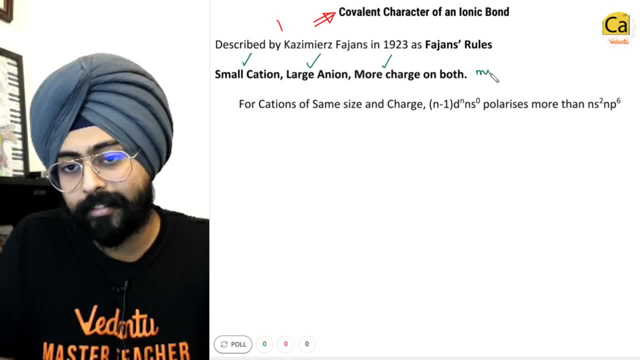 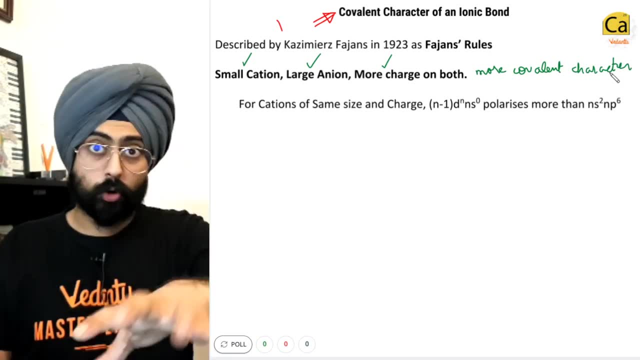 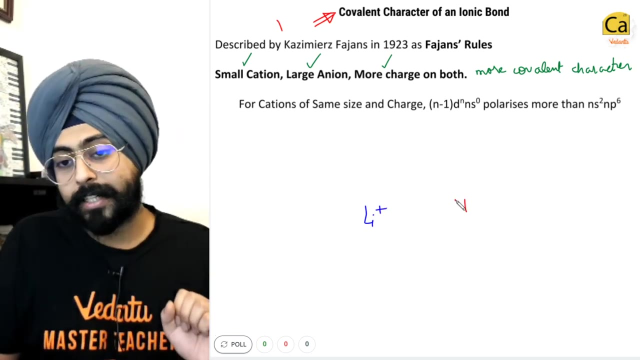 large anion and more charge on both, you will have more covalent character. okay, more covalent character if these conditions are satisfied. so in case you have lithium positive, very tiny covalent character, It, let's say, is binding itself with iodine negative. iodine's electron cloud is large. 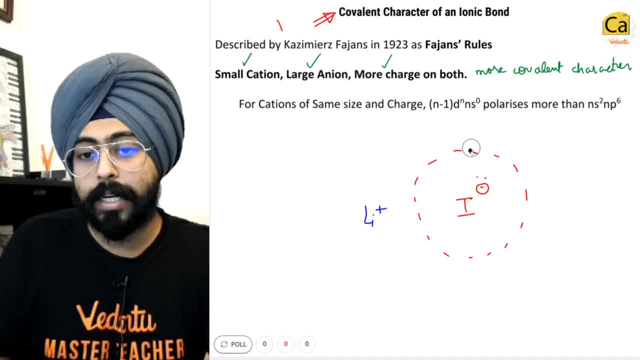 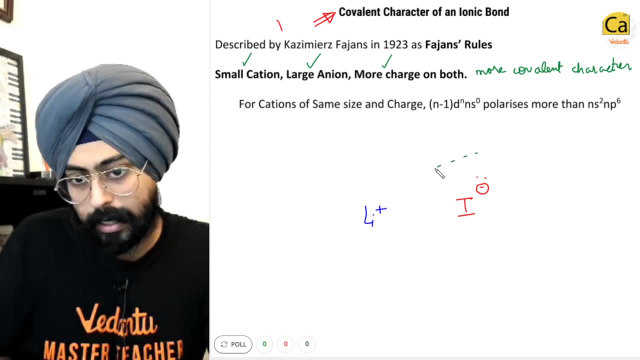 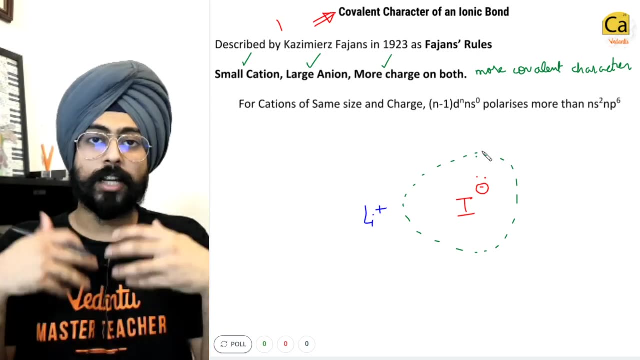 because it's a huge halogen. but what will lithium do? lithium will influence this electronic cloud and polarize it towards itself. so kaise ho jayega? the electron cloud of iodine will be distorted towards lithium. this distortion is known as polarization and smaller the cation. 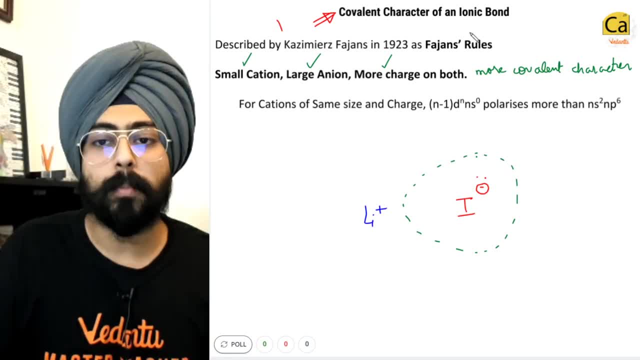 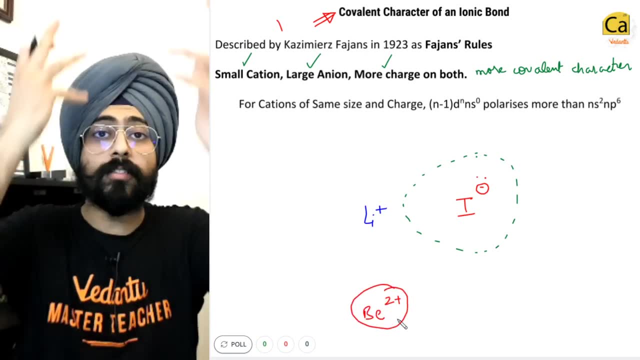 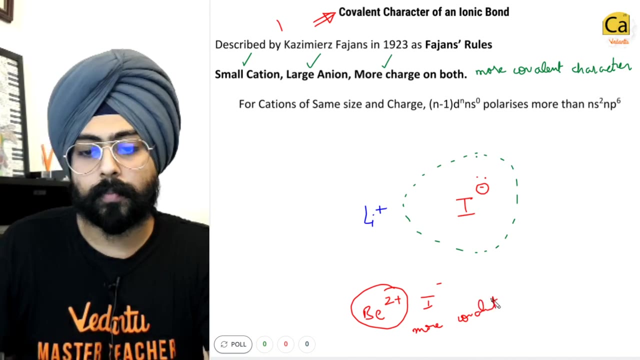 more the charge on the cation, more is the polarization Power. okay, fine, if iodine was binding with beryllium 2 positive, this would be even more covalent. okay, if it was binding with iodine negative, this would be more covalent, fine. 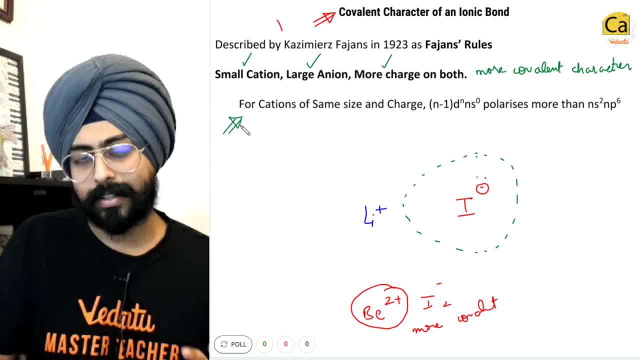 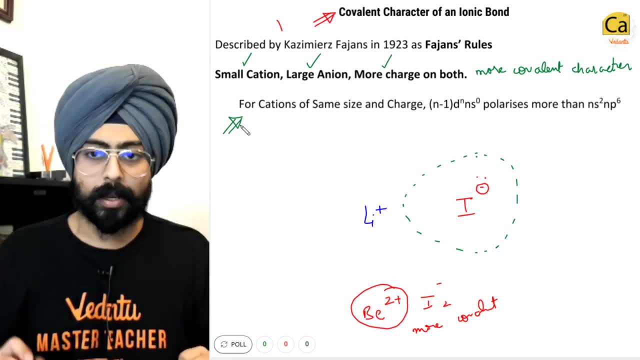 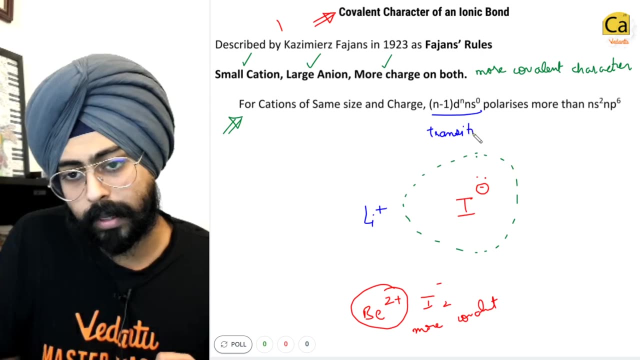 cool, very simple. now the last point that is written over here is very interesting. it says that for cations of same size and charge n minus 1, dnns0 polarizes more than ns2np6 in transition metals. it simply means that transition metals, if you have the same charge and the 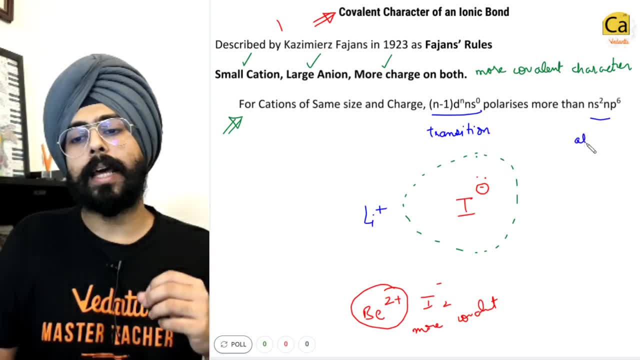 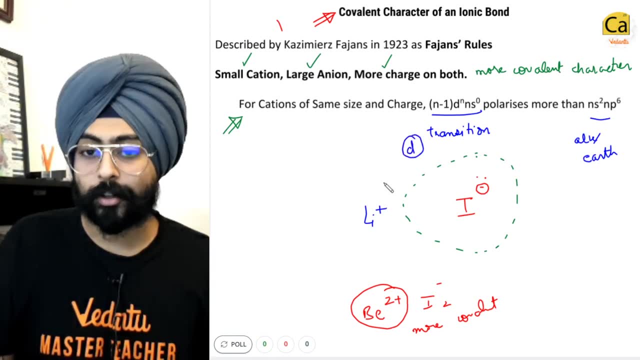 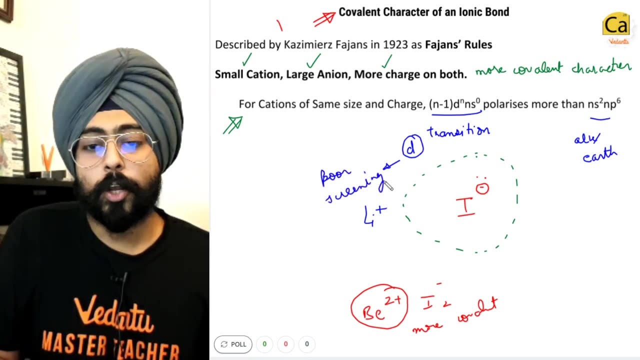 same size transition metals will polarize more than alkali or alkaline earth metals. why so? because in transition elements you have d orbital electrons, and d orbital electrons have very poor screening effect. everyone knows that. So because of the poor screening effect their nuclear charge can traverse better. it can. 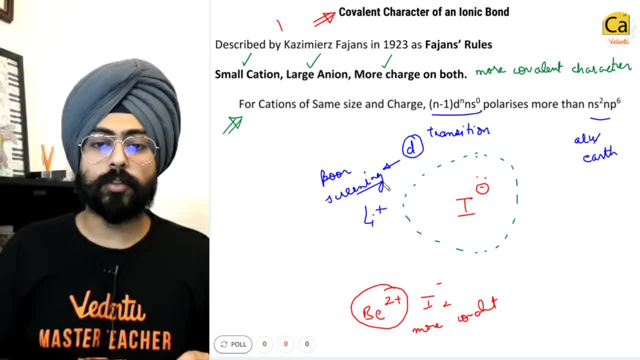 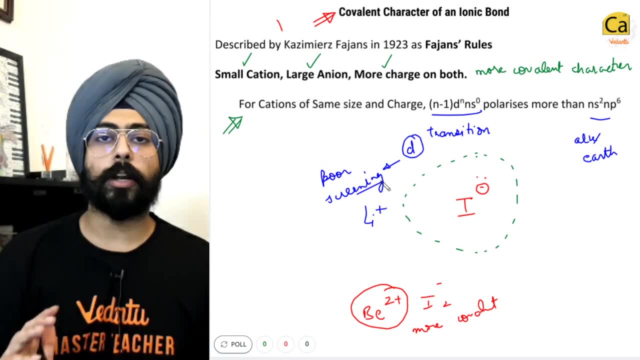 influence the ions, Hence the anions better and hence polarize more. so in case you have a transition element and an alkali or alkaline earth metal of the similar size, then give priority to transition element for polarizing power. this was about fayans rules, okay. 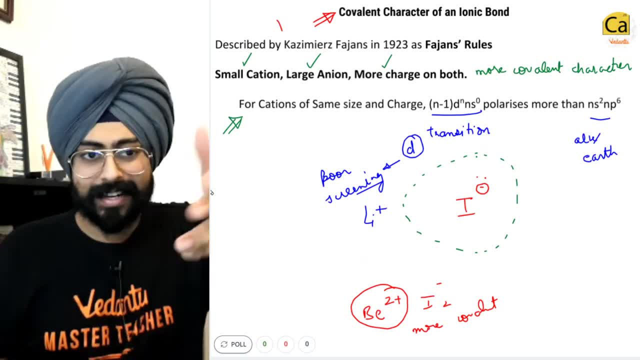 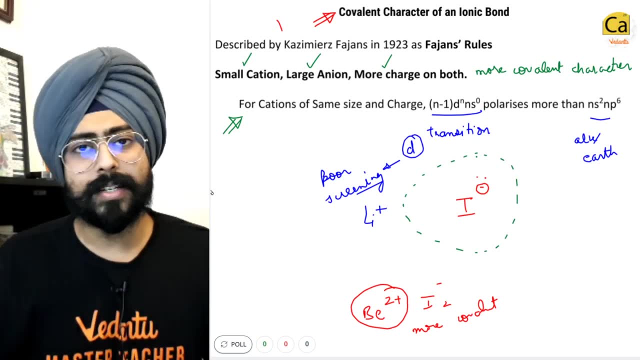 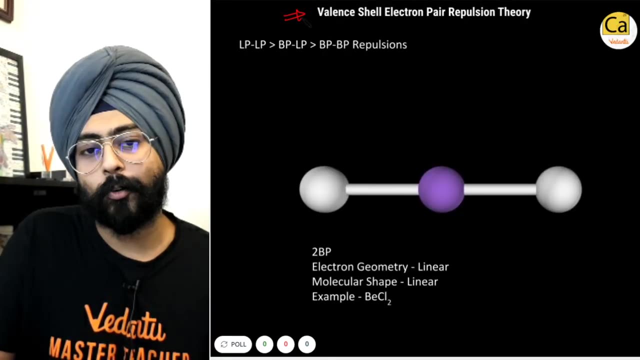 Now comes the idea of shapes. till now, what we've done? we've understood what are the different kinds of bonds, what are their characteristics- positive charge, negative charge, etc. but we still haven't talked about the shapes. So for shapes, As you all know, our very favorite theory of valence, shell, electron pair repulsion- comes. 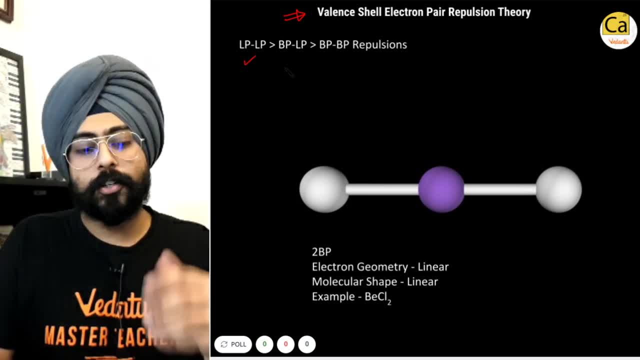 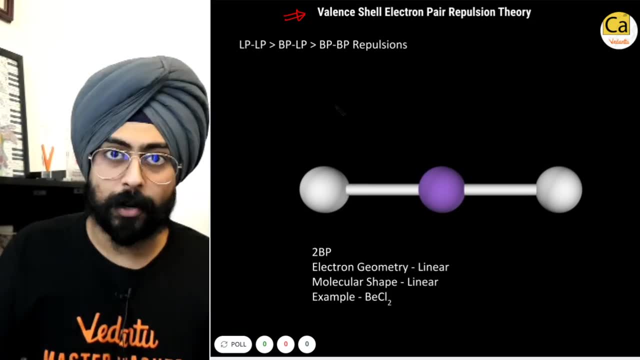 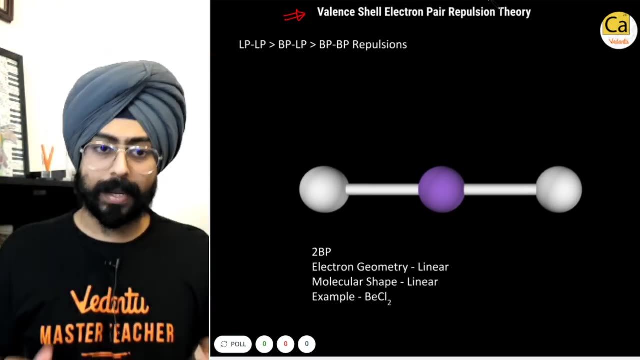 into picture. what it says is that lone pair- lone pair repulsions are more prominent than bond pair. lone pair repulsions are more prominent than bond pair. bond pair repulsions, yes. So in order to minimize these repulsions, the molecule will take a certain shape, and there 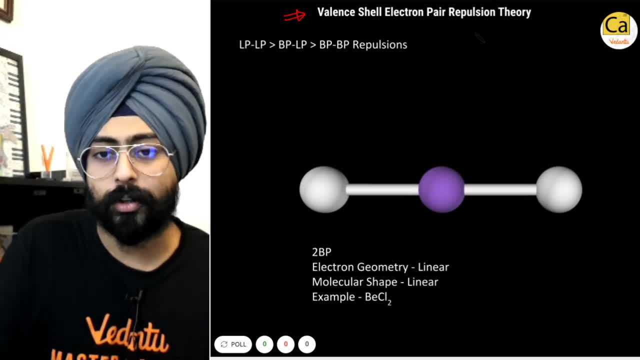 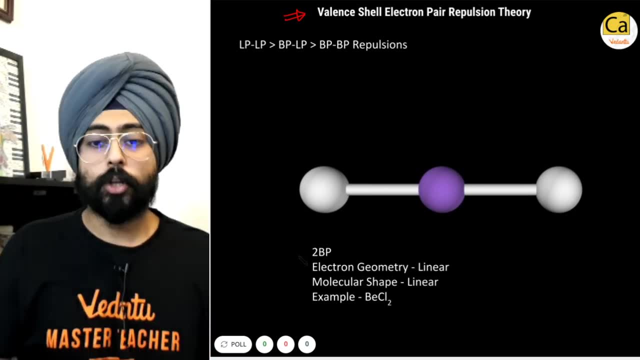 are a lot of cases in valence shell electron pair repulsion theory, better known as VSEPR. yes, Yes, So quickly. we'll revise all of those cases with one one, one example of each. so the first case that I've taken over here is the one with two bond pairs. all right, there is one. 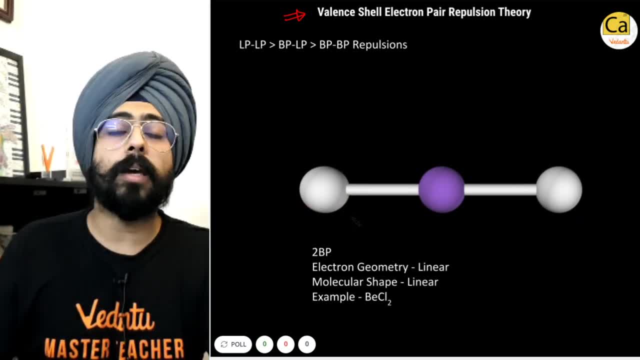 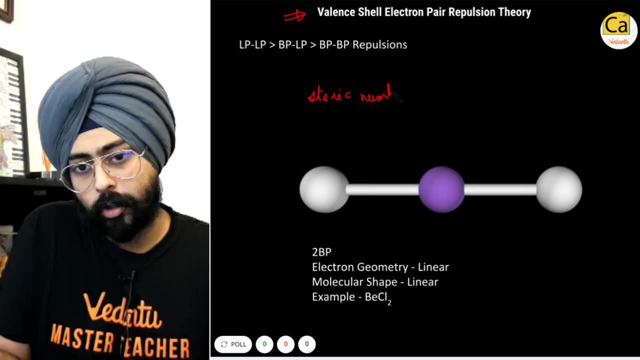 central atom and around it there are two bonded pair of electrons. my dear friends, let me remind you of something called the steric number. do you remember what is steric number? steric number is simply equal to the number of bond pairs plus the number of lone pairs around. 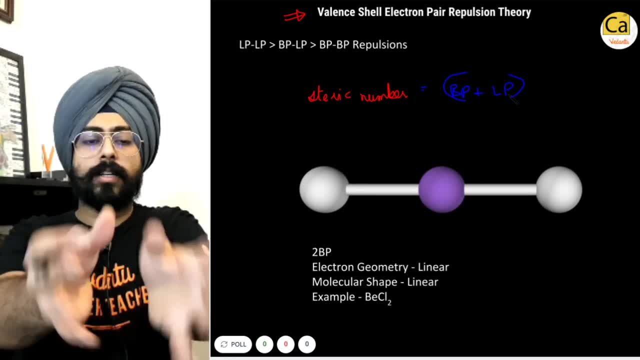 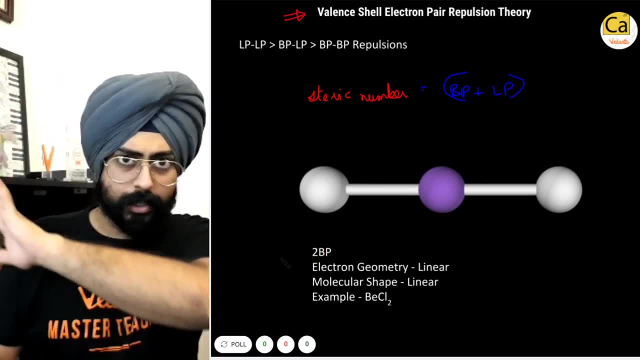 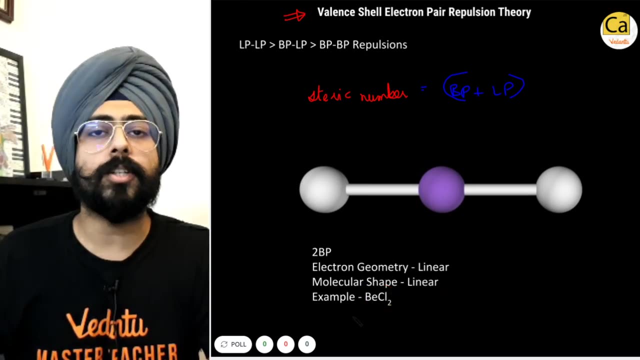 the central atom. Yes, Yes. So we'll keep on increasing a steric number in these examples, eventually. so the first example is of steric number two, only two bond pairs. in these two bond pairs, the geometry is linear, the shape is also linear, and an example could be BECL2. my dear friends, when 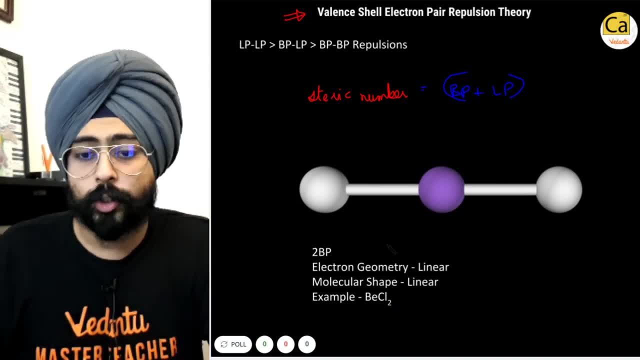 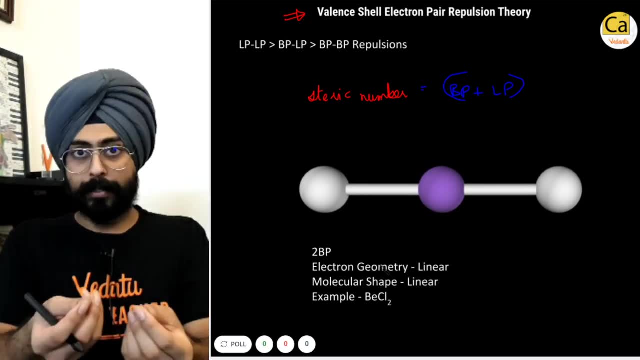 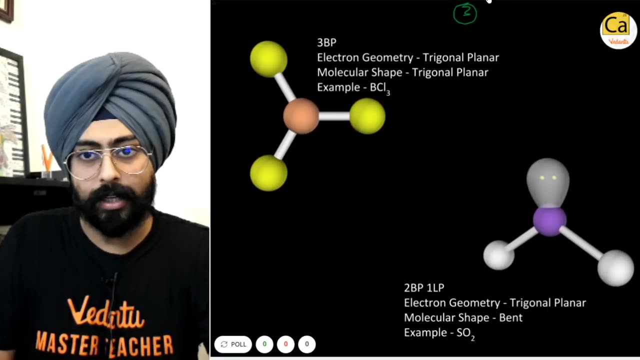 the steric number has only bond pairs in it, geometry is equal to shape. okay, only bond pairs. geometry will be equal to shape. but whenever there are lone pairs, then my geometry and shape will be different. For example, if we move on to the steric number three. okay, what are the cases over here? first, 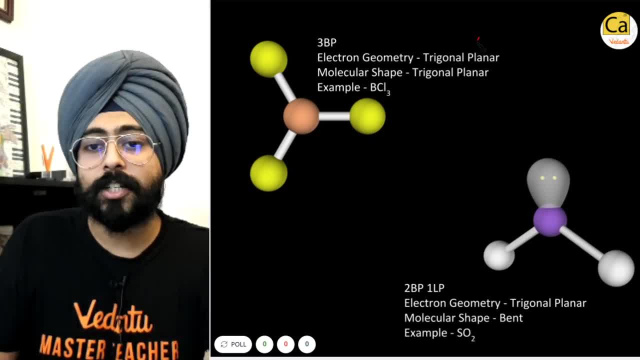 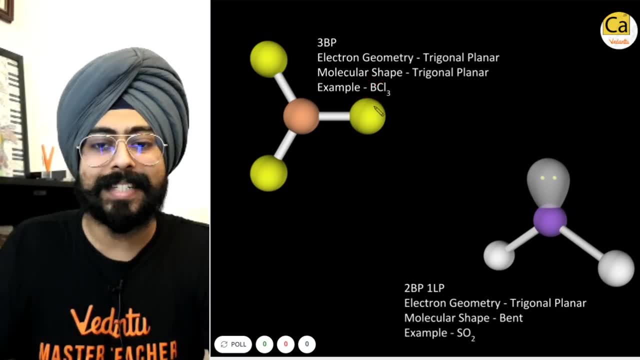 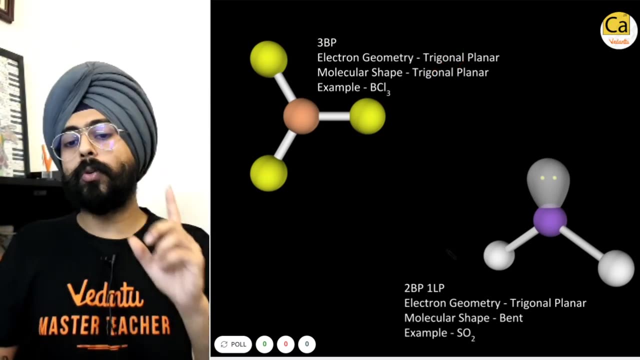 case is three bond pairs. electronic geometry is trigonal planar and molecular shape is also trigonal planar. one very good example of this is: BCL3 says there are only bond pairs: trigonal planar geometry, trigonal planar shape. but now let us look at a distortion. okay, so 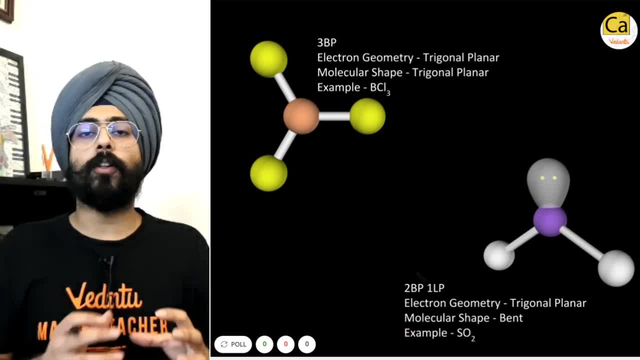 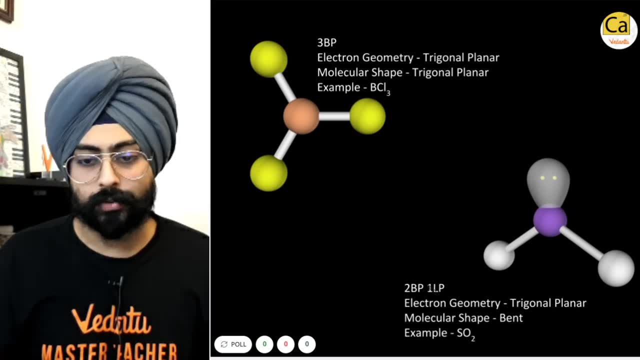 the first case, The case without any lone pairs, let's call them standard cases, and the cases with lone pairs, let's call them distorted cases. fine, so in the first distorted case over here you have one lone pair, two bond pairs. electronic geometry is still trigonal planar, can you? 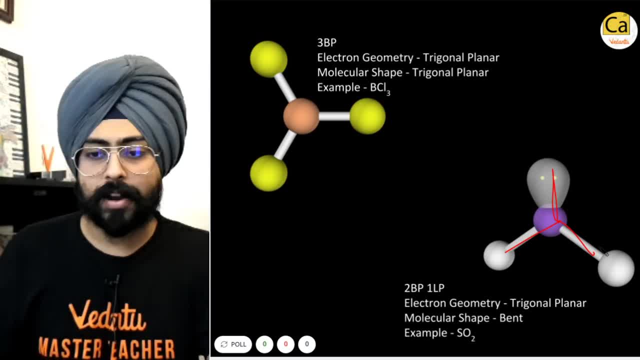 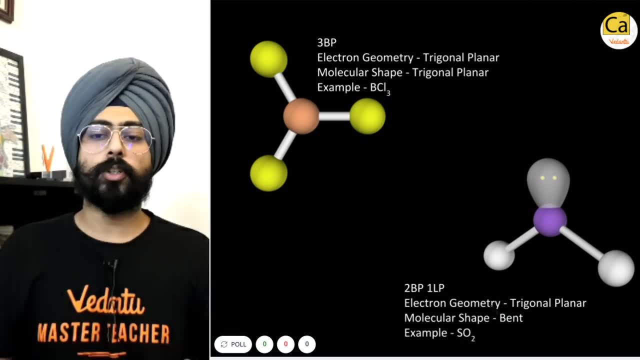 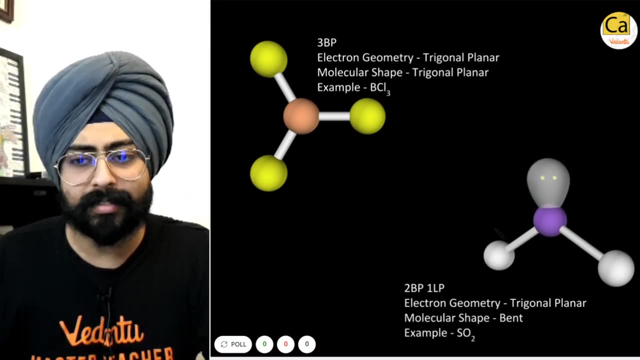 see, electrons are still oriented in this trigonal fashion, but the molecular shape over here is bent. why so? because if I'm looking at the molecule shape, do you realize that these lone pairs that I've drawn, This particular lone pair that I've drawn, It is a part of the central atom itself. it's residing in the orbitals inside the central. 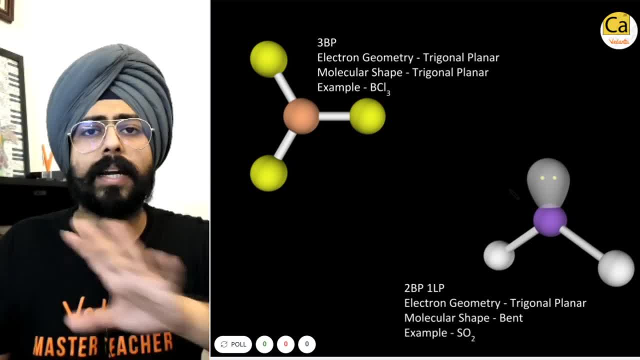 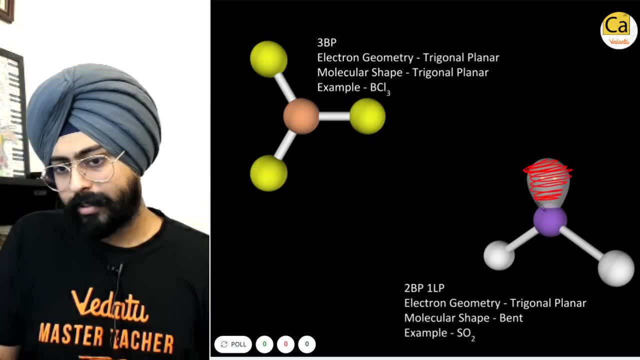 atom, isn't it? so this lone pair over here is just for representation. okay, in reality, when you're looking at the shape and, let's say, spectrometer, this lone pair will not be visible. so the shape that you have is just this much, and the shape hence is a bent shape. 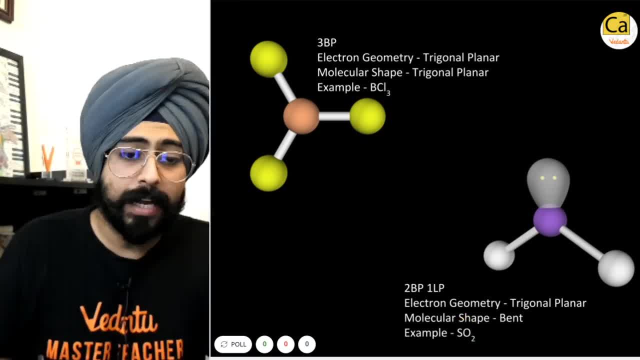 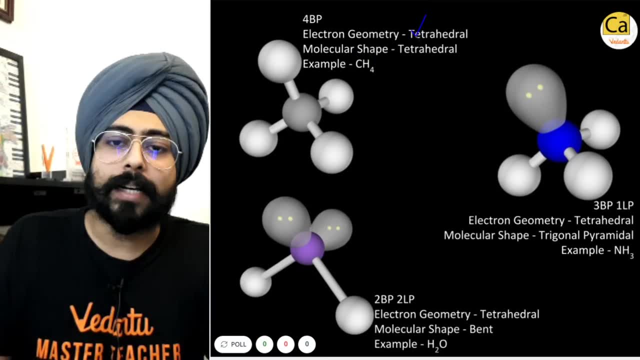 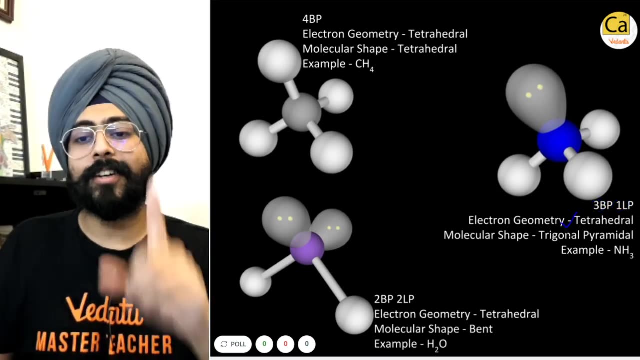 a very good example of this would be SO2. fine, let's move on. now comes steric number equal to four. Standard case is CH4. tetrahedral geometry, tetrahedral shape. very simple then the first deviation: three bond pairs, one lone pairs. tetrahedral geometry, but the shape is trigonal. 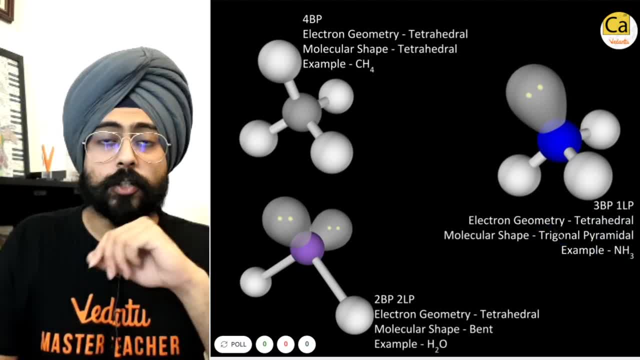 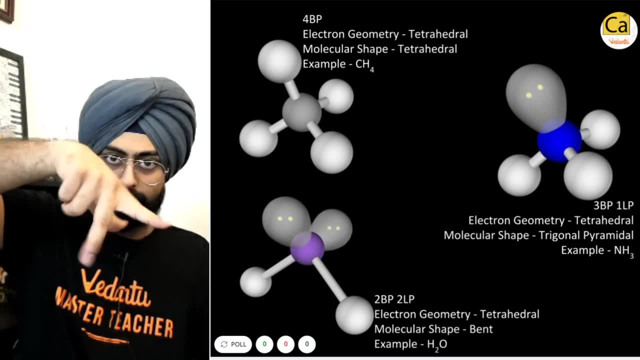 pyramidal example would be ammonia. why so? can you see the trigonal over here? can you see the triangle? triangle implies triangle, but in the triangle there is a protrusion towards the top. instead of being a flat triangle like trigonal planar, Now there is a pyramid kind of triangle. 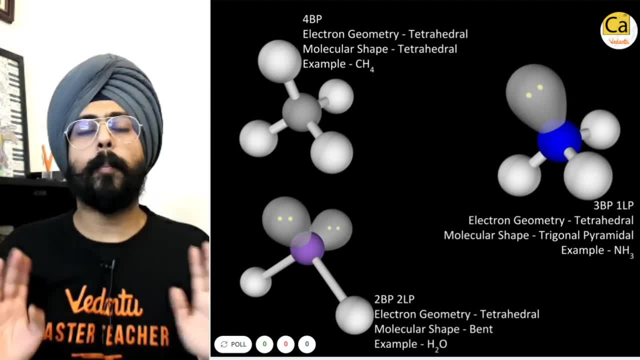 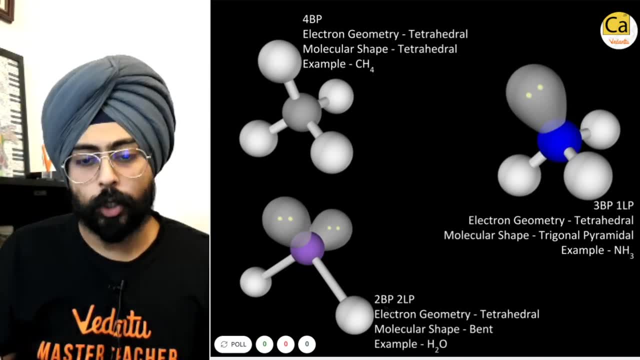 Now there is a pyramid, kind of triangle. Now there is a pyramid kind of a structure. yes, that is why pyramidal, this protrusion is called pyramidal. Then we come to the next distortion: two bond pairs and two lone pairs. so over here, electronic. 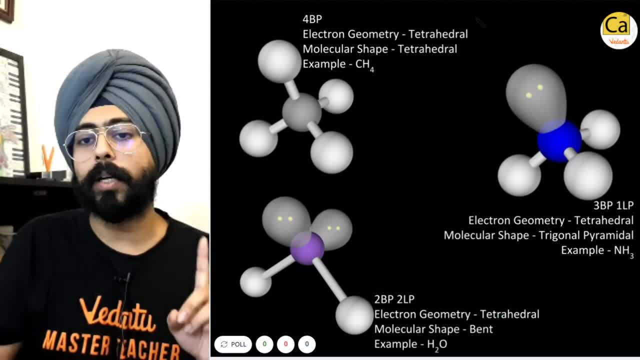 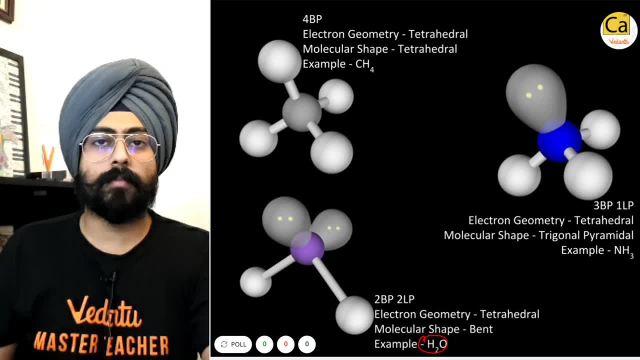 geometry is still tetrahedral. I'm pretty sure you can see that in the diagram. but if you ignore the lone pairs and just look at the bond pairs, their shape is bent. and this is the very famous water. we drink it every single day. fine then, moving on to steric number. 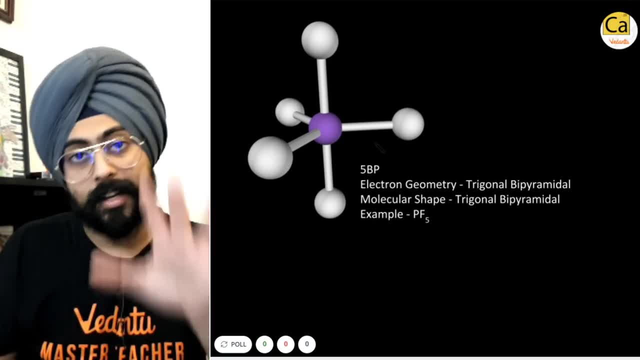 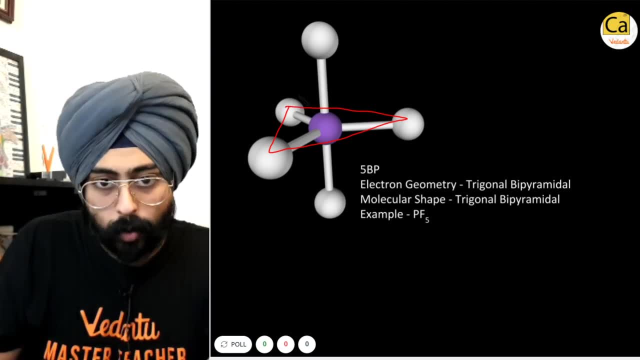 equal to 5. Five bond pairs. standard case: triagonal bipyramidal. I am pretty sure you can notice this triangle. There is one protrusion on the top, one protrusion on the bottom. So triagonal bipyramidal. 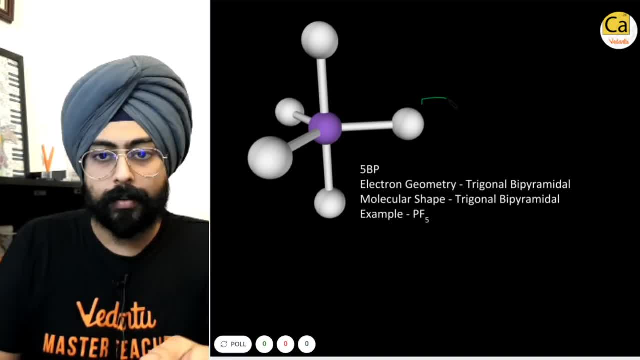 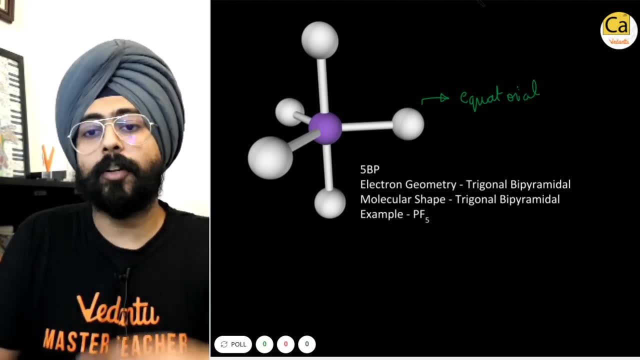 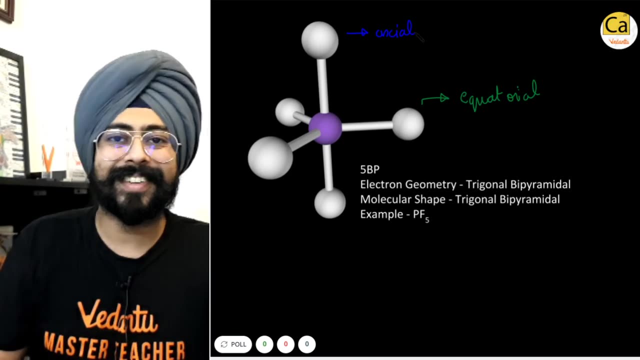 Yes, So the bonds over here that are on the triagonal, these bonds are known as equatorial bonds. Yes, And the bonds that are the straight ones on the top and the bottom, these are known as my axial bonds. Very simple. 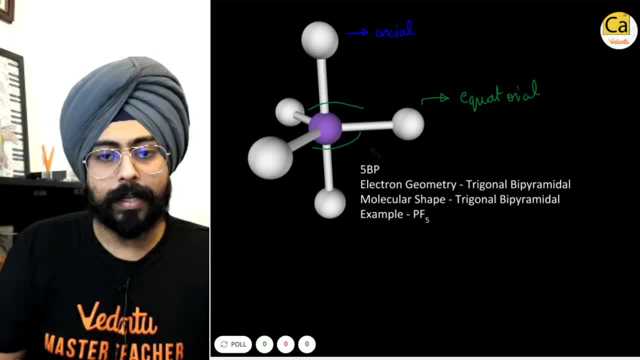 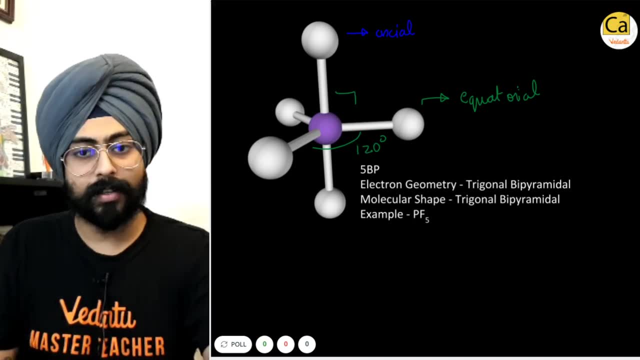 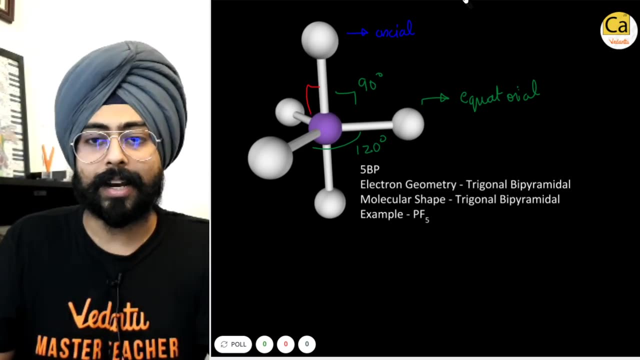 Now realize that equatorial bonds have two 120 degree interactions. Yes, Two 120 degree interactions, and they also have two 90 degree interactions, Isn't it? But if we look at the axial case, the axial case is facing three 90 degree interactions. 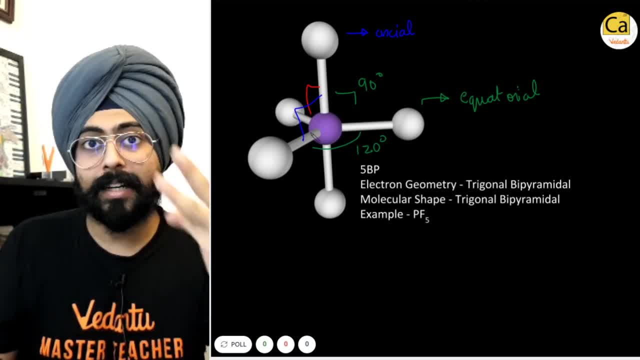 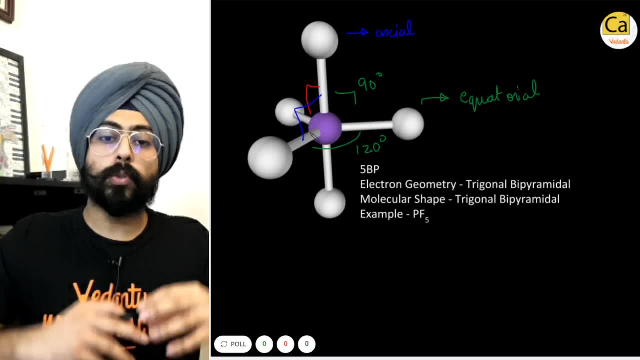 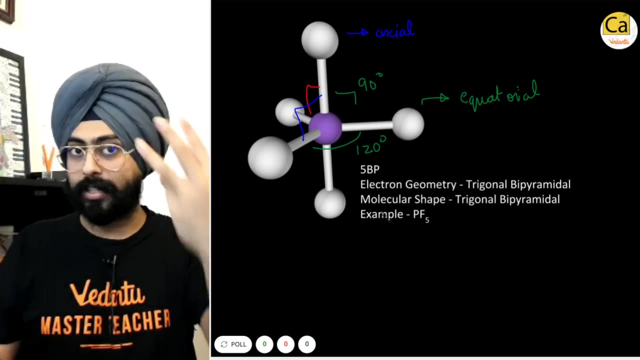 Isn't it? Yes, Three 90 degree interactions versus two 120 degree and one 90 degree interactions. Do you realize that three 90 degree interactions will cause a lot of repulsion? Yes, So even though in equatorial there are two 90 degree interactions, in axial, because of three 90 degree interactions, there is a lot of repulsion. 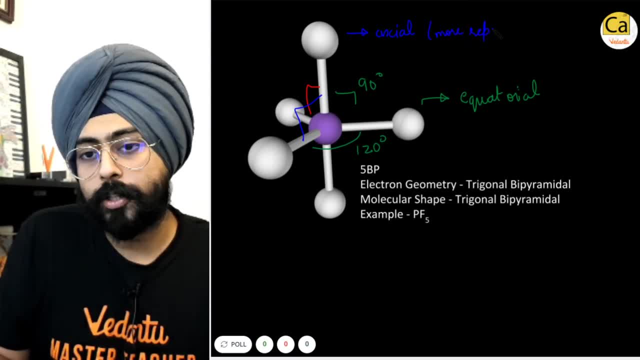 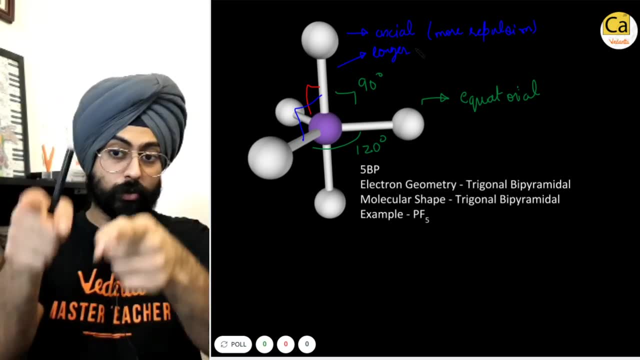 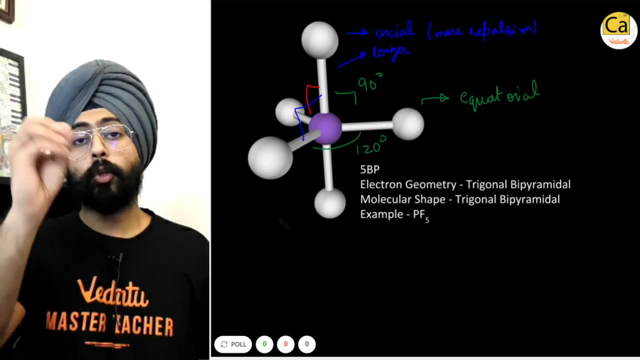 So axial faces more repulsion. Remember this. Okay, Axial bonds are longer than equatorial bonds in the case of triagonal bipyramidal. Please remember that. So whenever in the distortions we put any lone pairs into triagonal bipyramidal, you will always put them in the equatorial position. 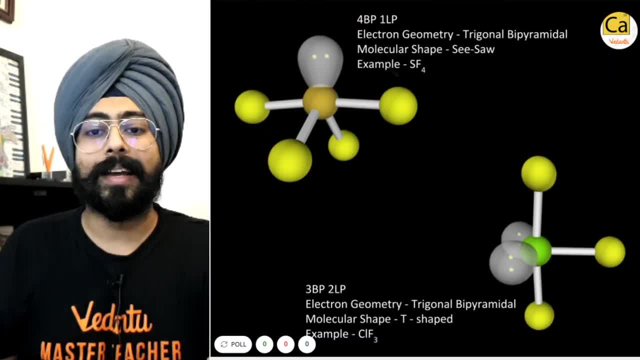 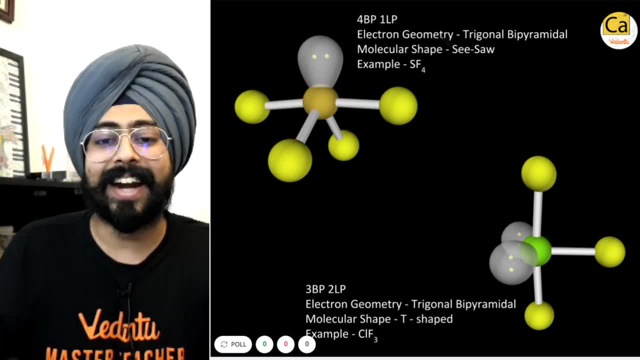 Let's see the distortions: Four bond pairs, one lone pair. Electronic geometry is triagonal, bipyramidal, but the molecular shape is seesaw. Can you see the seesaw? I guess, And the example could be SF4.. 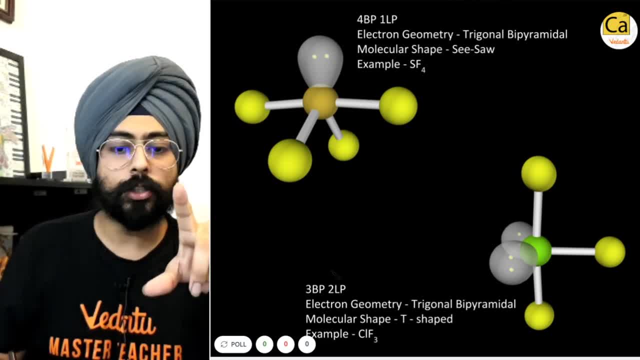 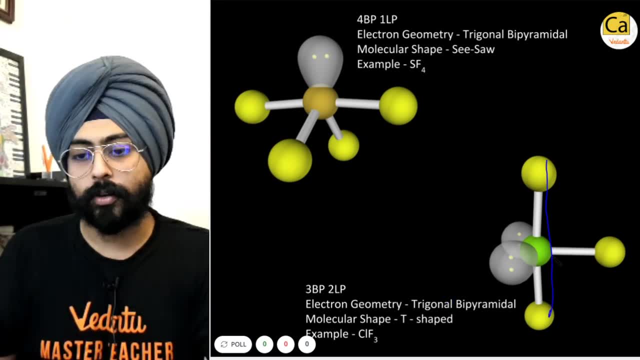 Fine. Similarly, at the bottom you have the next distortion: Three bond pairs, two lone pairs. The steric number is still five, So geometry will still be triagonal, bipyramidal, But the molecular shape, as you can see over here, it's a T-shaped molecule. 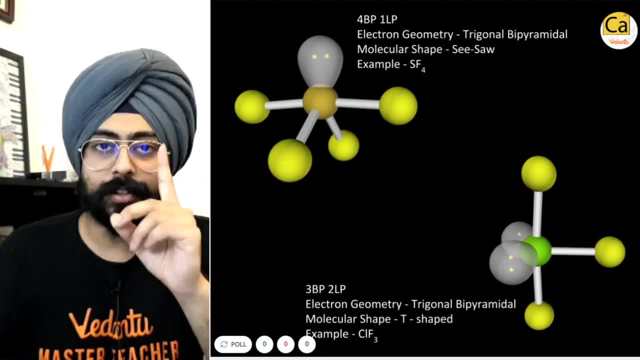 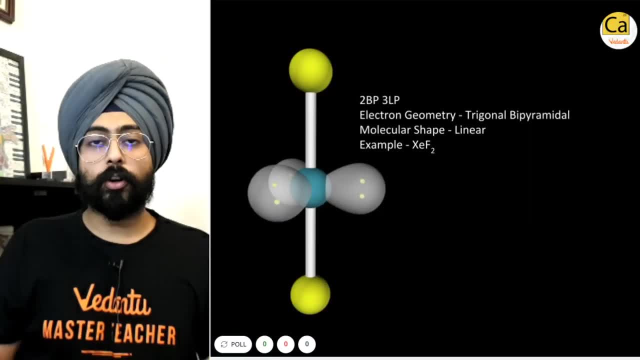 A very good example would be CLF3.. In case you people are feeling that this is fast, then please pause the video and you can look at the structures. Speed is of the essence right now. Now moving on to the next distortion. 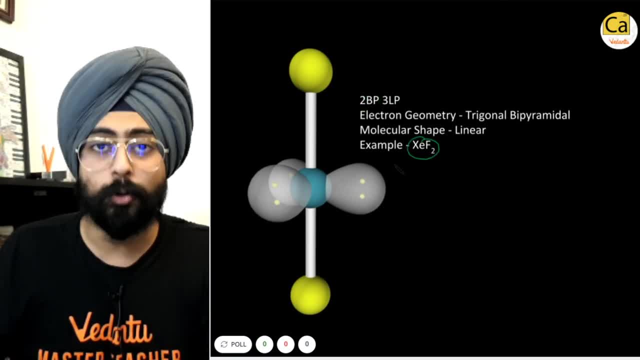 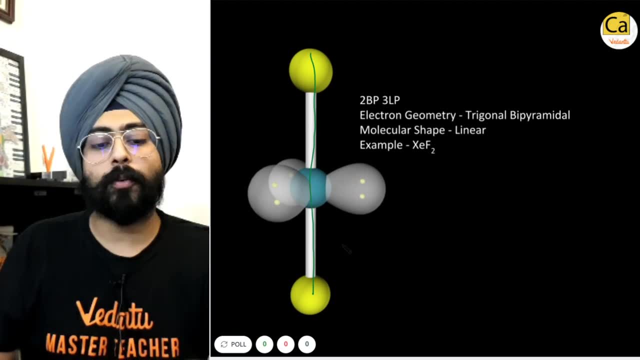 Two bond pairs, three lone pairs. A very good example would be XEF2.. And over here, if you ignore the lone pairs which are on the equatorial positions, you will realize that the shape of this molecule is absolutely Linear. 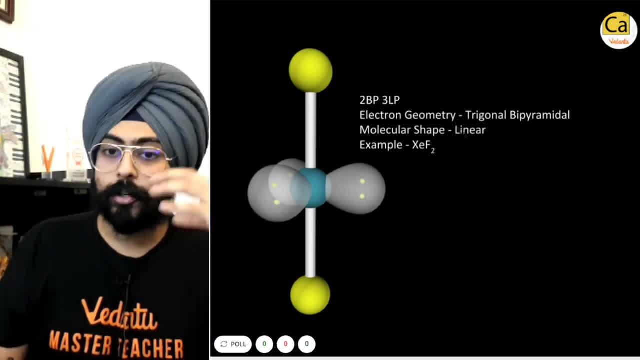 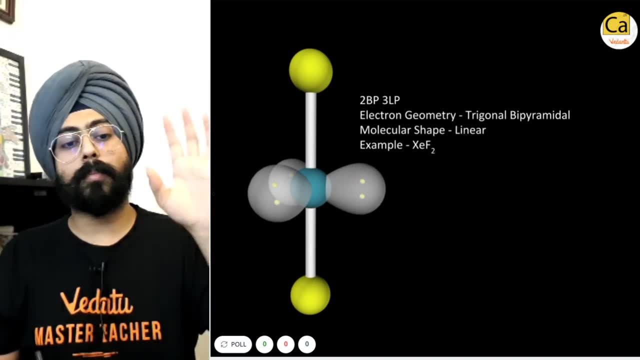 Geometry still is triagonal, bipyramidal, So geometry depends on the steric number only. Molecular shape depends on how many bond pairs and how many lone pairs there are. Once again reminding you that this video can be paused anytime in case you feel you want to look at the structures in a little more detail. 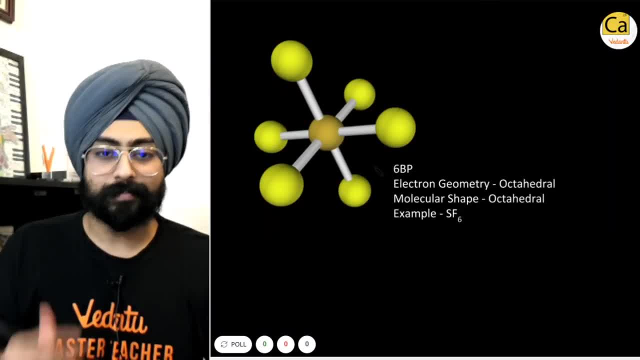 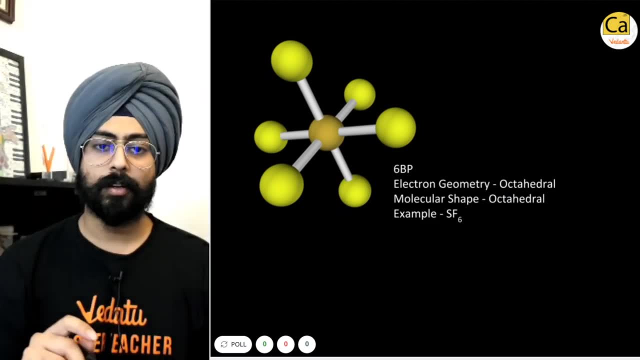 Then, moving on to the next steric number, Six bond pairs, Octahedral geometry, octahedral shape. Example would be SF6.. Very beautiful, very symmetric structure. Yes, I'm sure you can see an octahedron. 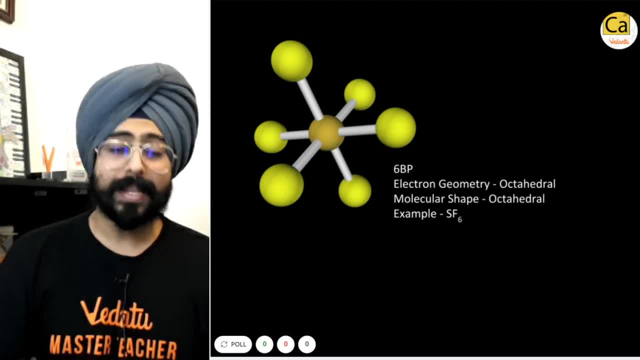 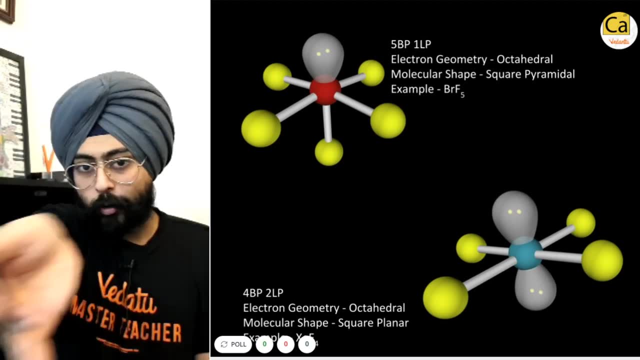 Fine, So this is your octahedral geometry. And now let's come to the distortions of this. The first distortion is five bond pairs, one lone pair. Yeah, So electronic geometry over here still is octahedral. 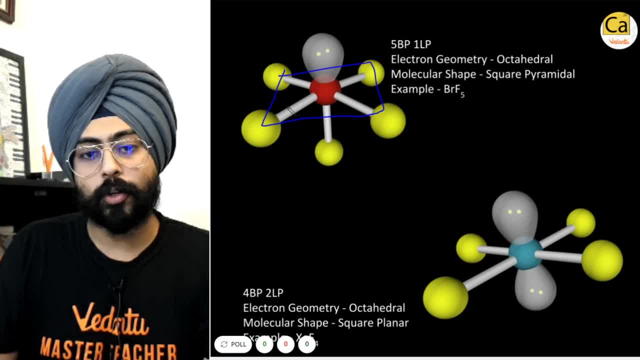 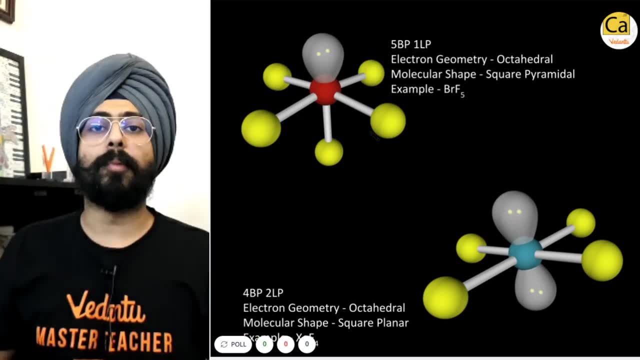 But look at the shape: A square with one protrusion towards the bottom. You could flip the structure and make the protrusion towards the top as well. So square, pyramidal, And the example's molecule would be BRF Five. 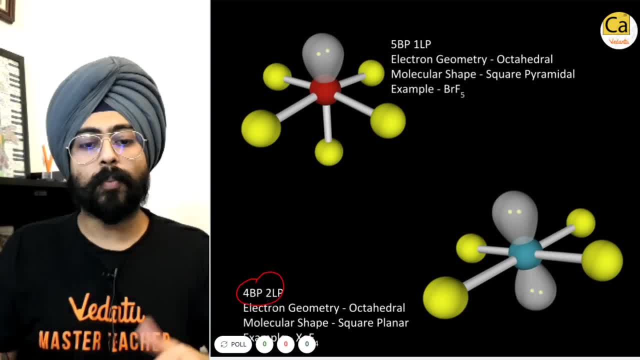 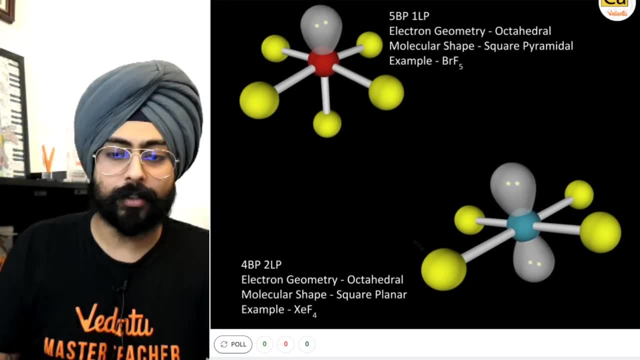 Fine. Then the next example is four bond pairs, two lone pairs, Yes, So in this particular example, what's going on? In this particular example, you have a square in the middle and no protrusions, Just a very beautiful square. 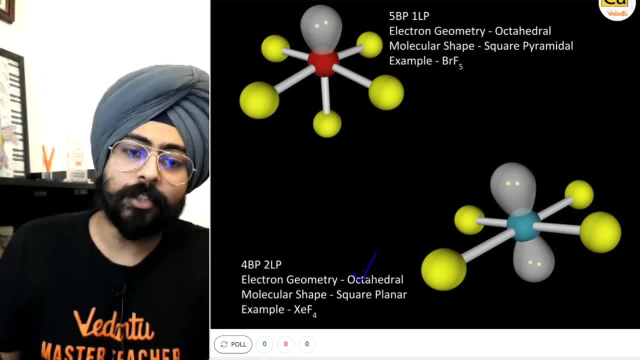 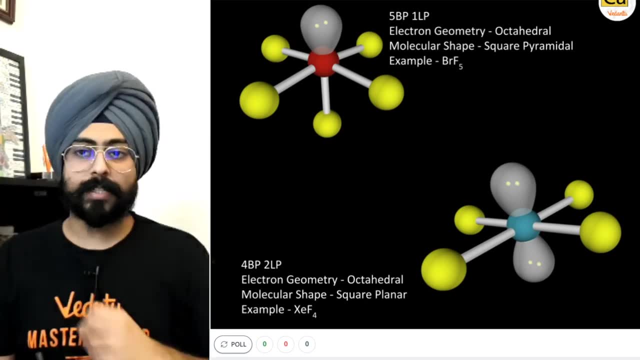 So over here you have the square planar shape. Octahedral geometry still holds true. Example could be XEF4.. Fine, And then moving on to the last case that we will look at for now. Fine, And then moving on to the last case that we will look at for now. 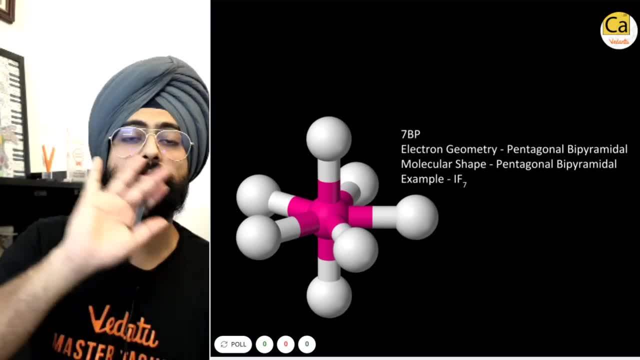 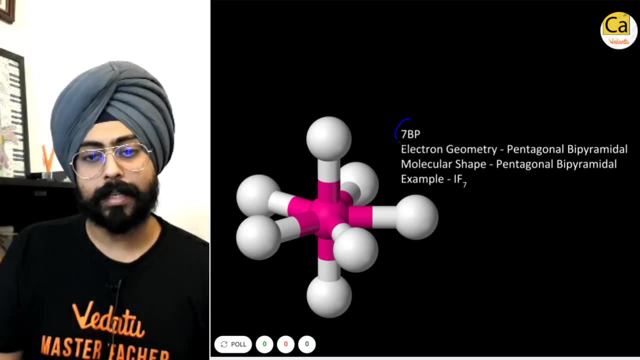 And that is the one with steric number equal to seven. This is very uncommon. Okay, This is very rare, and the distortions of this are even more rare, So we won't discuss that. Not necessary. Seven bond pairs, Electron geometry- I'm pretty sure you can see. 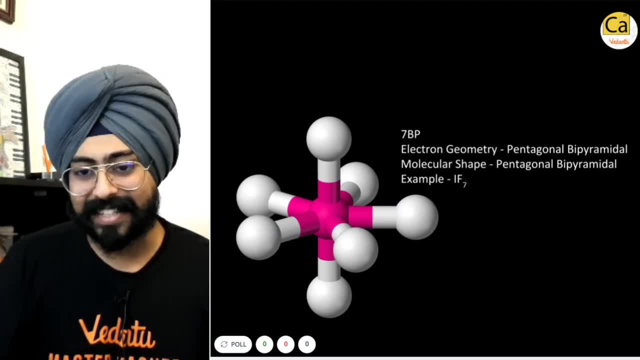 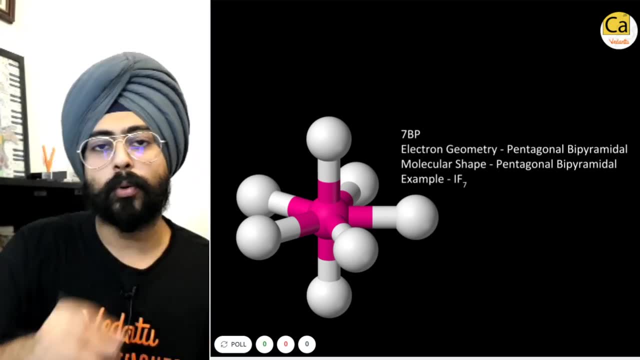 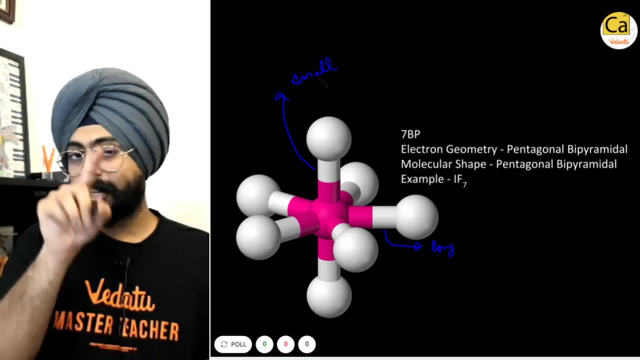 Pentagonal bipyramidal, And example is IF7.. Now I'll tell you one secret: In pentagonal bipyramidal the axial bonds are smaller, the equatorial are longer. In pentagonal bipyramidal, the axial bonds are smaller, the equatorial are longer. 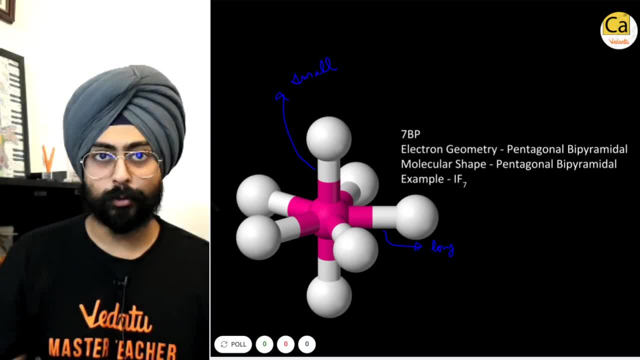 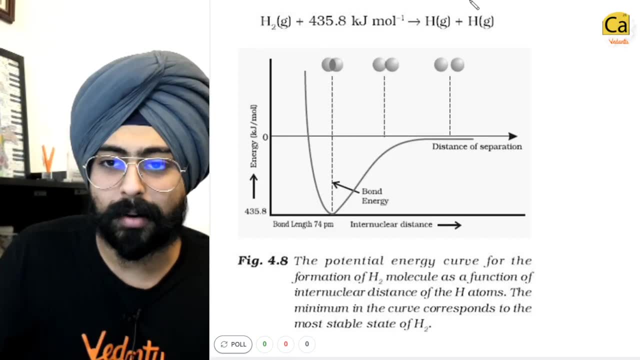 After the class, do a Google search to find that out. Okay, It'll be interesting for you to know. The idea is still repulsions. Come on, let's move on. Now let's talk about the energetics of bonding. 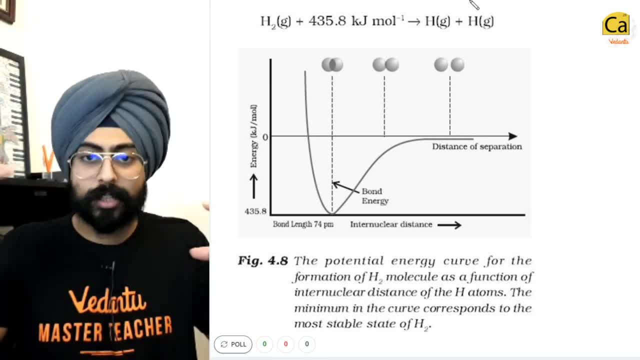 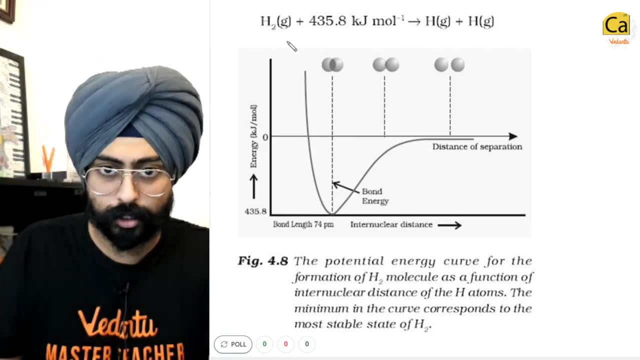 Types of bonds are done. Shapes of bonds are done. Now let's talk about the energies that are involved in bonding. So the first extensive experiment was done on hydrogen molecules, As you can see over here. I'm pretty sure you remember this energy diagram. If the hydrogen atoms are far apart from each other, there is zero potential energy. As you keep bringing them closer, their energy keeps on decreasing. They release energy to the atmosphere. Then comes a point where their energy is minimum. What is the amount of that energy? Minus 435.8 kilojoules per mole. At this point, they are at minimum energy. Minimum energy means maximum Stability. right. This distance between these two nuclei is known as the bond length equilibrium distance. This is the distance of 74 picometers for hydrogen. 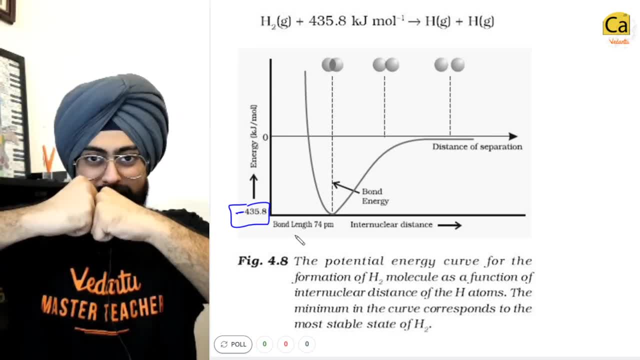 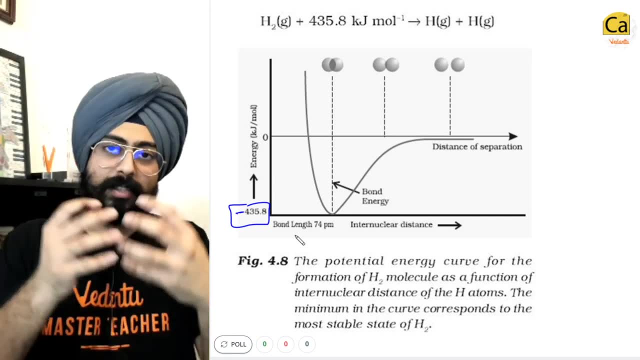 Now, if you bring the bonds a little closer to each other, more than 74 picometer- Do you realize there'll be a lot of repulsion, So they'll again start repelling each other. electrons versus electrons, Neutrons, I mean nucleons versus nucleons. 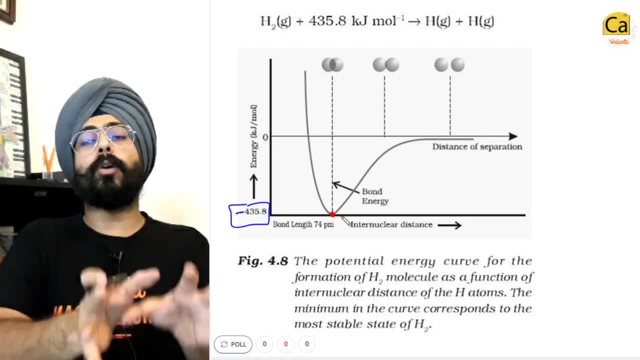 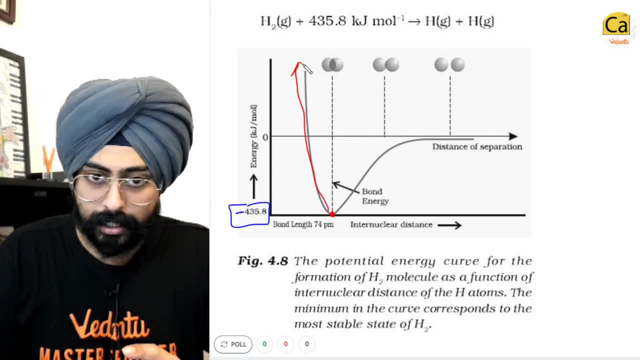 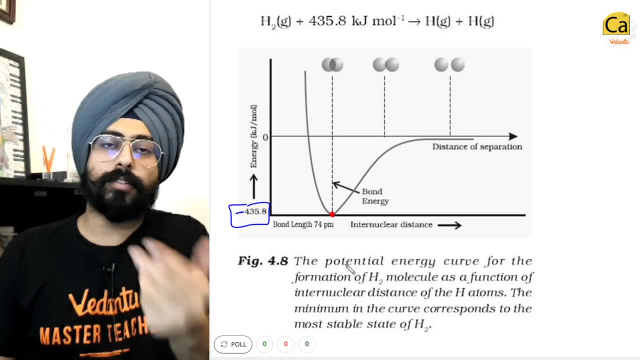 Yes, So 74 picometer. This is a very beautiful equilibrium distance where every force is balanced and they stay with each other very beautifully. Push them further and the energy keeps on increasing. OK, so this is the potential energy curve for the formation of H2 molecule as a function of distance. 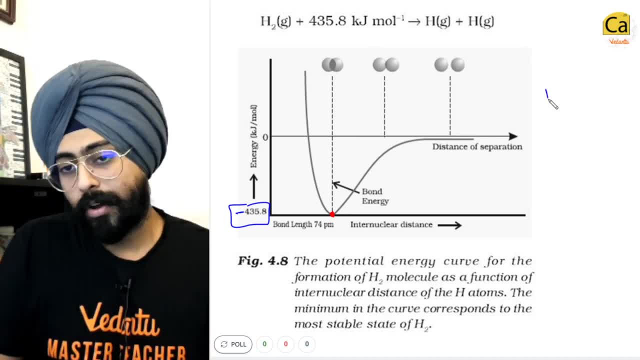 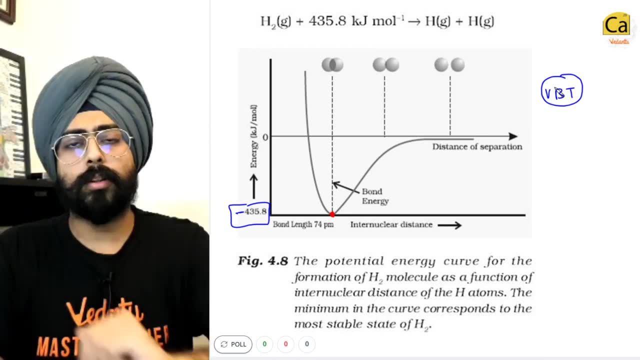 Fine. Now then comes the idea of valence bond theory, VBT. VBT is just a quantum mechanical model, But we again, since we don't want to go into the mathematics of it, we revise VBT and we study VBT only in terms of its qualitative behavior. 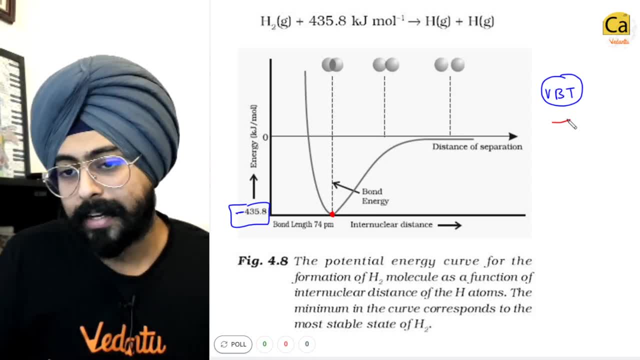 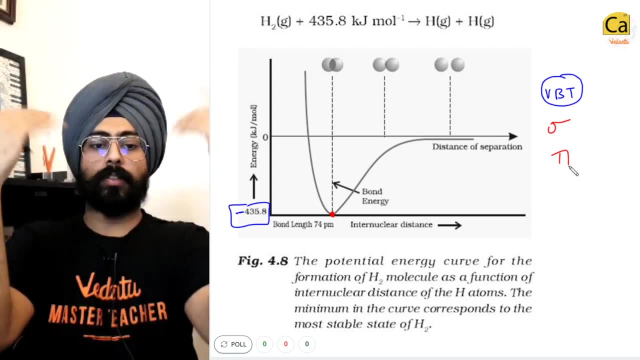 So VBT talks about types of bonds. What are the types of bonds? Sigma bond and pi bond. Yes, Sigma bond is head on overlap. Pi bond is lateral overlap. So on the next slide that I'm showing you right now, there are different. 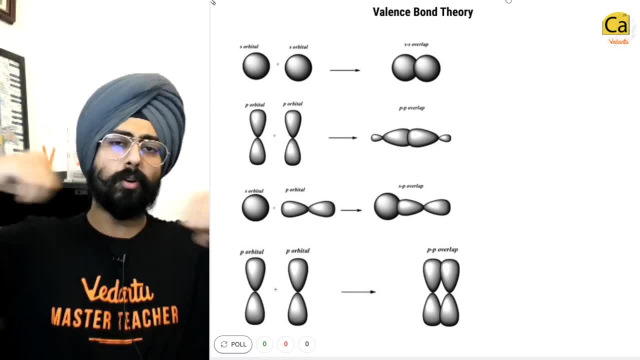 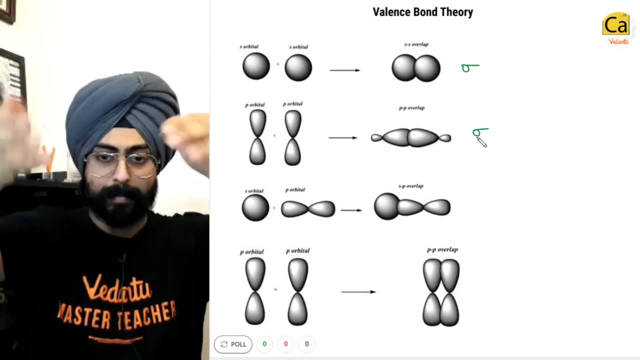 different types of bonds that are given. The first one is S, with S always going to be a head on overlap, So this is a sigma bond. The next one: P versus P. this is also a sigma bond- head on overlap. 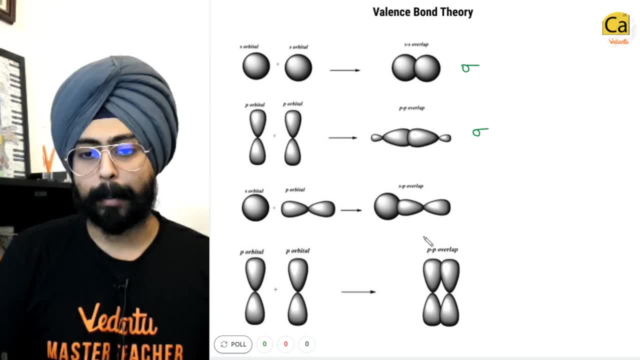 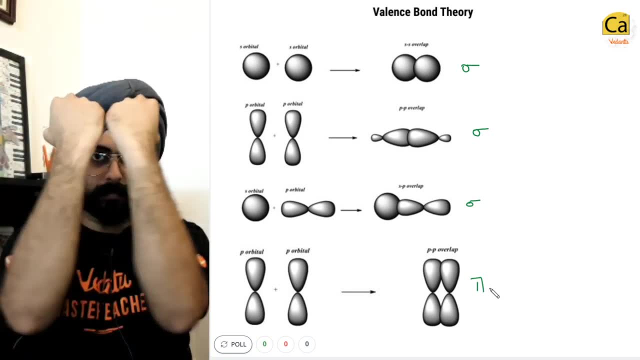 The next one S orbital versus P orbital. once again head on overlap sigma. And the last one over here is pi. Why pi? Because the overlap is lateral. If the overlap is like this, or if the overlap is like this: 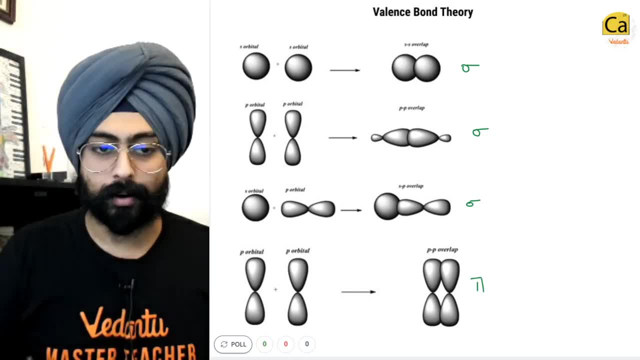 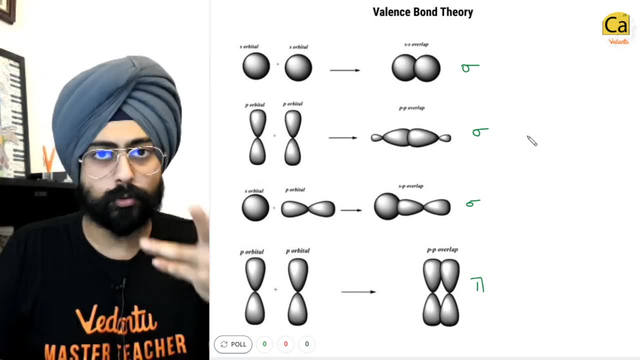 it is a lateral overlap and hence you call it a pi bond. Fine, That's how the normal picture works. Now, do you remember that in some cases, in some places, if you notice these bonds, they have given you signs on the wave function of the 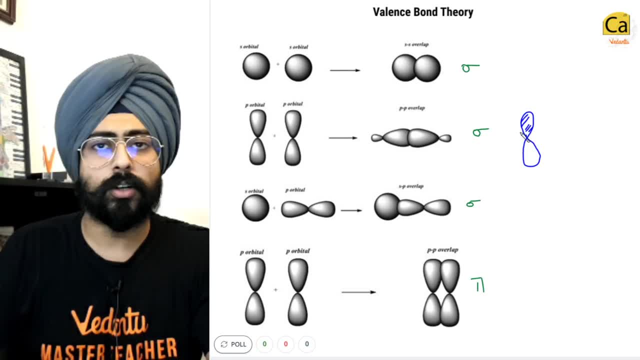 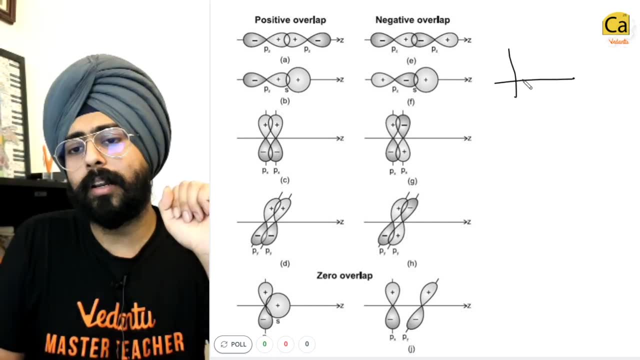 orbital, Yes, Or they sometimes color one of the lobes into one and the other lobe is of a different color. What does that mean? I'll tell you. Think about a sinusoidal wave function. Let's talk about a sine wave. 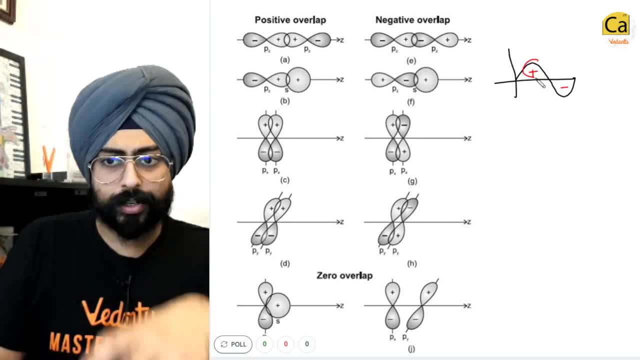 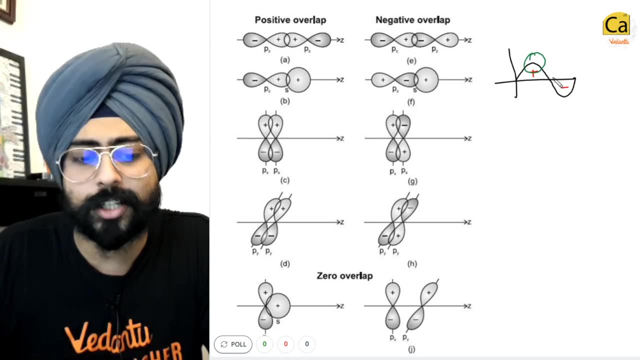 In a sine wave you have a positive and a negative side. Over here, the values of the sine are positive. Over here, the values of the sine are negative. Does this mean that the wave function is positively charged here and negatively charged here? 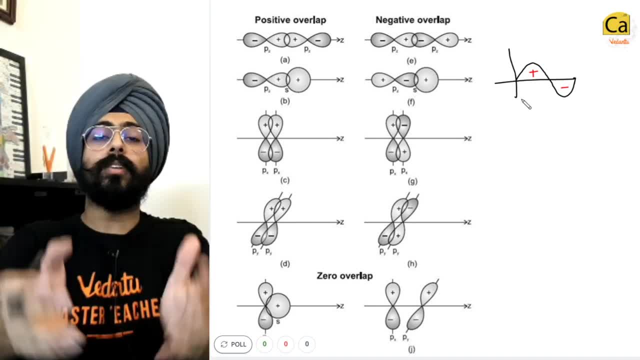 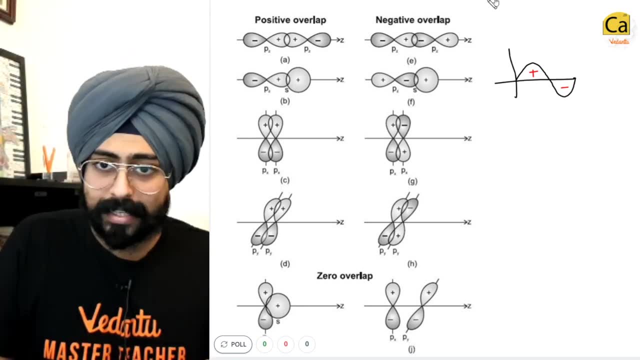 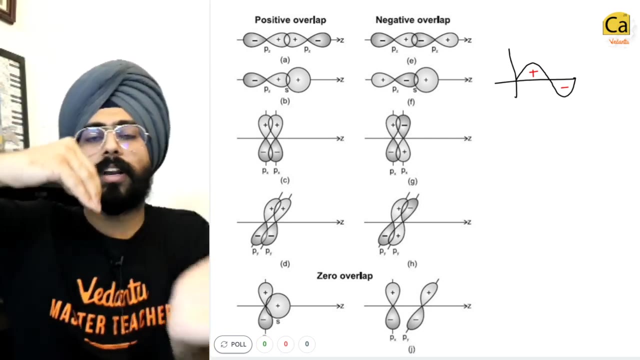 It has nothing to do with charges, It is just the sine of the wave. Similarly, since orbitals are just electronic wave function representations, OK, these signs, these positive, negative, are just signs of wave functions. And you know, for waves, if the same sine overlaps with the same sine, 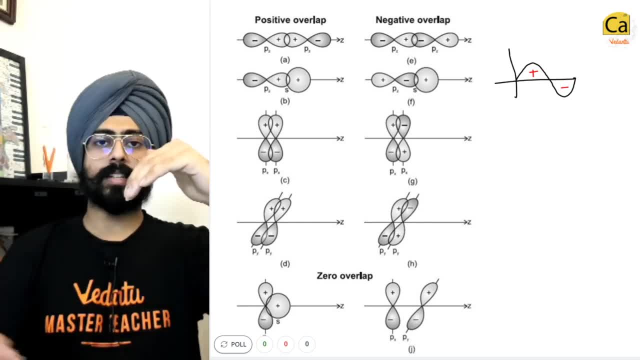 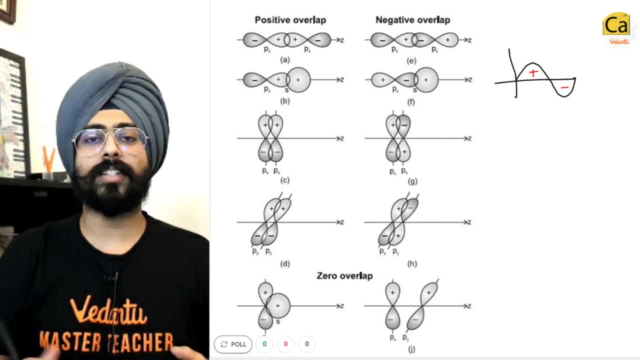 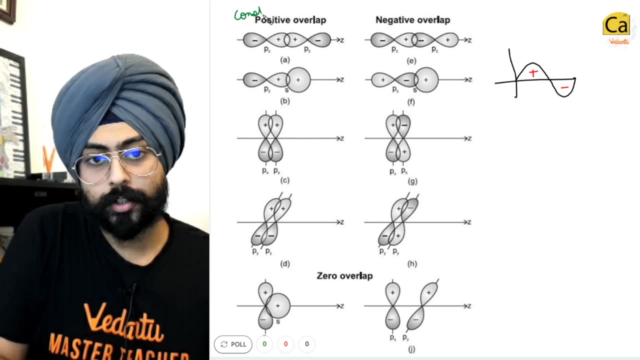 they will do constructive interference. If the positive sine overlaps with the negative sine, they will do destructive interference. Yes, So that's exactly what the significance of these signs are, And over here we have two different cases: positive overlap or constructive. 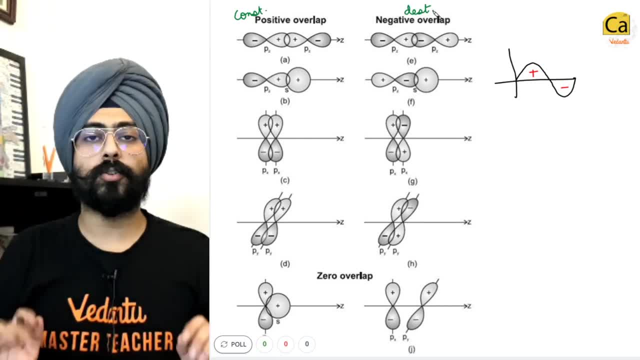 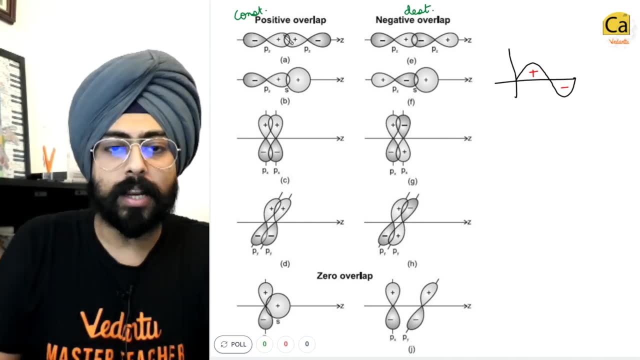 negative overlap or destructive. I'm sure you've understood about interference in waves, chapter in physics. Yeah, So on the left hand side of this page you have positive overlap, positive bonding with positive, sigma bonding, positive with positive, again sigma bonding positive with positive, negative with negative. 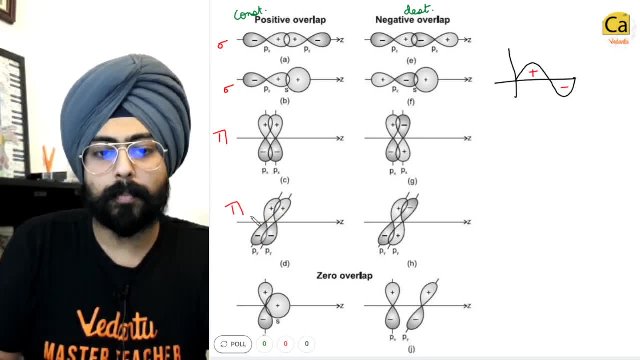 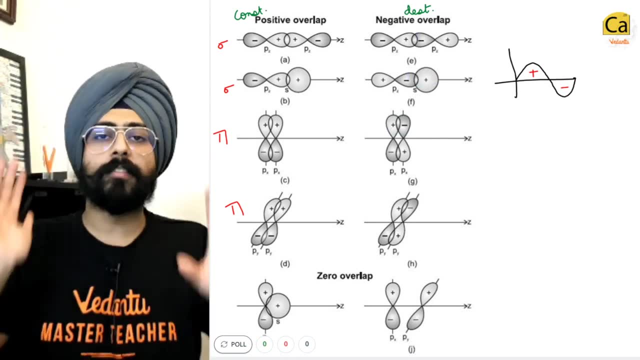 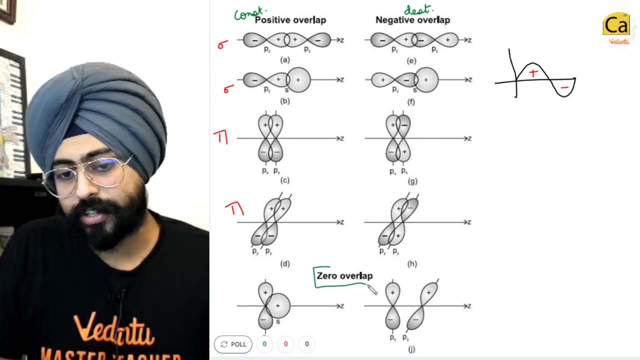 This is a pi bond: positive, positive, negative, negative. Once again, pi bond. On the right hand side you have negative overlap. They will eat into each other's wave functions. They will cancel each other's wave functions. Yes, Then at the end you have two cases which are of zero overlap. 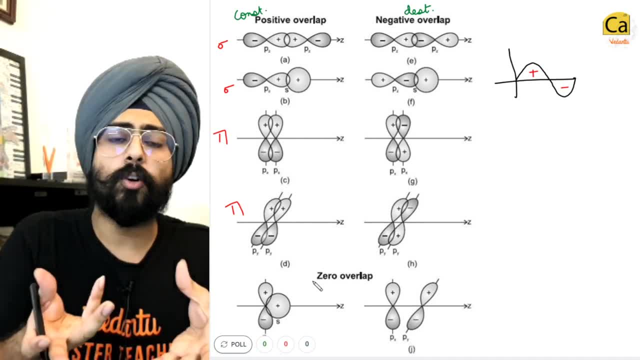 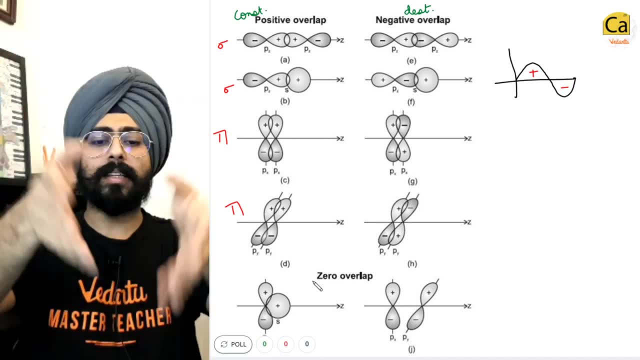 What does this mean? This means that the directions of the wave do not coincide with each other. OK, their phases do not meet at all. Positive, positive phase is far away. they are not meeting at all. So P orbital is in this position. S orbital is coming over here. 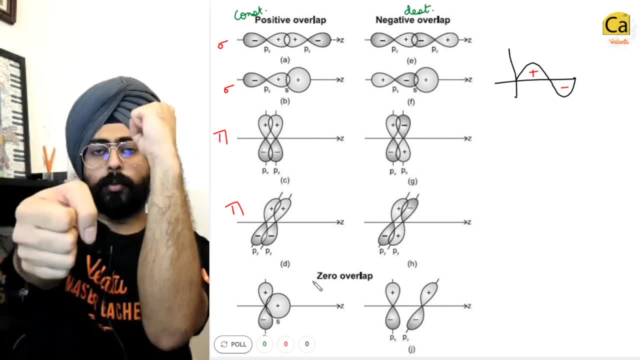 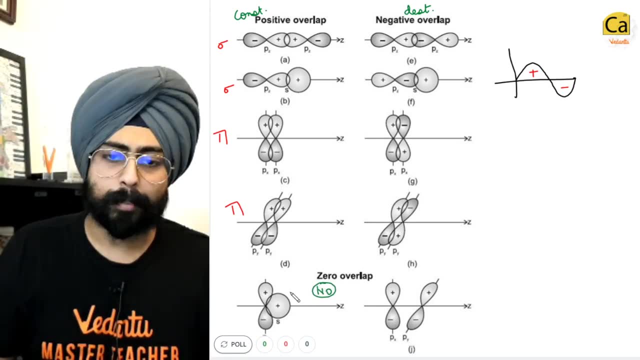 No overlap possible. One of the P orbitals is in this position. One of the P orbitals is in this position, No overlap possible. So the last case is zero overlap or essentially no overlap. Fine, This example is also given in the NCRT. 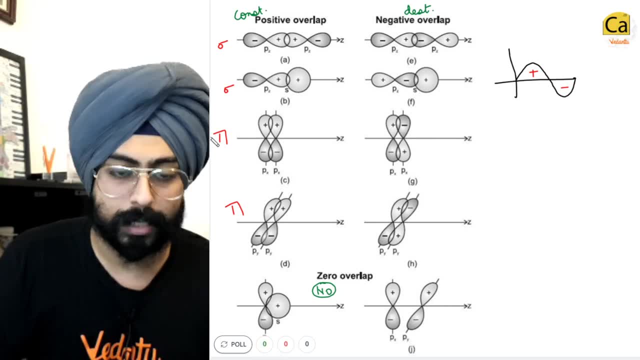 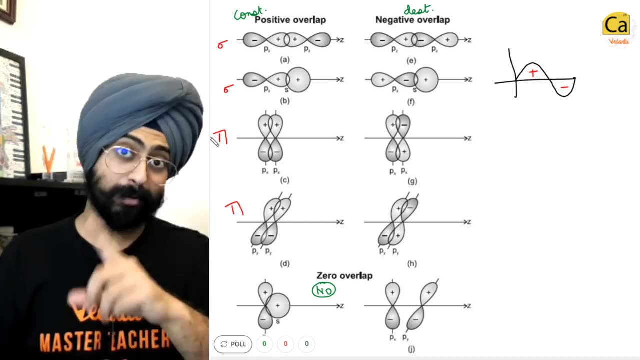 You can pause the video in case you want to focus on the diagram for a little more time. Then more improvement was suggested to valence bond theory by none other than Linus Pauling. Remember him from electronegativity? So what Linus Pauling said was that VBT tells us. 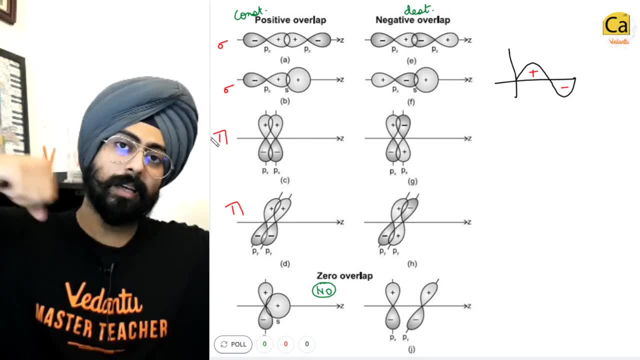 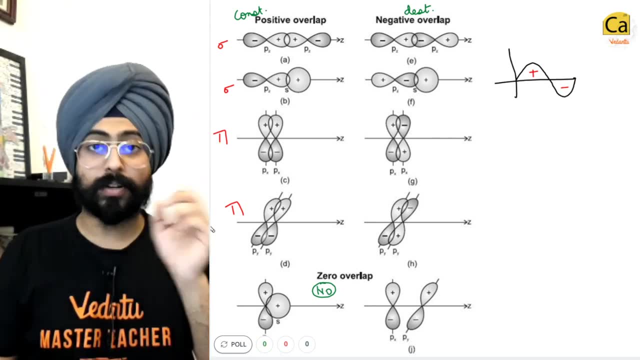 about the energetics, the kind of bonds that you form, the way they associate with each other and overlap. But what about the shapes? So Linus Pauling gave us the theory of hybridization, And hybridization theory is absolutely similar to VSEPR theory. 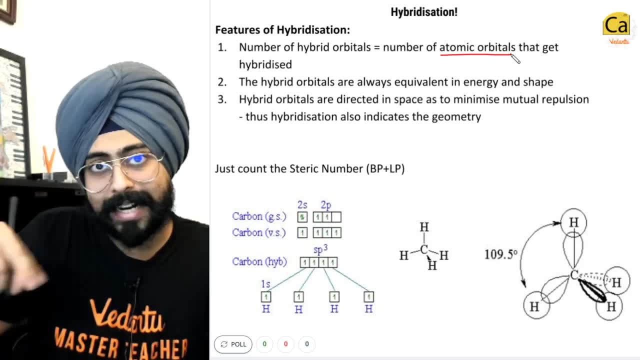 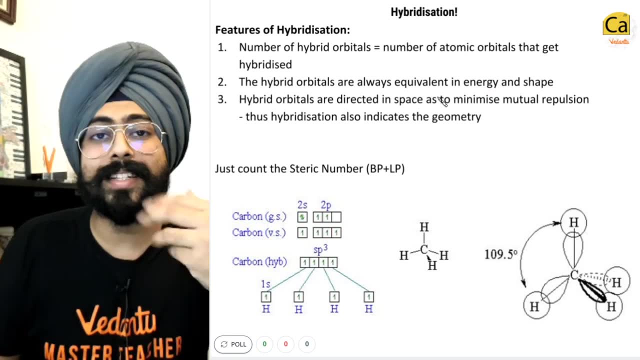 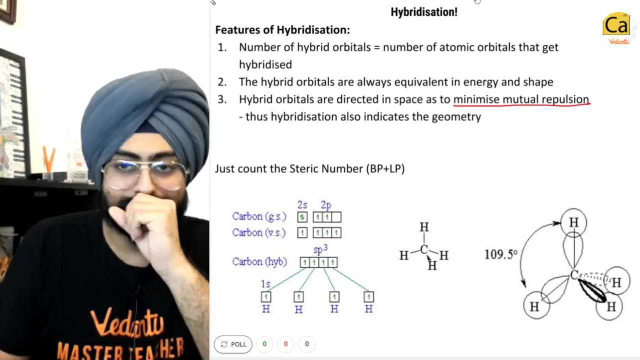 Hybridization says that number of atomic orbitals that get hybridized is equal to the number of hybrid orbitals. Hybrid orbitals are always equivalent in energy and shape, which means they are degenerate, And hybrid orbitals are erected in space to minimize mutual repulsion. 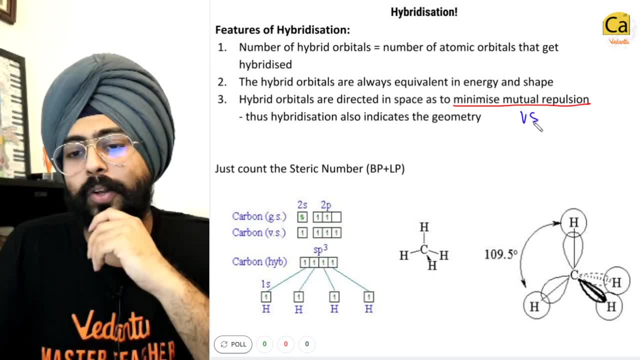 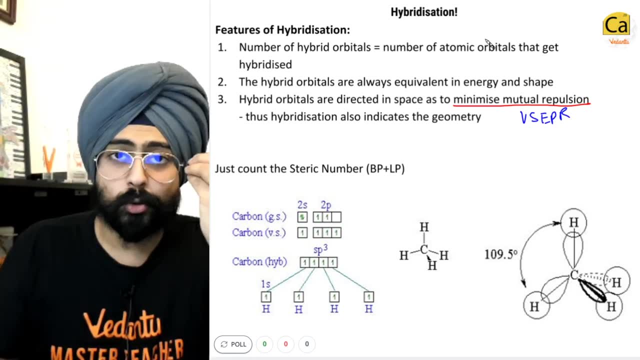 Doesn't this mutual repulsion minimization remind you of VSEPR? So if you know VSEPR, you know hybridization. It's as simple as that. You just have to count the steric number. To take a complete example, I have taken CH4 over here. 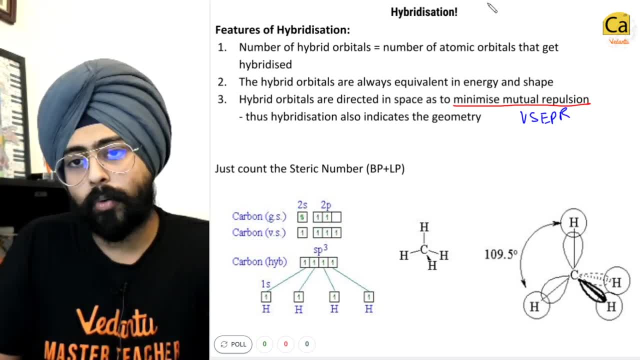 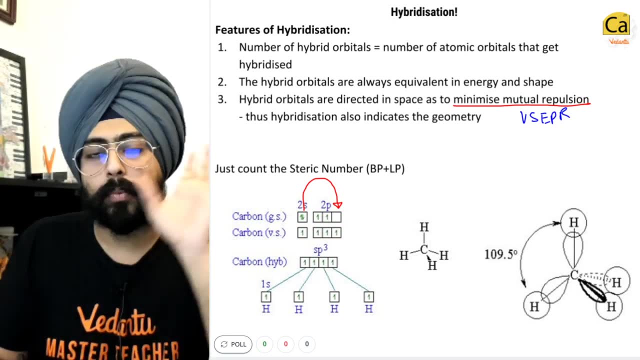 Carbon's ground state is 2s2- 2p2.. Now what we do is we take one of the electrons from the 2s and promote it into the 2p. Now you get four orbitals with 1111 electron each. 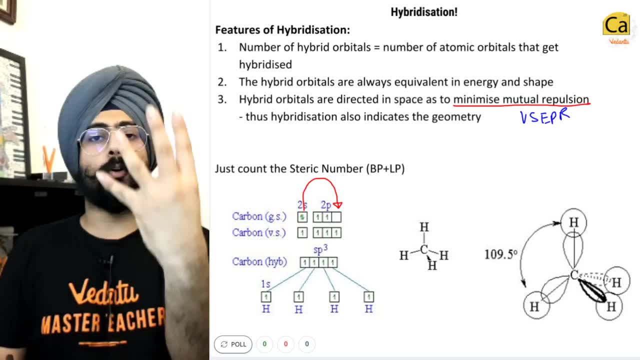 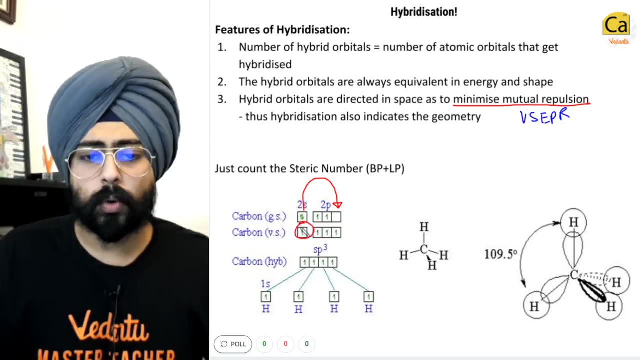 You combine these four orbitals together and you get four hybrid orbitals. What will those hybrid orbitals? be called sp3.. Why sp3?? Because one s orbital is getting involved and three p orbitals are getting involved. So, very simply, sp3. 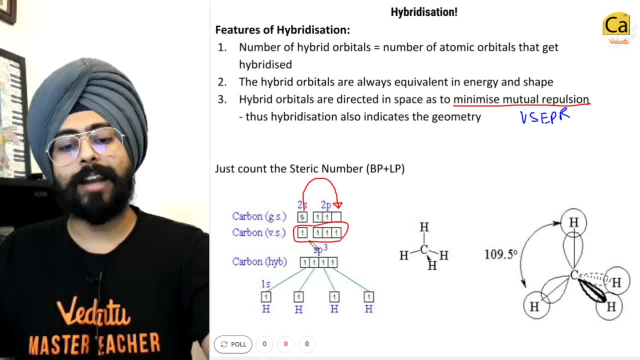 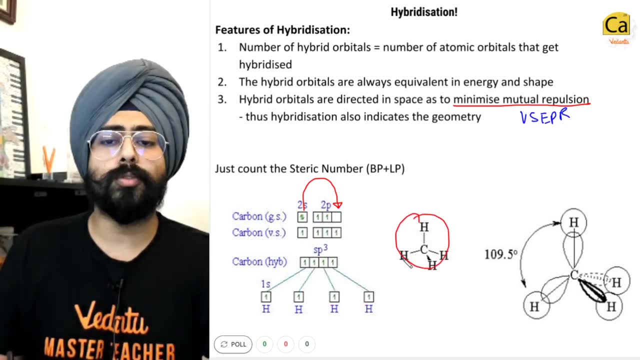 How many sp3? Four, Because we started with four atomic orbitals. Now, each of these sp3 orbitals can bind with one hydrogen and give you CH4.. Now what's the shape of these hybrid orbitals? Every hybrid orbital ever will have this shape. 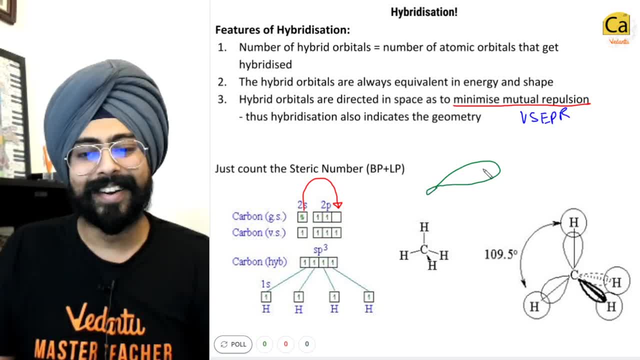 Remember this fan type of a shape, fin of a fan. Yeah, one of the lobes is positive, one of the lobes is negative. The signs tell us that these two have different signs in the wave function. OK, fine, Now if I have to align them. 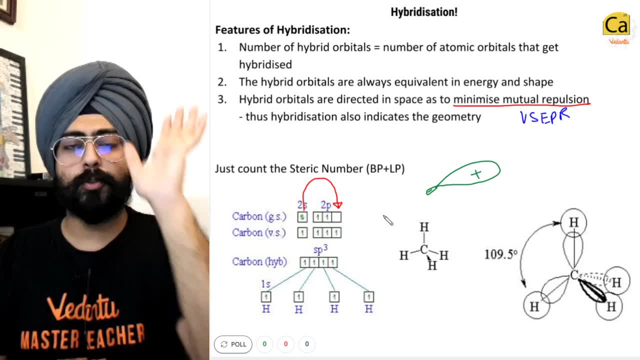 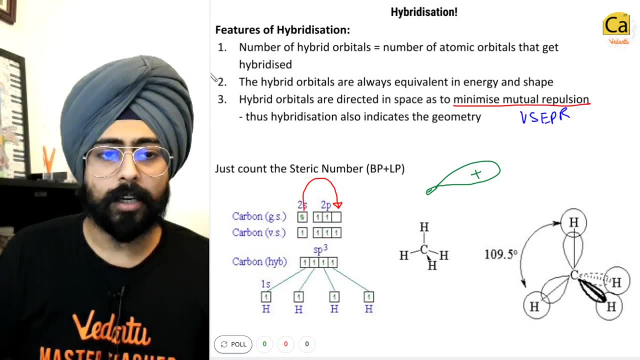 I am pretty sure you realize that the positive directions will align themselves to minimize repulsion, Hence the tetrahedral structure. Do you realize this is the same as VSEPR, In fact. let me quickly take you through the VSEPR things once again. 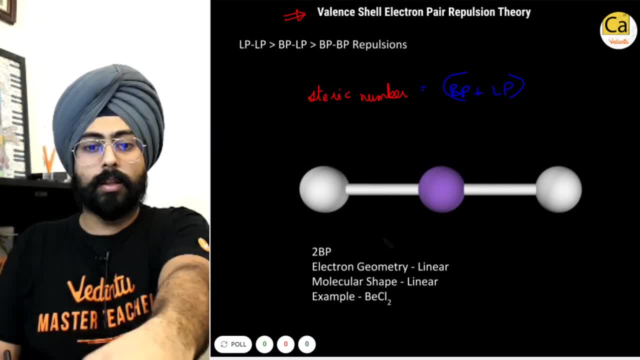 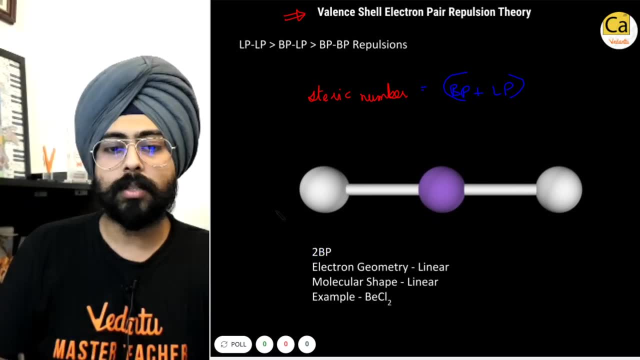 And let's write the hybridizations of all of these cases: Steric number equal to two. What is the hybridization over here? sp? Why sp? Because there are two hybrid orbitals: One comes from s, one comes from p. 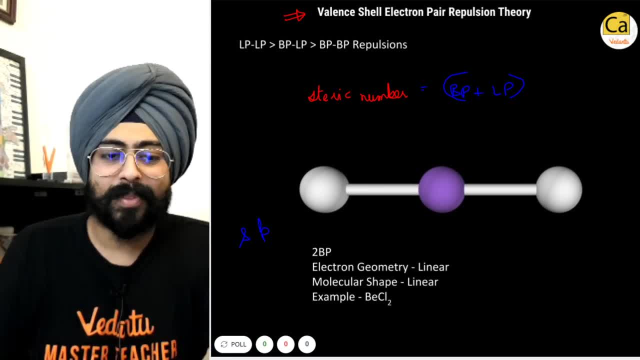 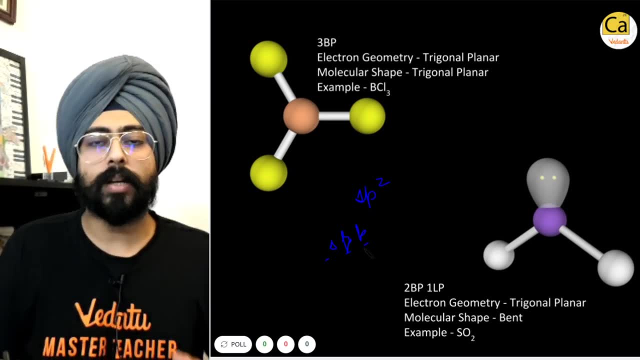 So two sp hybrid orbitals, as simple as that. Steric number three: What is the hybridization? Sp2.. Why? Because s, p and p. How many orbitals? One, two and three Done. Then steric number four: 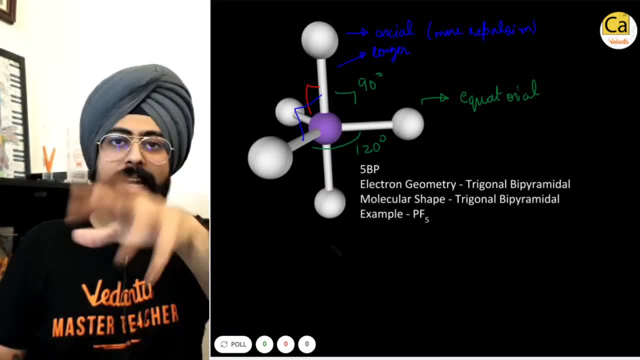 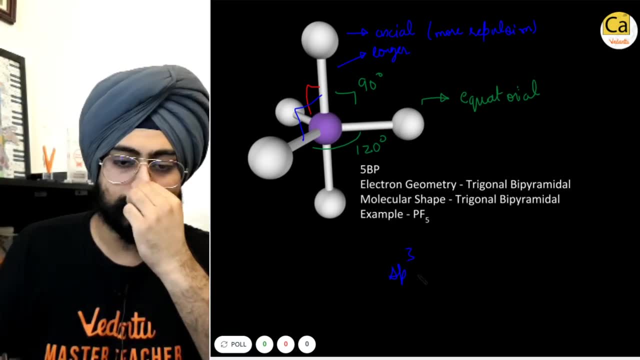 What will be the hybridization Sp3.? Steric number five. What will be the hybridization Sp4?? No sp3, because you can't have more than three p orbitals. Sp3d: There are some cases of dsp3 as well. 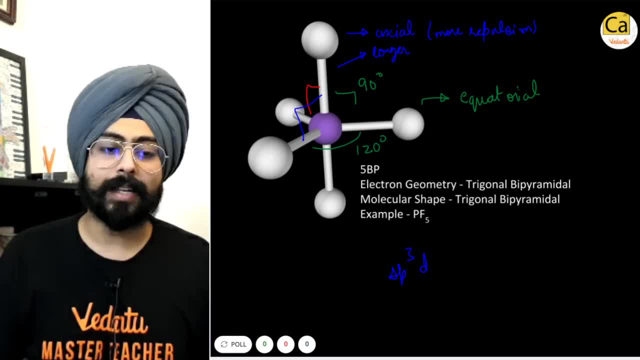 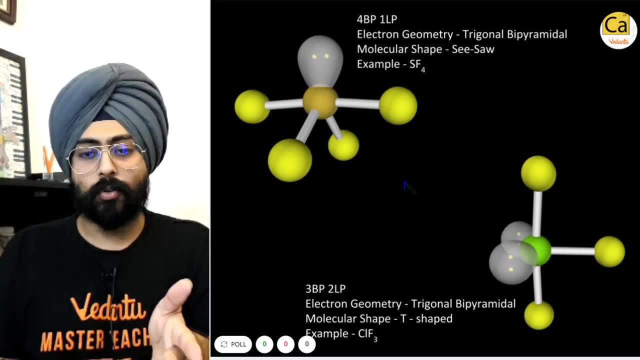 You can look at coordination complexes chapter to understand that idea better. We'll do some revision of that in the question solving session tomorrow. Once again over here: all of these are sp3d. We'll go ahead. Sp3d is still going on. 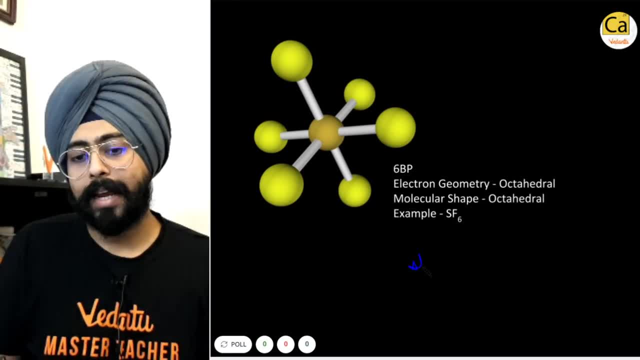 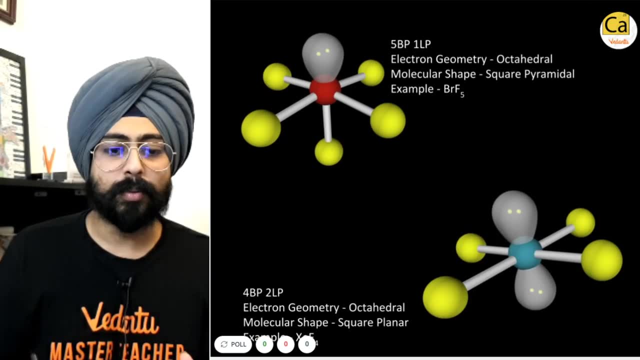 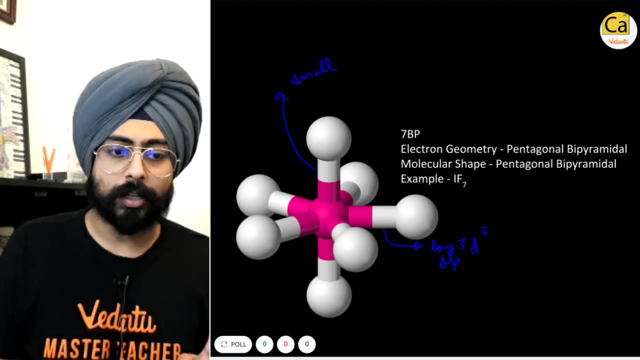 Five steric number. Then comes six steric number, sp3d2.. Why s, p, p, p, d and d, Six orbitals. Similarly for steric number seven, sp3d3.. So in case you know the VSEPR theory, in case you are able to calculate the steric, 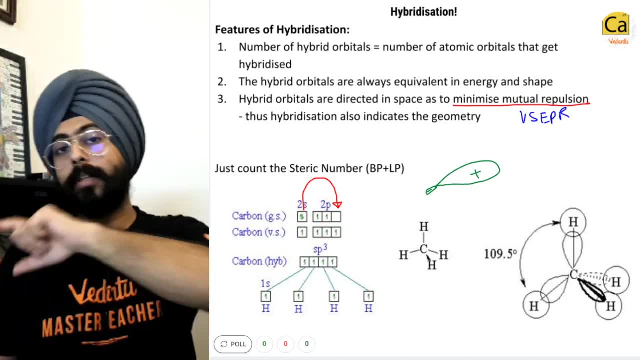 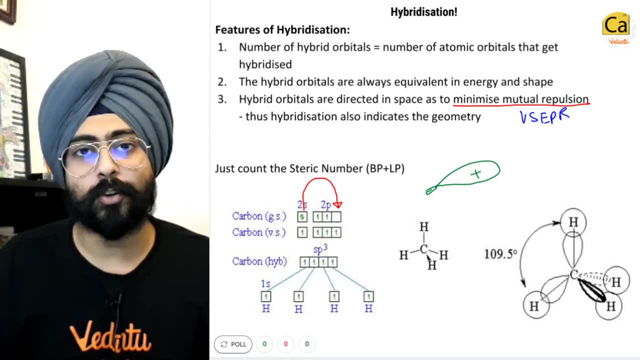 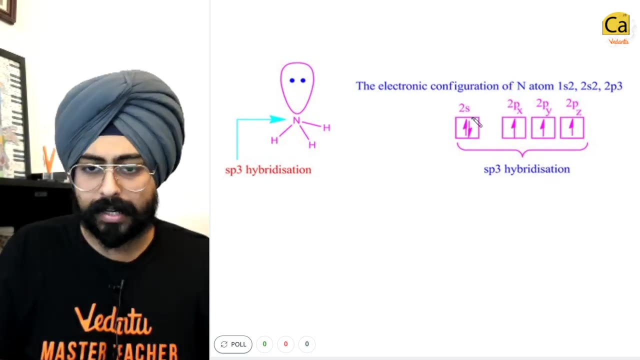 number. you can do hybridization Now. there are multiple tricks to calculating the steric number, and the details of that will be discussed in tomorrow's question solving session. Fine, Awesome, We'll go ahead For hybridization. you definitely do not need to. excite the electrons, not always. In some cases it is necessary, like it was in CH4.. Over here NS3's example is taken. This is the lone pair. The rest of them will bond with hydrogen Hybridization. over here will still be sp3. 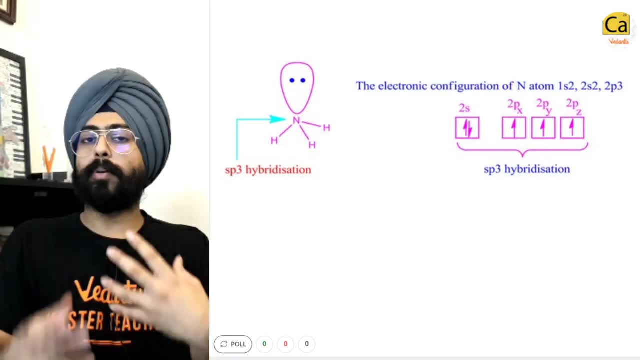 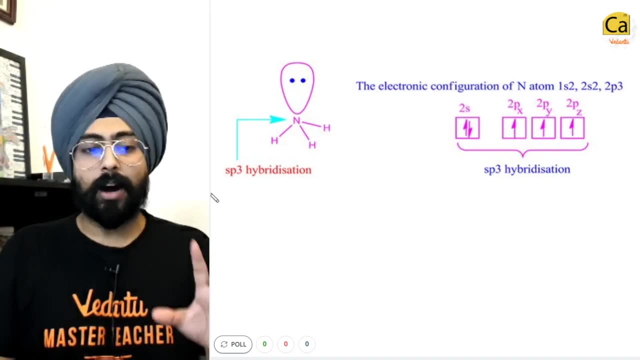 Very nice. So for more details and more examples on this, please make sure you join the discussion, the question solving session. that is tomorrow at 8 pm. Anyway, now let's come to the final and the most important and the most relevant. 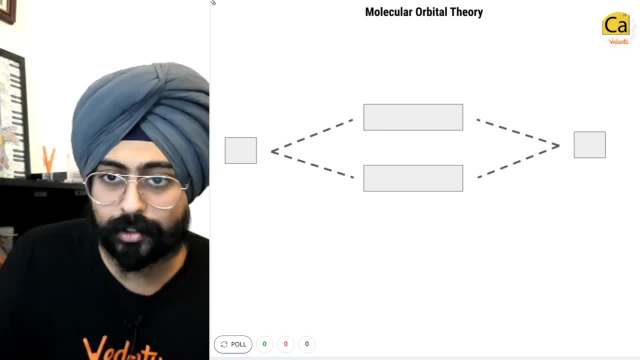 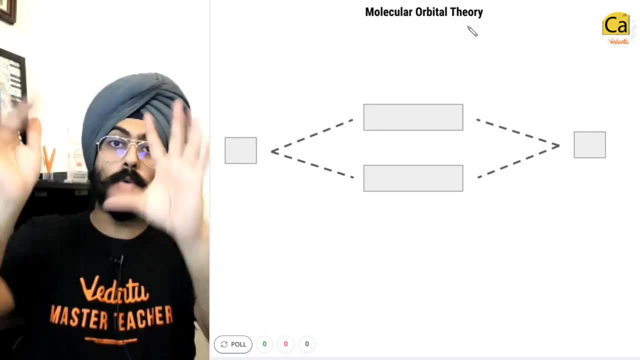 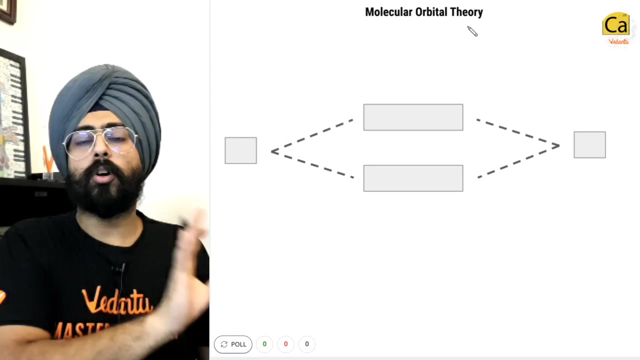 theory of all, and that is molecular orbital theory. What happens in molecular orbital theory? You consider molecules as different entities. Atoms plus atoms gives you something new altogether, and that is a molecule. Molecule will have its own orbitals. Molecule does not have atomic orbitals anymore. 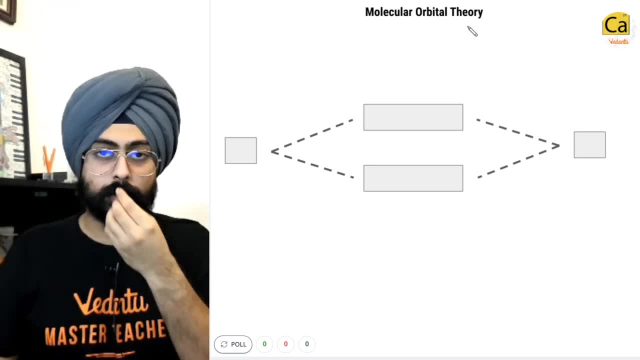 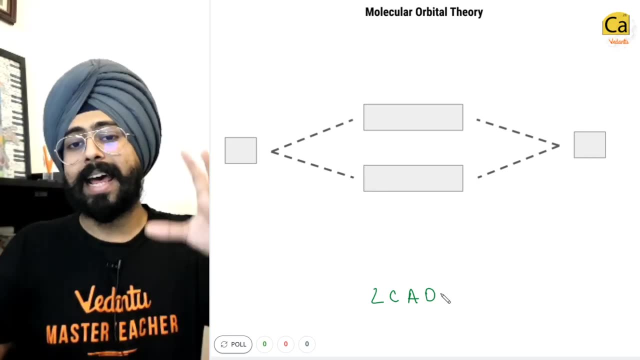 It has its own molecular orbitals. So what we will do is we will do linear combination of atomic orbitals- LCAO means linear combination of atomic orbitals- and then we will create molecular orbitals. Fine, So you can have a 1s combining with a 1s. 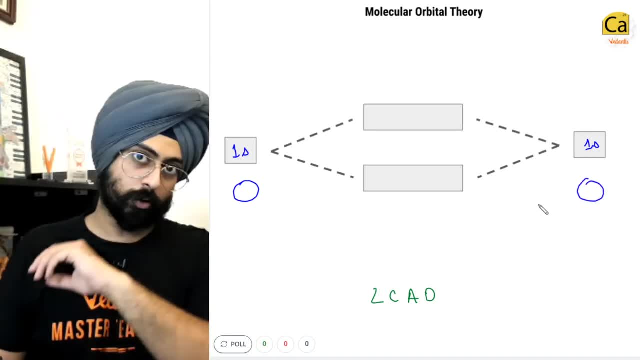 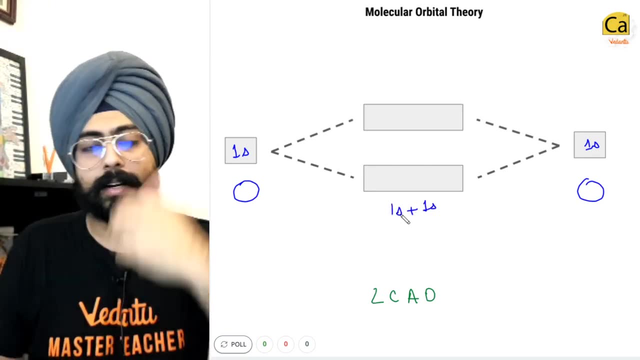 Yeah, A spherically symmetric orbital combining with a spherically symmetric orbital. What can happen is there would be two cases. One would be a constructive interference case. Let me write it as 1s plus 1s. There would be a destructive interference case: 1s minus 1s. 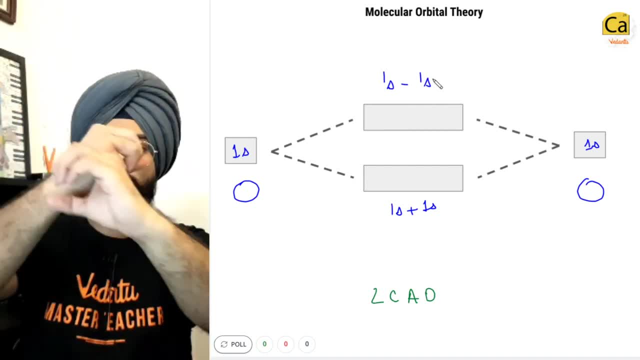 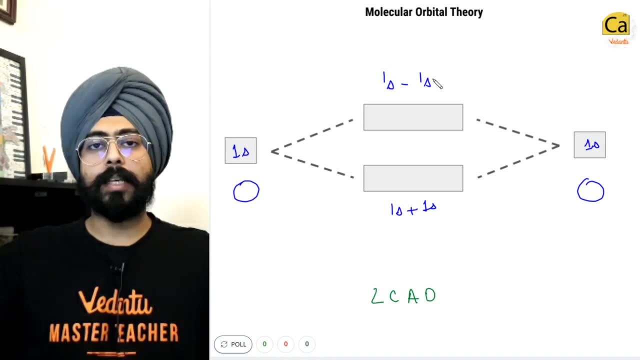 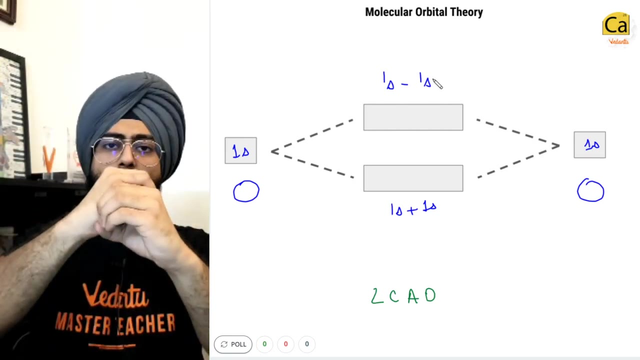 Now in destructive interference. does this mean that they both will just eat each other out and give you no orbital at all? No, Why. They will only interfere with each other partially. Why so? Because assume these are the two atoms coming together. will they sit on top of each other in the bond? 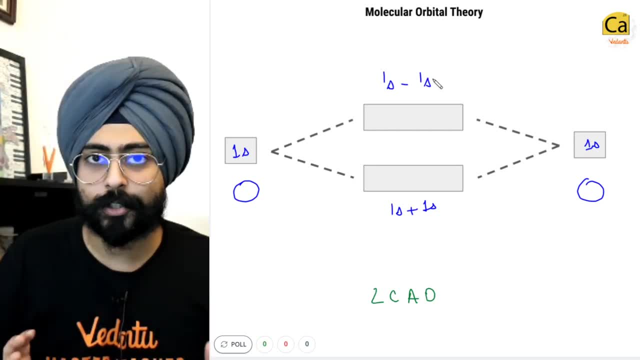 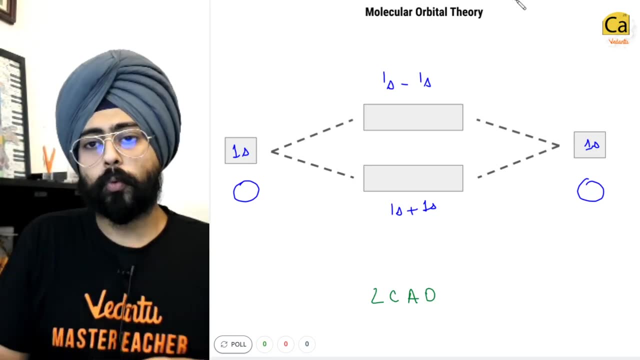 They will sit at a certain distance, like 74 picometers in hydrogen. So over here the overlap is just partial. This much overlap, OK, fine. So when these two combine together in a positive overlap they will give you a bigger orbital. 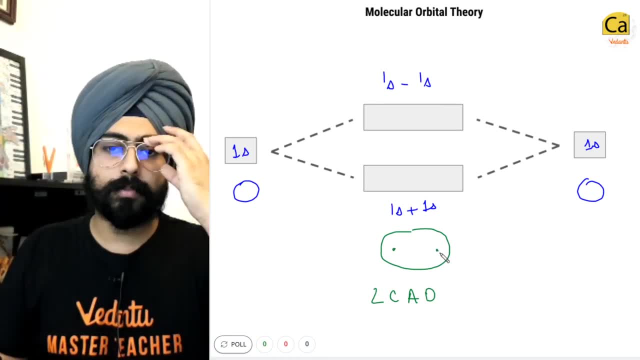 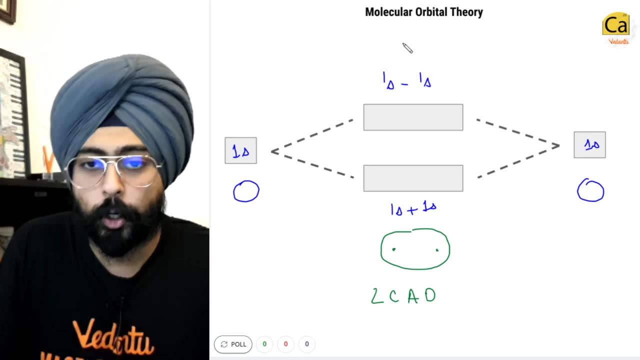 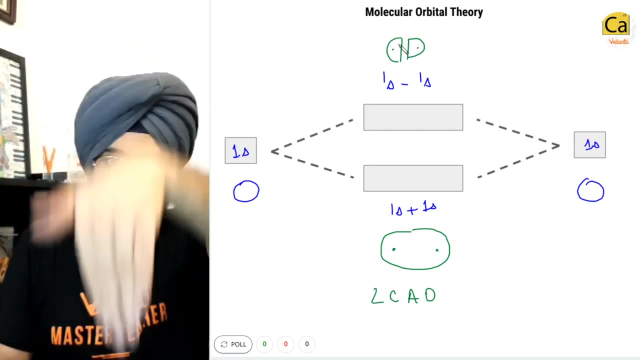 Yeah, This and this are the nuclei of the original atoms, And in a negative overlap they will eat out some portion of each other. So what will that look like? That will look something like this: Yeah, Do you see? there is a node in the middle now? 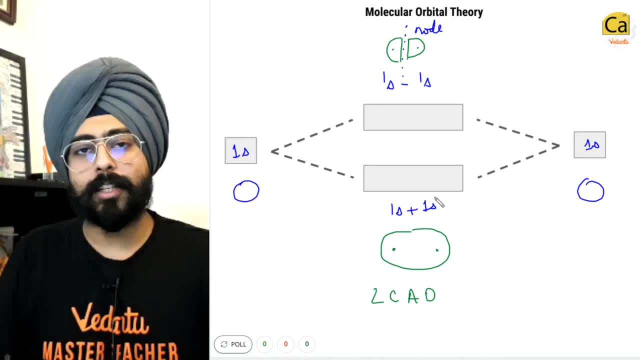 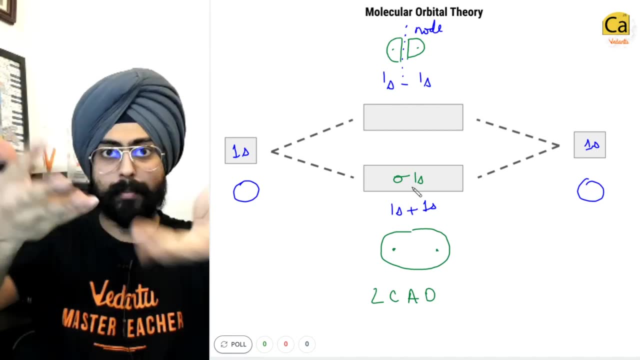 So they've eaten out each other to a little bit. How do we name these orbitals? We can call the bottom one sigma 1s. Why sigma? Because it's a head on overlap, like in VBT, And the top orbital can be called sigma star 1s. 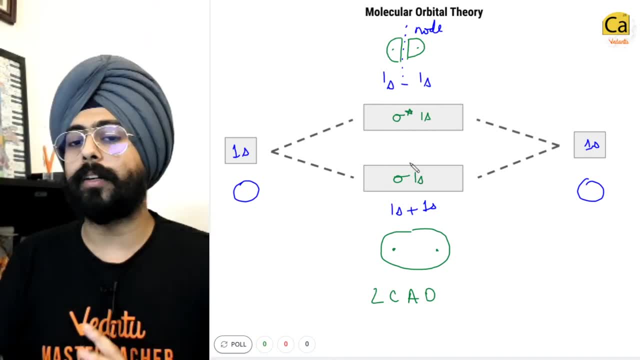 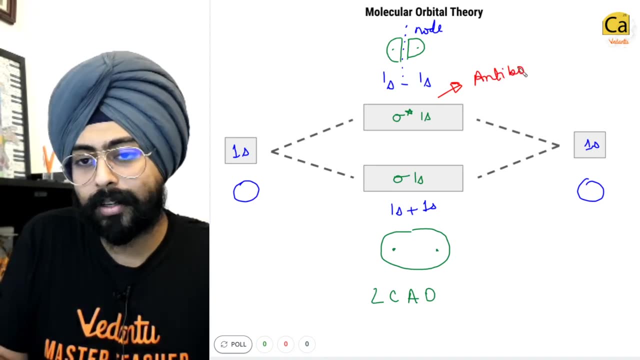 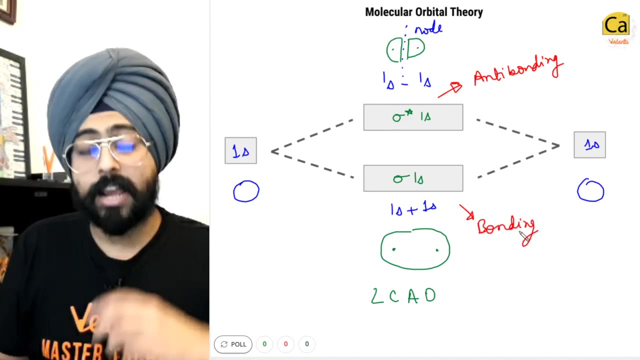 The one on the bottom has lower energy. The one on the top has higher energy. Higher energy means unstable. We call it the antibonding molecular orbital And the one at the bottom is known as the bonding molecular orbital. If electrons in a molecule go to bonding orbitals, that makes it stable. 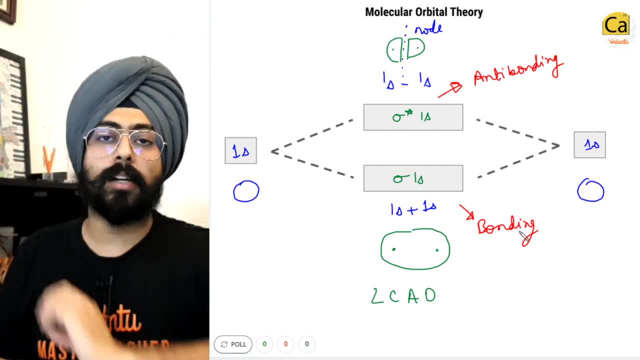 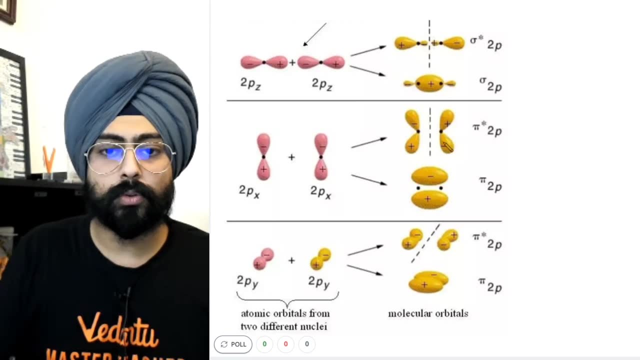 If electrons go to antibonding molecular orbitals, that makes the final molecule unstable. Fine, Now, quickly, let us look at the other types of orbitals that we need to figure out. If we have p orbitals overlapping, you could have sigma overlap, 2pz combining: 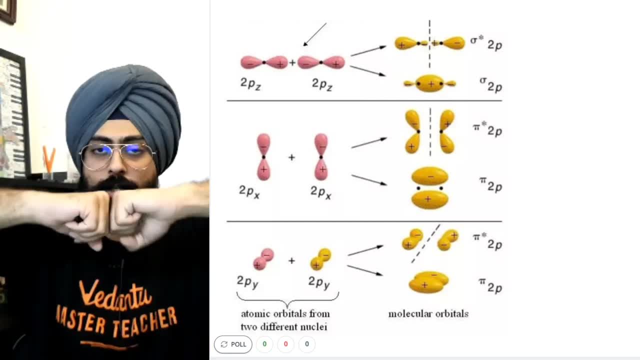 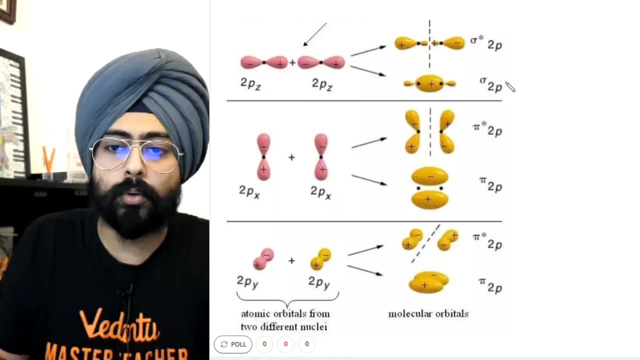 with 2pz, considering that z axis is the principal axis of overlap. So sigma overlap will happen over here. So you will get sigma 2p and sigma star 2p. You can call it sigma 2pz and sigma star 2pz, Fine, 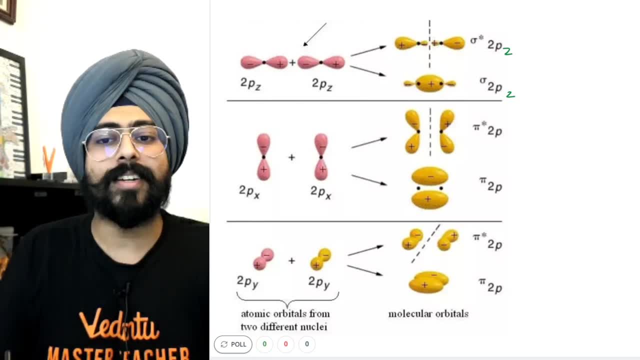 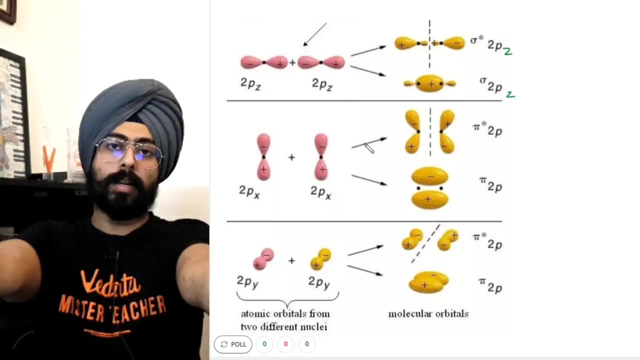 So you can see how this has a positive overlap and this has a negative overlap. So antibonding is always denoted with a star. Now you could have pi overlap as well. Two types of pi overlap are given over here: One in this direction, one in this direction. 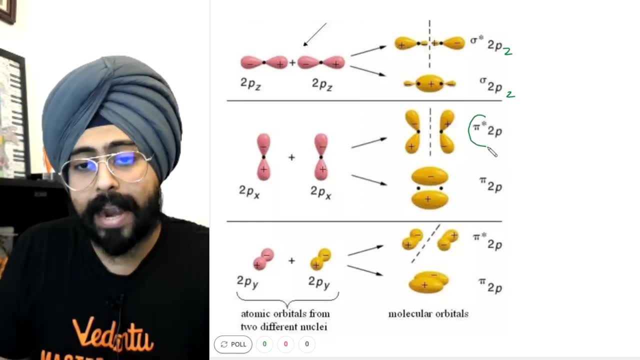 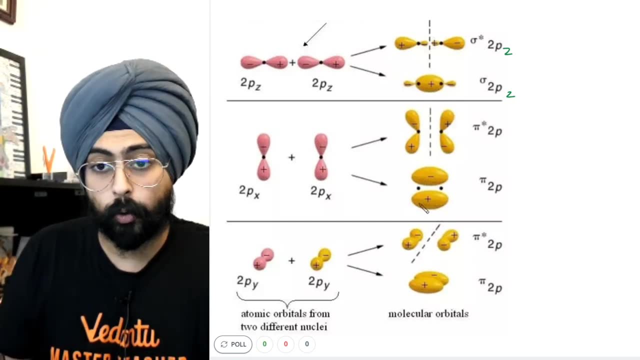 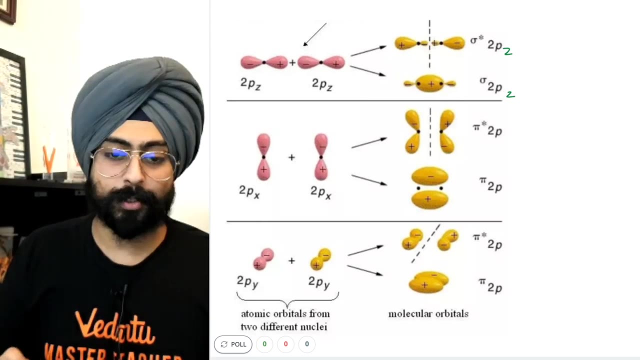 And the orbital shapes are also given to you: Pi 2p and pi star 2p. pi 2p and pi star 2p: In the star you create a node, an extra node, But in the bonding molecular orbital you create bigger, more expanded lobes. 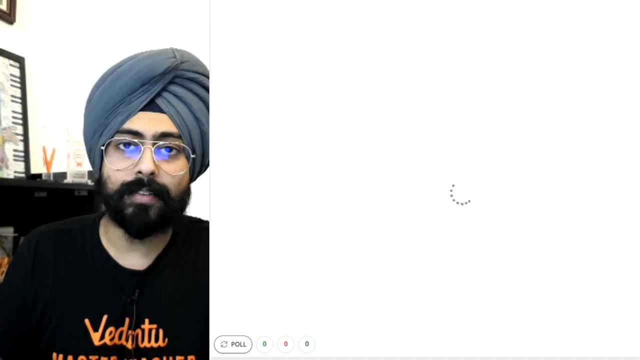 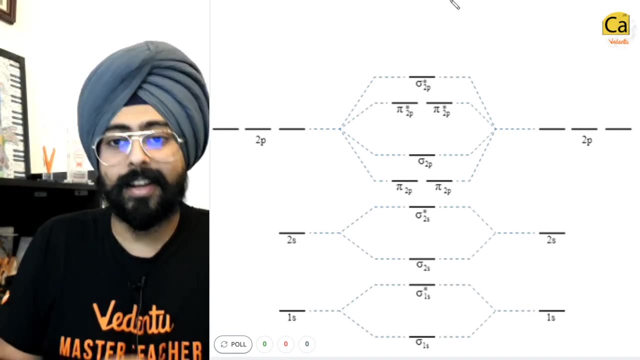 Fine, In case you want to pause on this page, you can pause. Otherwise I will move forward to energy diagrams. Now, the last thing that we will discuss in this class: another five minutes energy diagrams. this particular energy diagram on your screen is applicable. 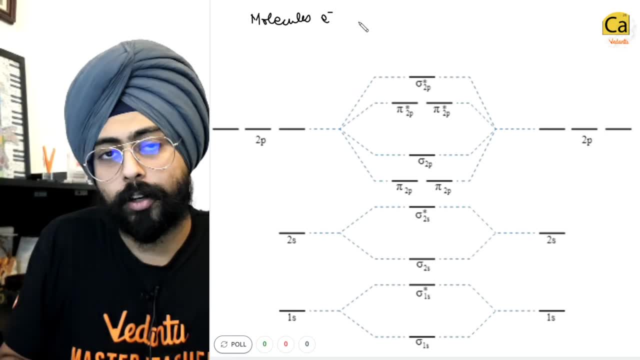 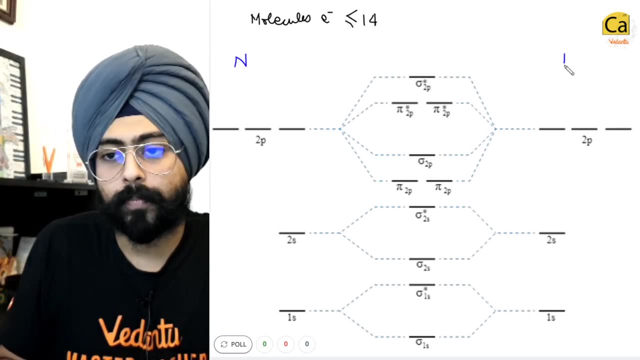 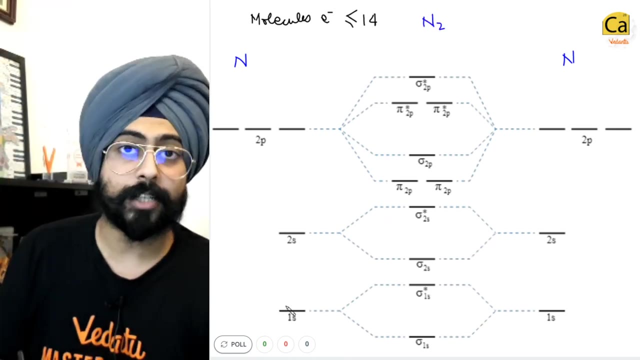 for molecules with electrons less than equal to 14.. OK, let's take the example of nitrogen: Two nitrogen atoms combining together to form N2.. So seven. seven atoms in each of the nitrogens. Let's write the electronic configurations. 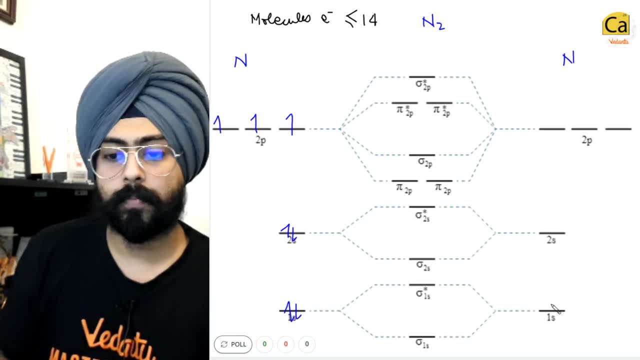 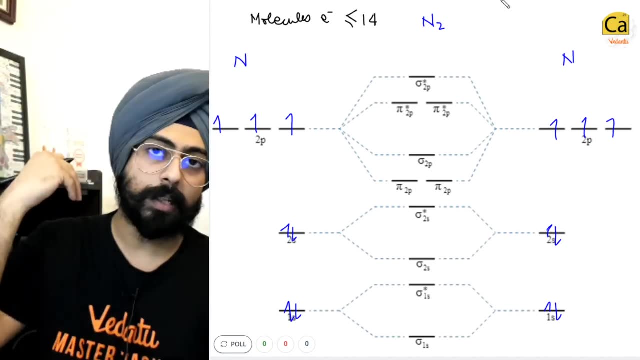 1s2, 2s2, 2p3, 1s2, 2s2, 2p3.. So finally, in the molecular orbitals you have to fill the electrons and give the molecular orbital electronic configuration. 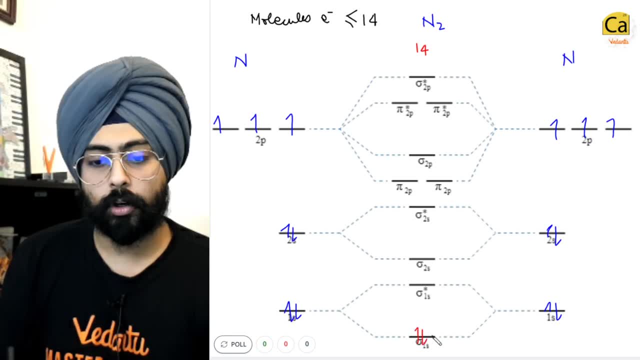 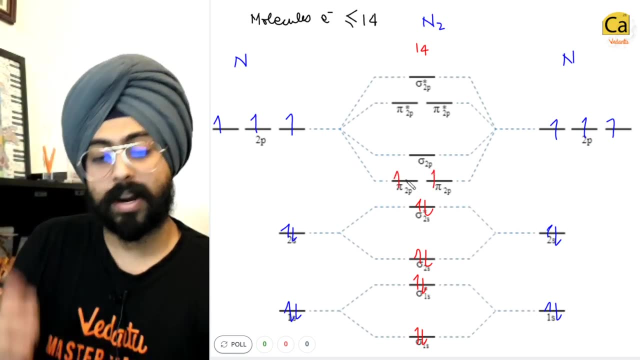 So over here, total electrons are 14.. Let's fill them 1, 2,, 3,, 4,, 5,, 6, 7, 8.. Notice 9. 10. Why did I fill 1, 1 each? 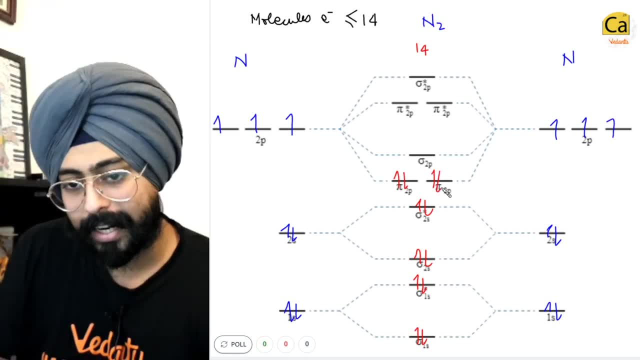 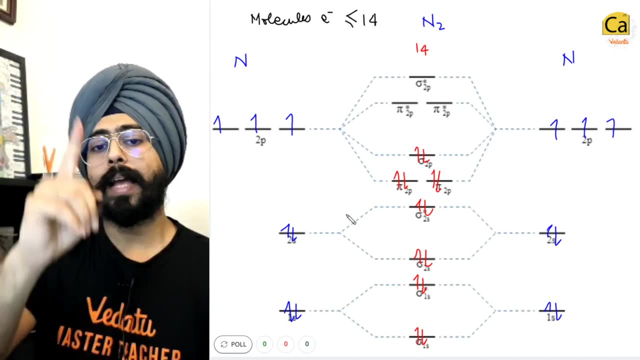 Because Hund's rule of maximum multiplicity: Yes, 9,, 10,, 11,, 12,, 13 and 14.. This is how you're supposed to fill electrons in the molecular orbitals, Also in electrons less than 14,. 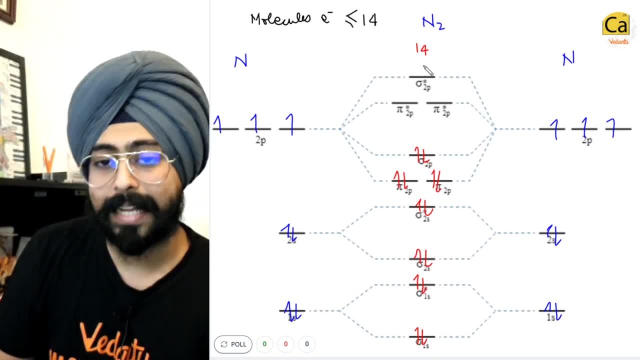 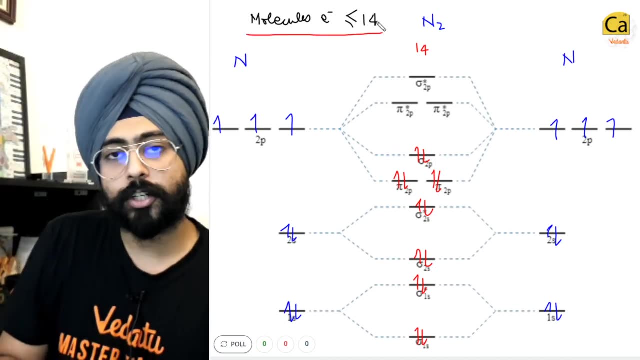 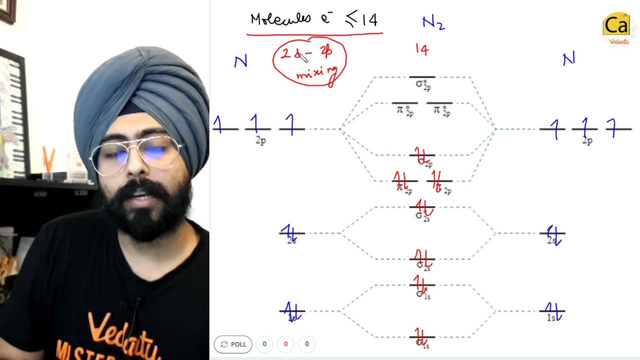 for molecules and electrons having electrons less than 14.. This order is very important. This is the energy diagram that you will follow And we say that in such small molecules you have 2s- 2p mixing. OK, What happens in this 2s- 2p mixing happens. 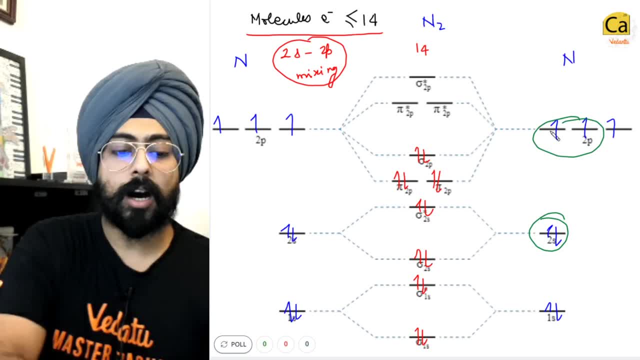 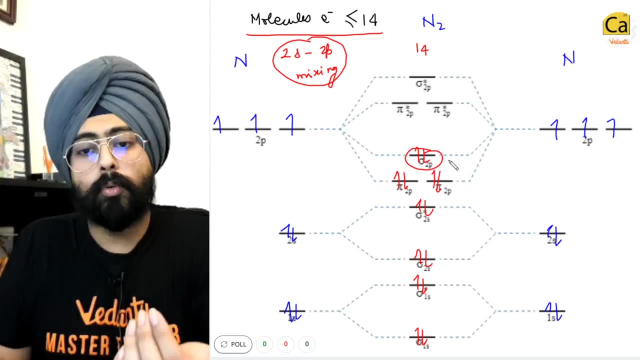 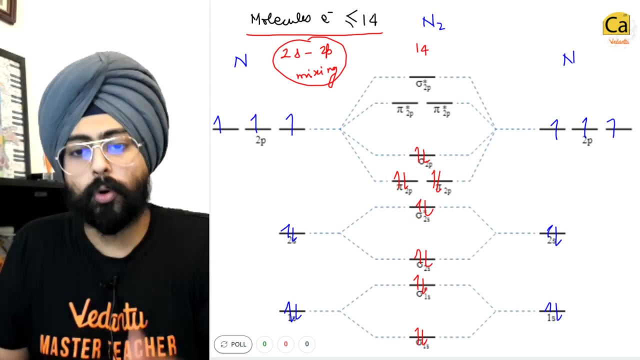 What it means is that, because 2s and 2p are very close to each other in energy, when they mix together they make the 2pz more unstable, They cause it to go a little towards the top and they cause the sigma star 2s to go a little towards the bottom. 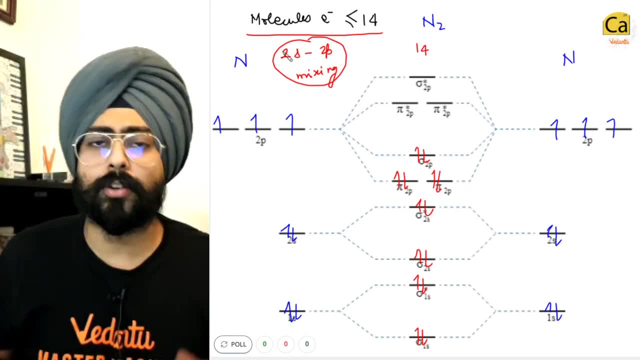 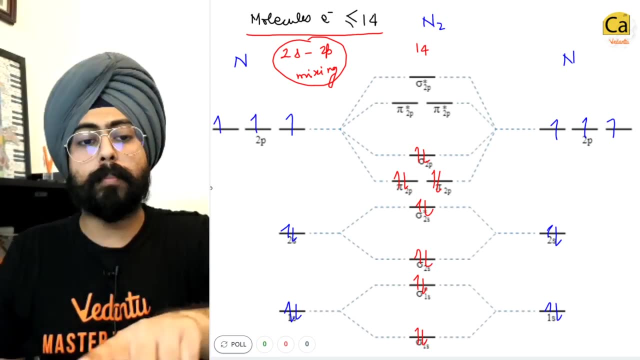 Now you can research more on 2s 2p mixing. No one's going to ask you questions on this in our syllabus, but you should know That this case is of 2s 2p mixing. What does the 2s 2p mixing absent case look like? 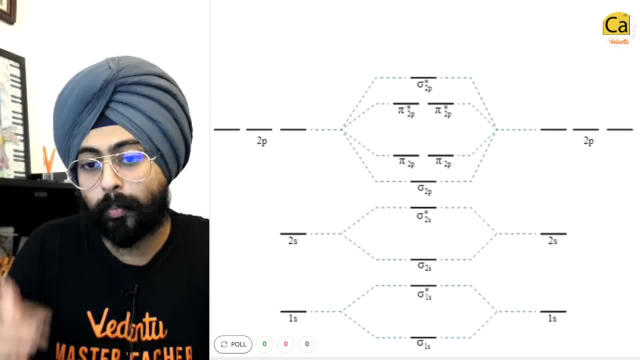 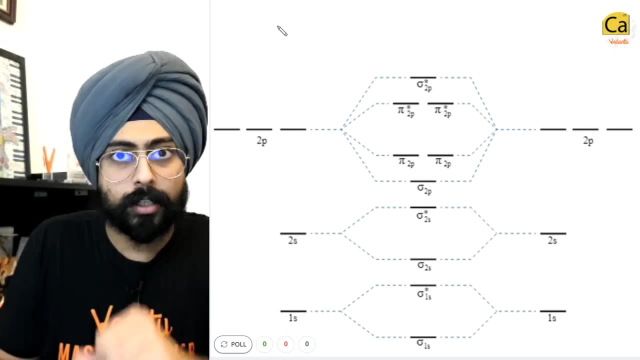 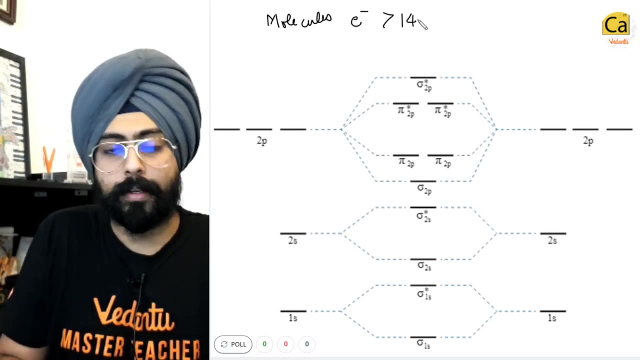 This is what it looks like. Do you notice the difference? over here, The sigma 2p is lower than the pi 2ps. Over here, sigma 2p is higher than pi 2ps. Yes, So this particular diagram is applicable for molecules with electrons more than 14.. 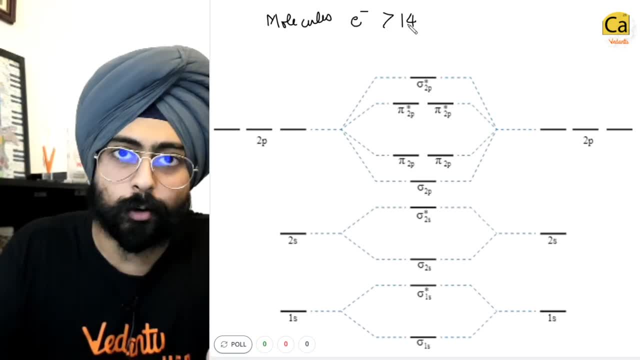 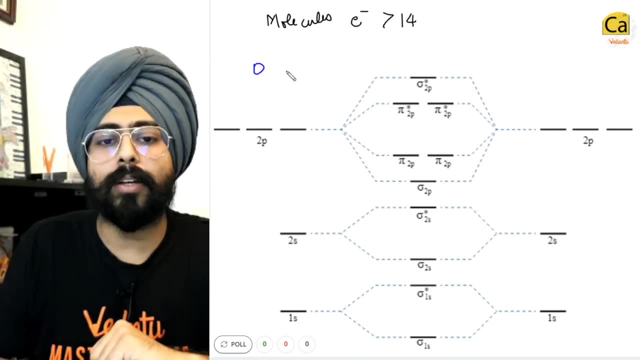 Now in our syllabus we do not talk about molecules having more than 20 electrons And we talk only about diatomic molecules. So that is just a limitation of our syllabus. As an example over here we'll take oxygen. 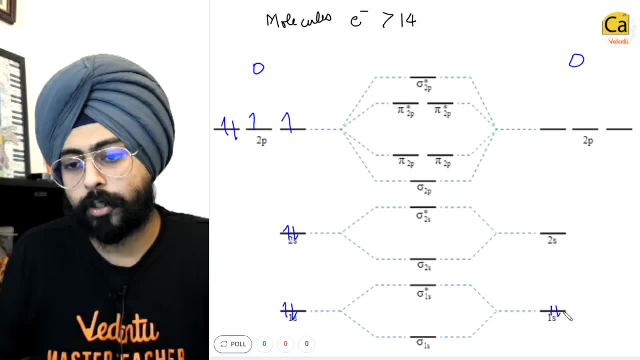 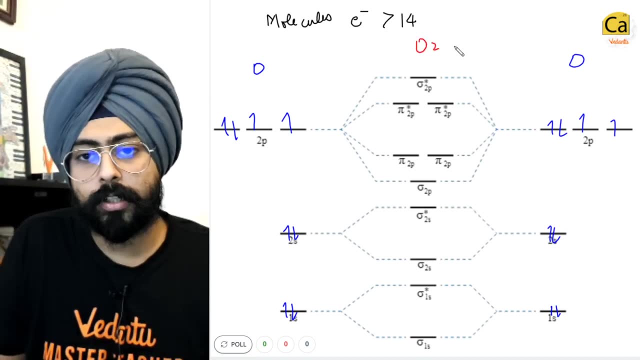 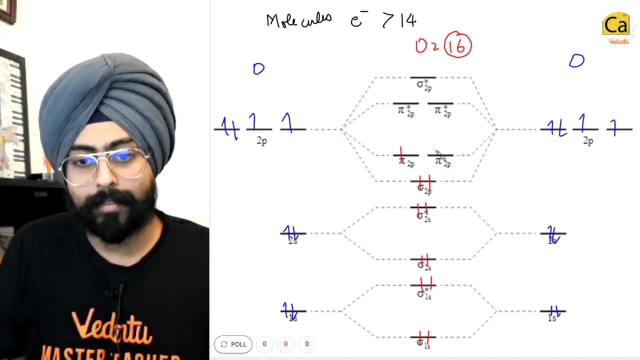 1s2,, 2s2,, 2p, 4.. Let's fill these on the right hand side as well. Let's fill them in the middle. How many electrons do I have to fill? total 16.. So 1,, 2,, 3,, 4,, 5,, 6,, 7,, 8,, 9,, 10,, 11,, 12,, 13,, 14.. 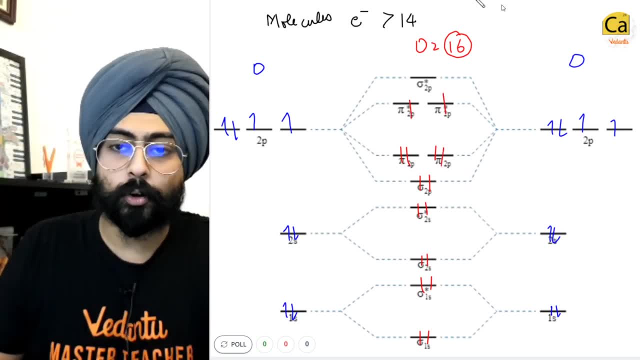 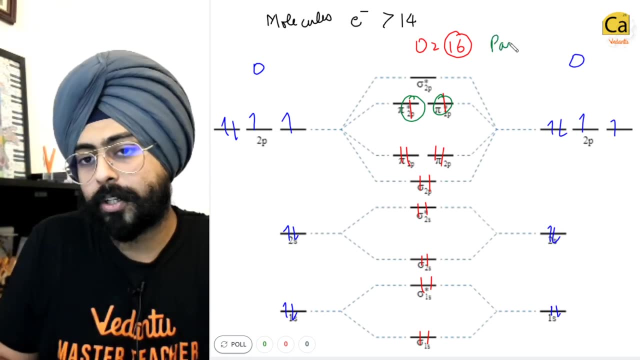 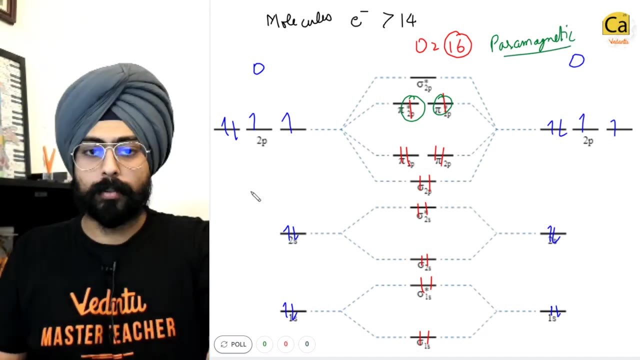 15 and 16.. One thing that you should notice over here are these two unpaired electrons. What does this mean? Unpaired electrons mean that oxygen is paramagnetic. Yes, oxygen is paramagnetic. Fine, Now people, quickly to summarize just the molecular orbital theory. 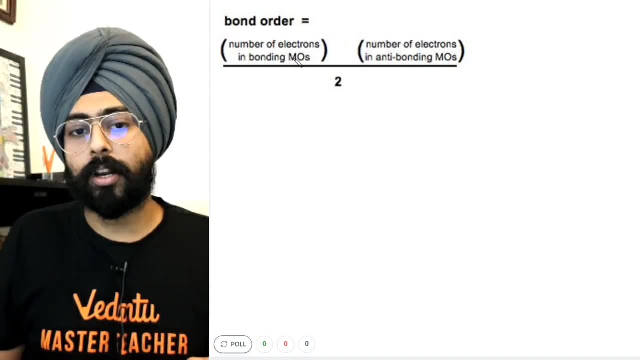 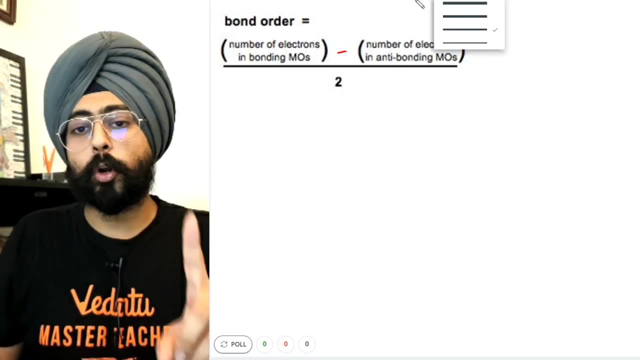 Over here I'll tell you the formula of bond order, That is, number of electrons in bonding molecular orbitals minus number of electrons in anti-bonding molecular orbitals. And now I will give you a trick. This trick is going to make your questions way faster. 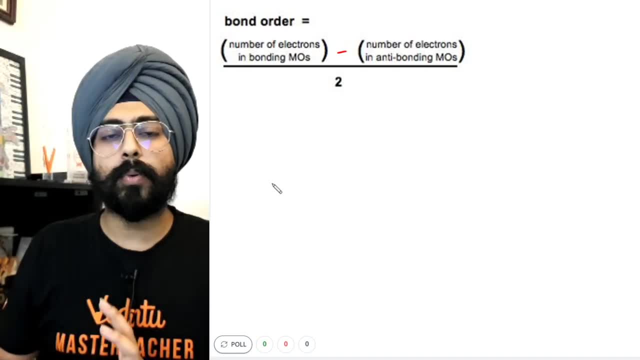 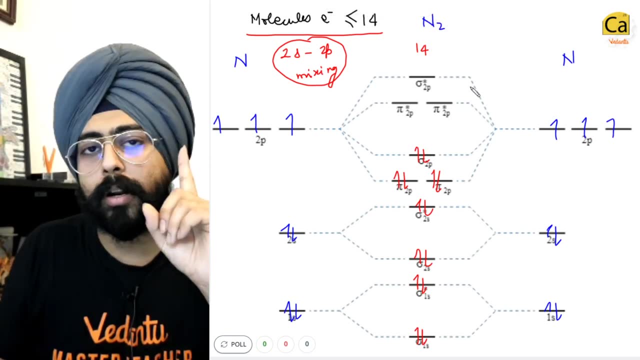 Ready for the trick. In order to draw molecular orbitals, let us say we have to draw the case of 2s2p mixing. This was the case In 2s2p mixing. you have to remember a number For 2s2p mixing. the number that you have to remember is 2, 1, 2, 1.. 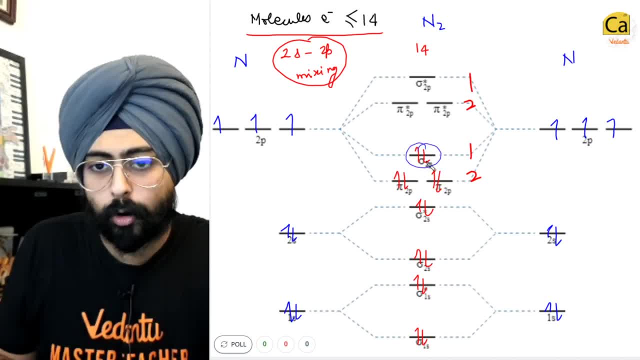 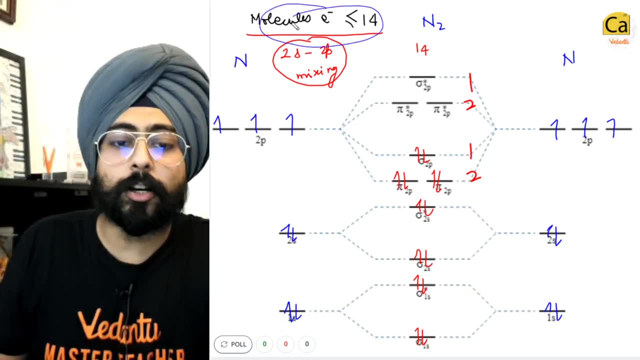 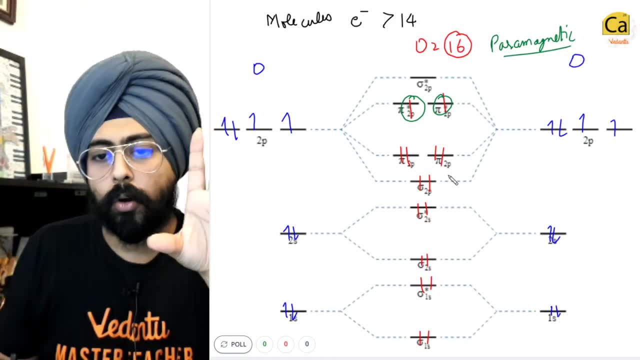 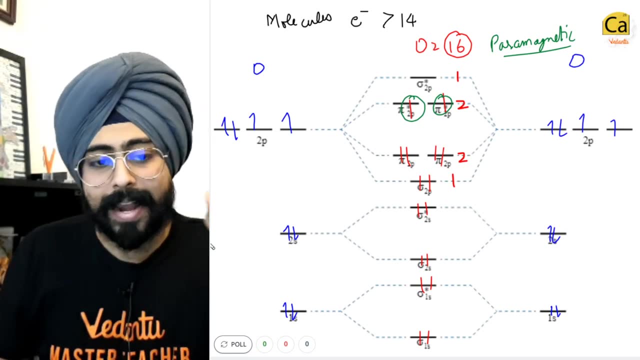 For more than 14,. what you have to remember is 1,, 2,, 2,, 1.. OK, what you have to remember is 1,, 2,, 2,, 1.. Fine, Now coming towards the final page, over here. 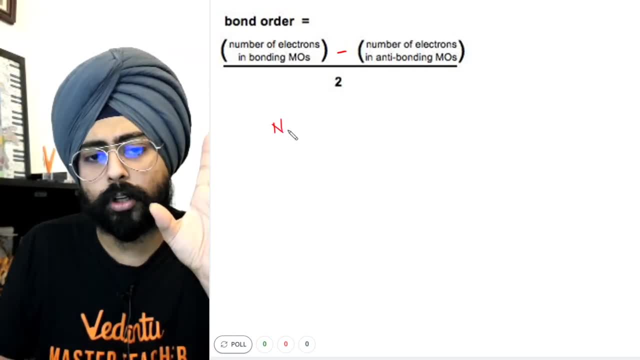 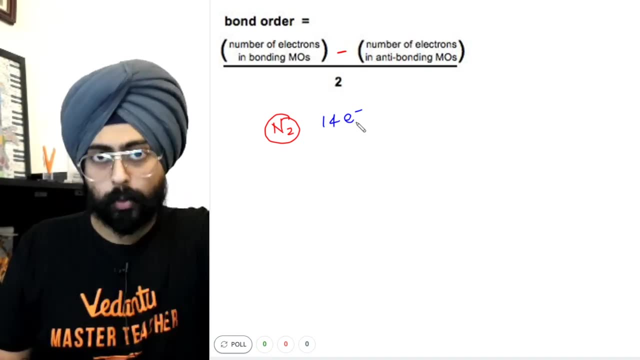 The trick that I want to tell you is: imagine you are making the molecular orbital diagram of N2.. N2 has 14 electrons, So over here you have to make 2s2p mixing present. Yes, 2s2p mixing will be present over here. 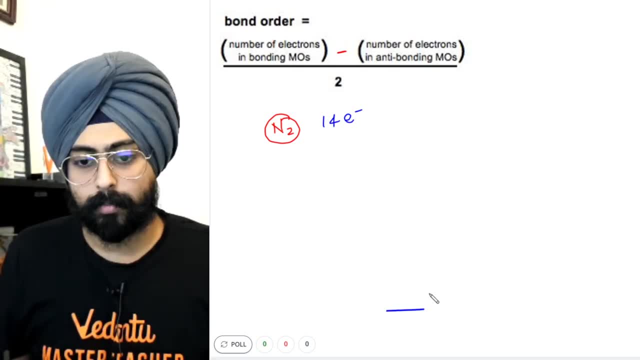 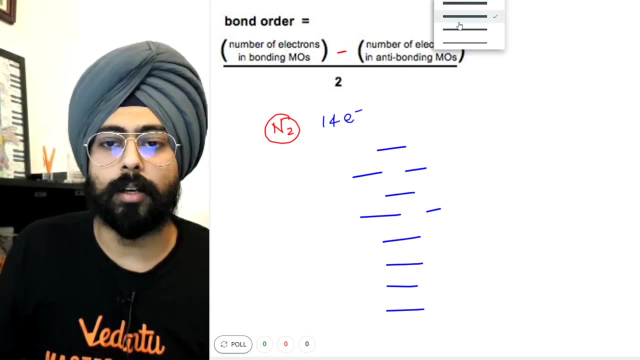 Watch carefully. This is how you draw it in the examination: Sigma 1s, sigma star 1s. sigma 2s, sigma star 2s, 2, 1, 2, 1.. Molecular orbital diagram is done.